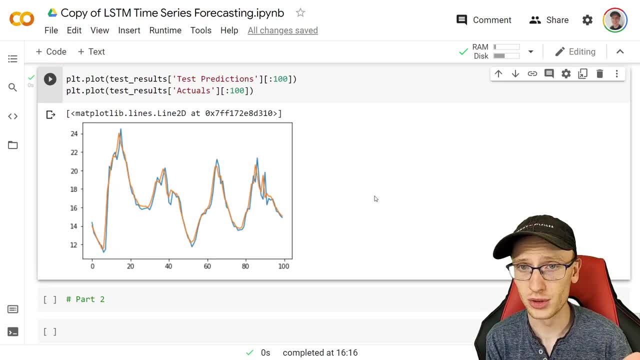 that you definitely might want to do is use more variables to help predict, because, you know, often in neural networks or whatever type of model, we don't generally just look at one type of variable. Technically, we're looking at five data points or five different values to use our prediction. 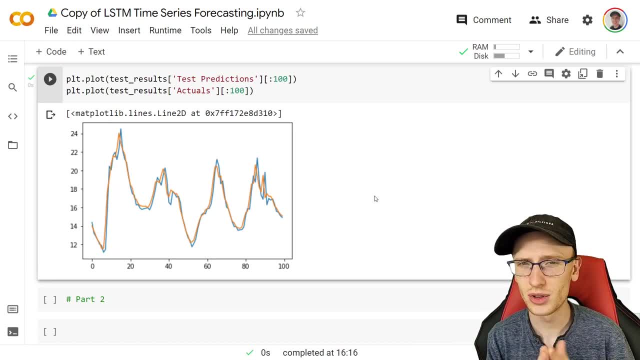 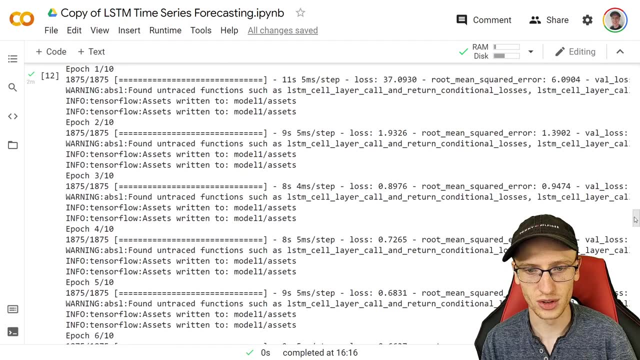 or to make a prediction. We're using the last five hours Of temperature data, except there's no reason we can't just look at temperature. We can look at all these other variables And, if you recall, we have a bunch of them If I scroll to the very top. 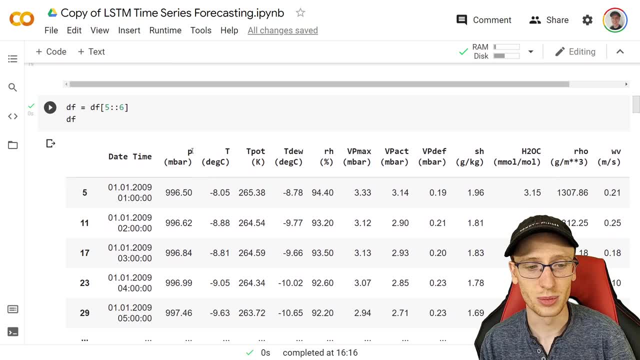 here we have all of this information. Okay, This is pressure. We are using temperature just to predict temperature, So we could use pressure to help predict the temperature and all of these other stuff we wanted to, although we're actually not going to do that. Something else that we 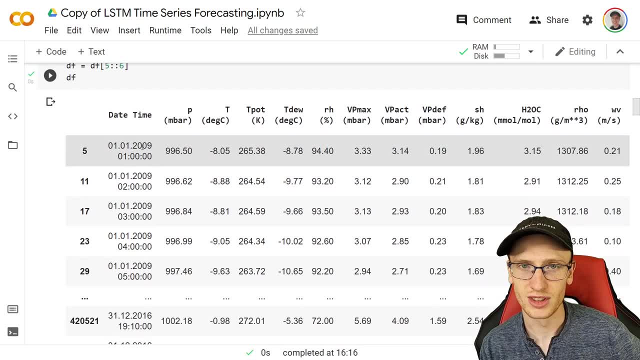 didn't even consider was using the actual time itself as a variable. And you might think like: okay, time, it's a timestamp. Why is that important? Well, actually we have a lot of periodicity here, And if we were to graph it out over time- and in fact- sorry, I hit my computer- 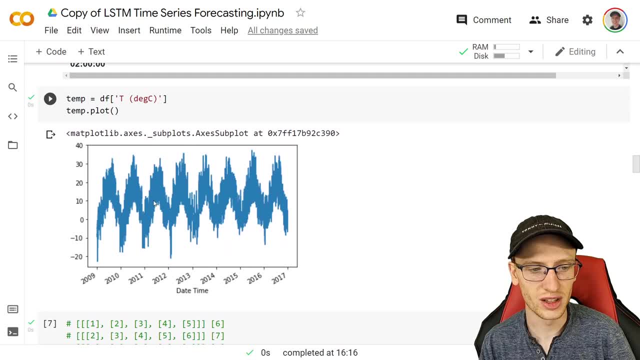 there. If we do graph out the temperature over the years- and we did that- we can see a very obvious relationship here is. you know, it goes up and down like this, And if you think about that, that makes sense for the temperature and it would for many other variables as well. 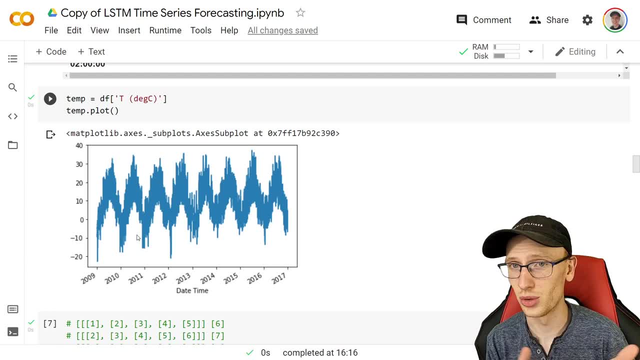 where it's probably going to get hotter in the summer, depending on where you are and assuming you have a summer, like most places do- And, yeah, very, very interesting. So over years we have this pattern like that, And also there's another pattern we didn't even think about, or maybe you. 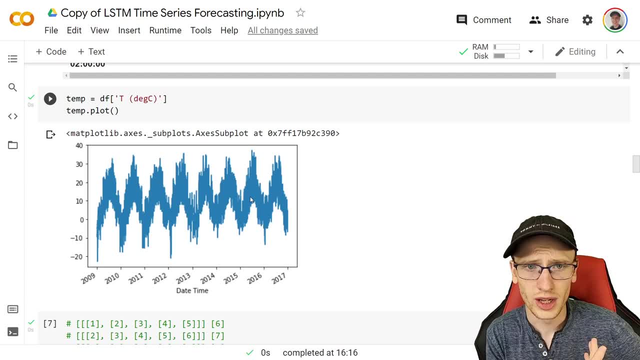 did is well okay. temperature: We know that in each day it's generally hotter in the middle of the day, And I'm not sure if this is true for every location, but I assume it is- It's generally hottest in like the middle of the afternoon or so, And then it's colder and colder at nights, and 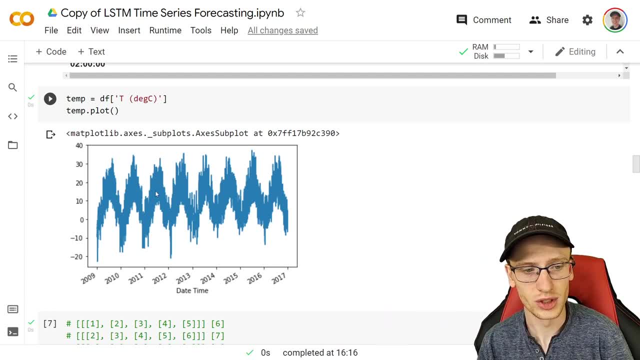 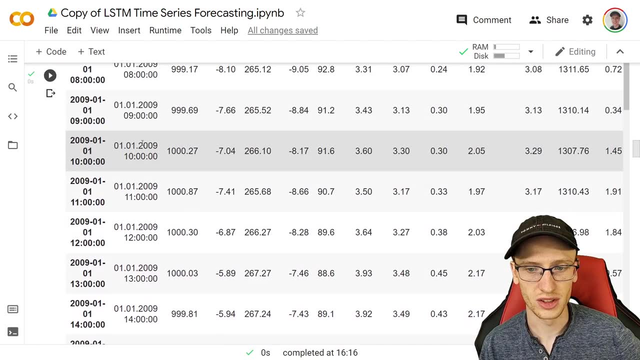 colder in the morning, So it's a little bit different. but it's a little bit different. but it's a little bit different. So we can use that information And that all actually comes from just what time it is here, from that timestamp. Although it takes a little bit, it looks like. it looked like I was scrolling. 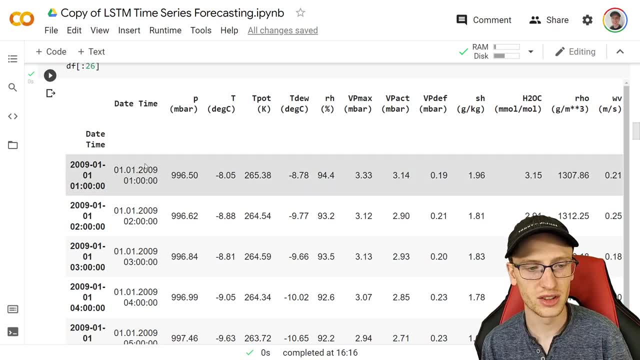 forever there. It takes a little bit of a transformation to get the something useful out of this. we're actually going to be translating it two seconds, just the number of seconds since some certain time, And after that we'll do some sine and cosine transformation, which I don't. 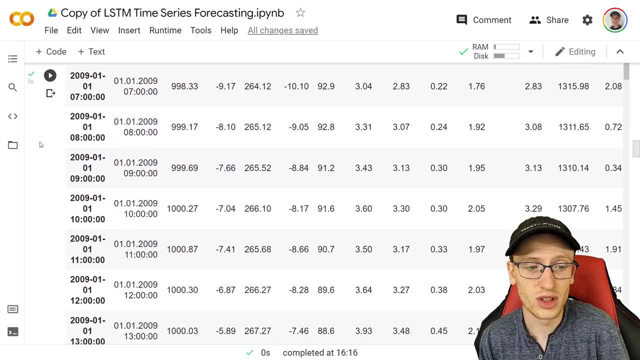 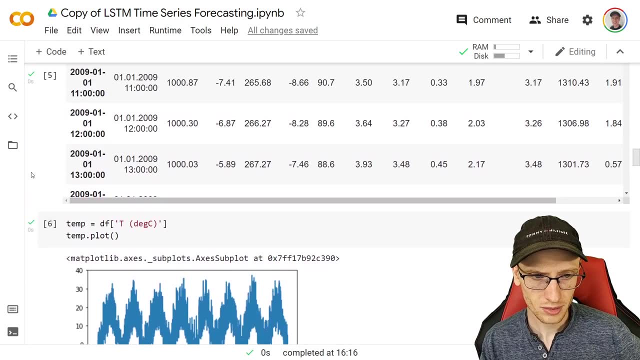 really want to talk about too much. But we're going to do some sine and cosine transformation, which I don't really want to talk about too much. But the point is that we can use that sort of periodicity or just graphically. it makes sense to look like that as variables as well, And 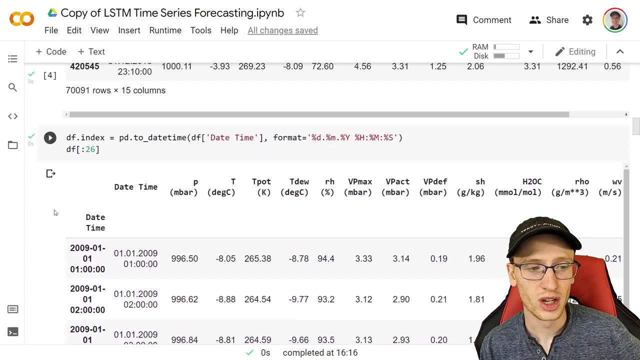 including something like maybe the pressure as well, just to show, we can use other variables here as well, And also there's no reason that we can. we have to predict one variable as well, like there's no need. Well, if you wanted to predict just temperature, that's great. 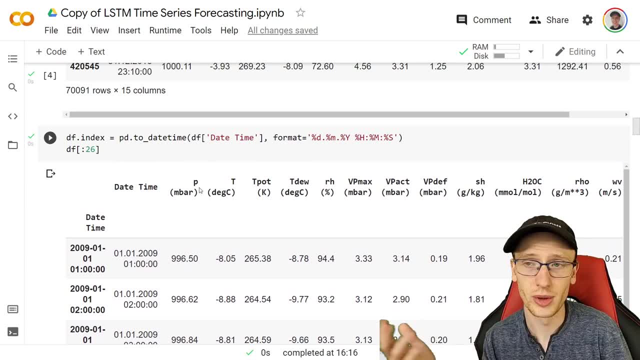 except why not predict the, the pressure at the same time? if we're trying to make a forecast model for the future on climate, I don't know why we just predict pressure. we totally can And it turns out we can do it accurately. 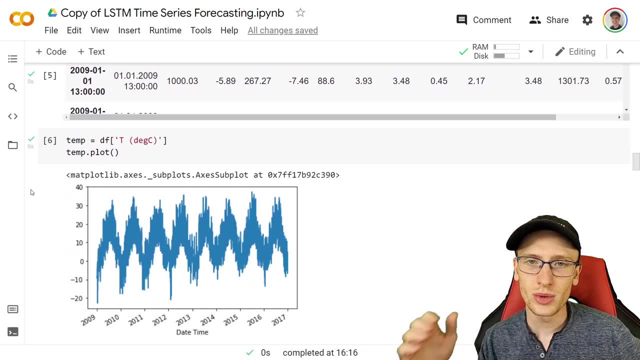 Okay, so there's all of that to consider as well, as. something we haven't talked about is basically LSTM, And I believe I mentioned GRU last time. I'm not sure if I got to that, But basically these recurrent neural networks are generally used or thought of as the go to 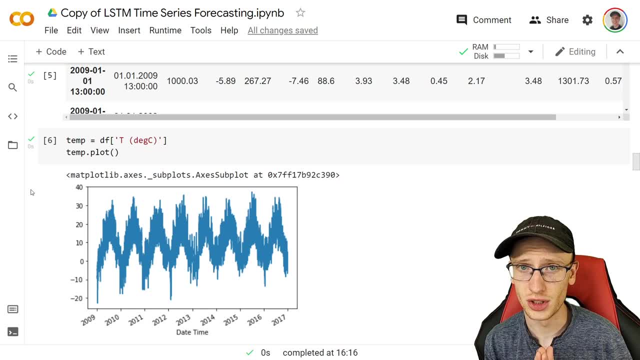 for forecasting stuff, And you know predicting time series data. they're very common in neural natural language processing because they are time series as well, And so they're actually. there's not the only model that you can use. we have these things. 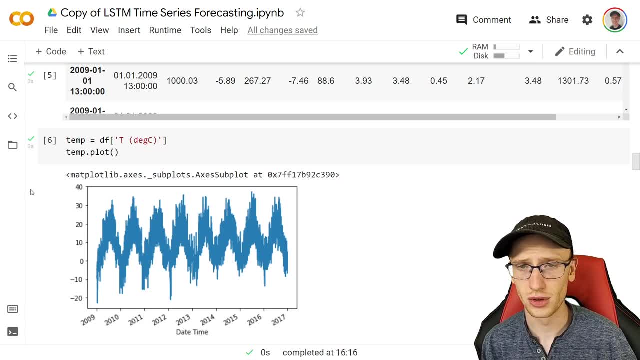 called convolutional neural networks, which people often associate with two dimensional meaning for pictures goes through a picture, except that doesn't have to be true. we can do one dimensional CNNs which go across, go across like that. Okay, so we didn't even really talk about that in the 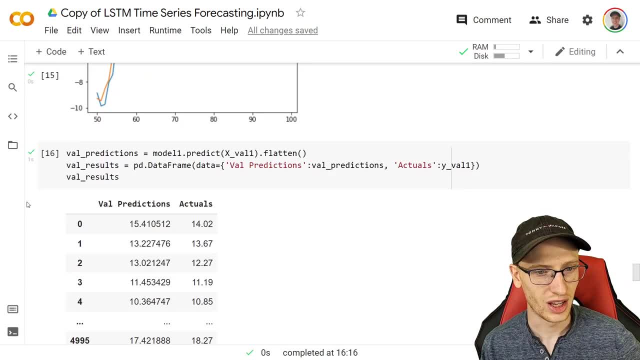 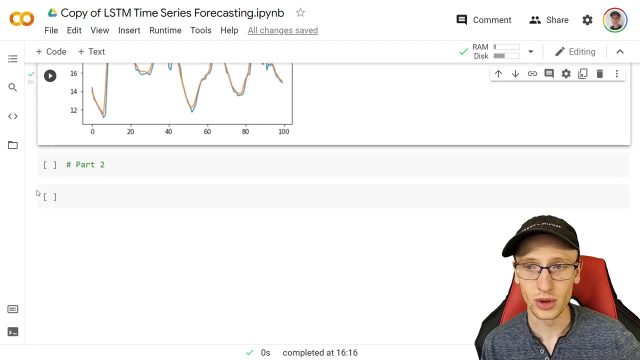 first video. all we did is make that one model And then we showed the results of that model And there they are- train, test and val. And yeah, we're going to be making that today In this next video. sorry, 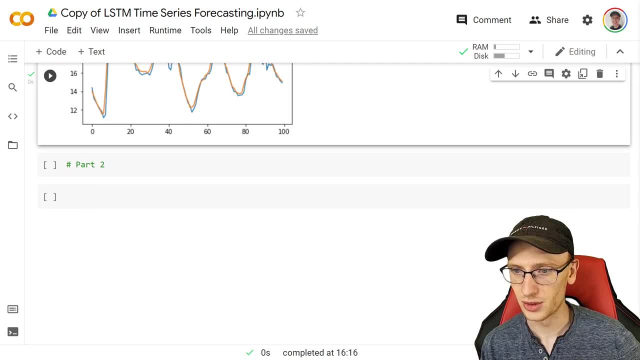 I'm just going to scroll to my other thing to make sure I'm in the right spot. Yeah, so I don't know why people don't really associate LSTMs or CNNs with forecasting as much as they should, because they're a lot lighter weight, as in there we'll find out- there's a lot, a lot less parameters. 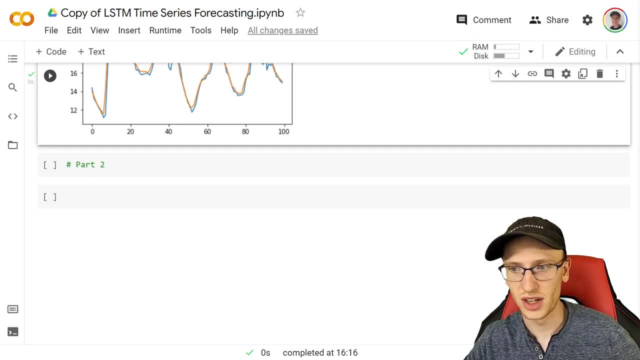 that you can, that you have to learn here which can make your model a lot faster, both in training and action, especially on inference time, how well it can, how quickly it can predict as well. Okay, so a lot of interesting things to think about in this video And we are going to cover. 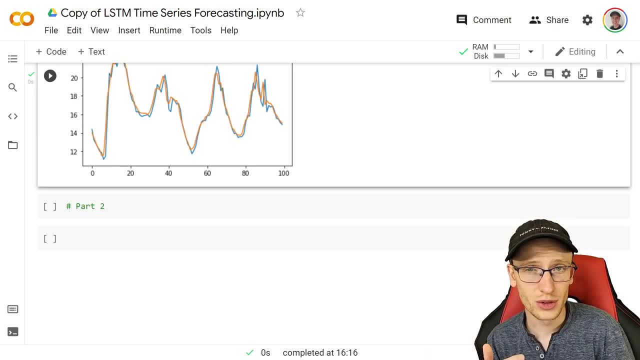 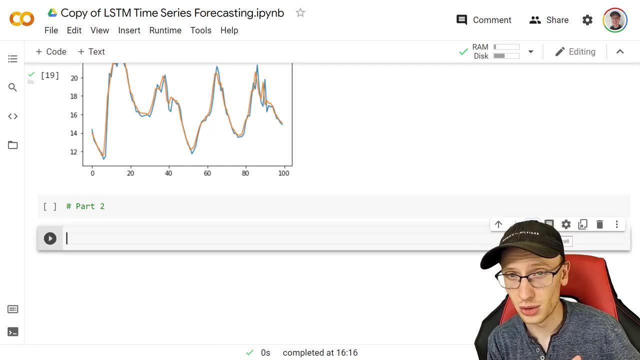 a lot of them, So let's get started. Okay, at this point I am definitely going to assume that you're somehow familiar with our code and what we did last time. So if you don't want to watch that and you want to try and follow along, that's okay. But I'm letting you know if you get confused. 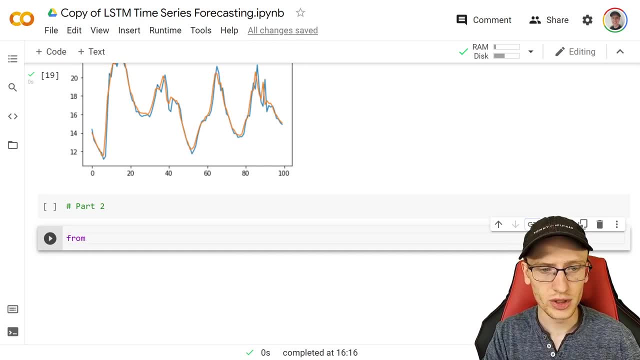 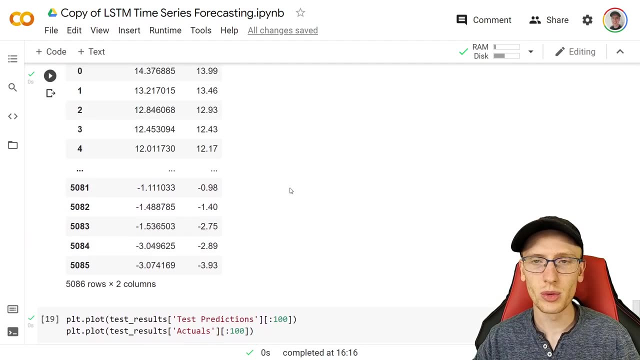 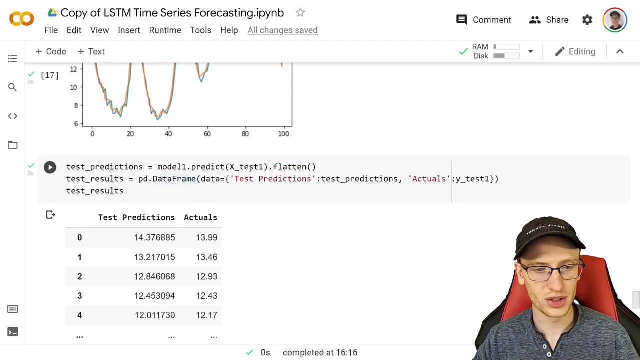 I would probably watch that one first. So to start, we're going to just kind of make a function- that's I should say before I start writing stuff and typing it wrong. we want to automate the predictions and the actuals and this graph all at the same time. So I'm just kind of taking a matrix. 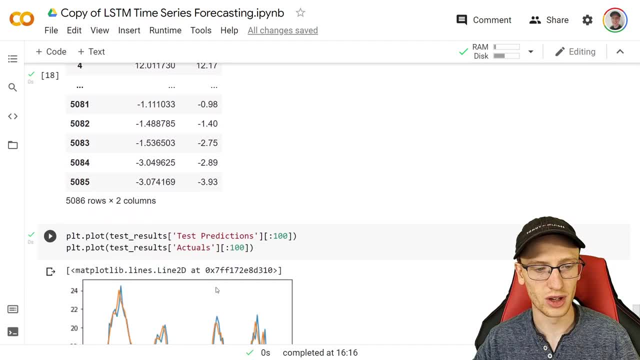 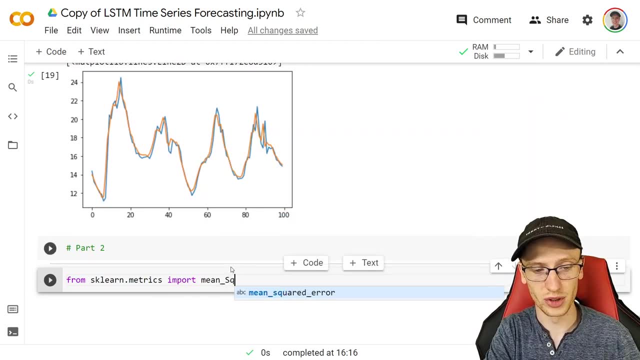 of input and then making a data frame out of it And then plotting those columns. I want to do that all in one function. probably should have done that last time, But it leaves a nice warm up for this time to remember what we're doing. So mean squared error. do that. import that as MSC And 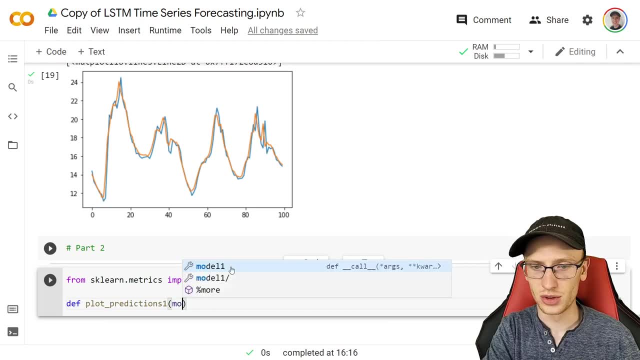 we're going to find something called plot predictions, one which is going to take: take a model, a model in memory, not a, not a model path- although that's an option to model- and x and y and we'll say start and end indices okay, and we're just going to make those defaults to be. 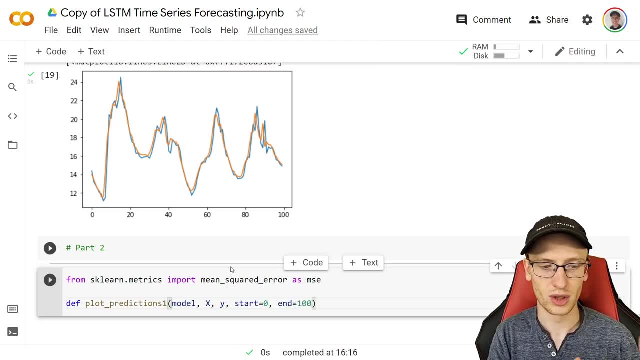 started zero and n is one which is saying okay for this, for this range. you know how much do you actually want to want to plot? and that's just for plotting. we're also going to use this MSC because I want to say the M, the mean squared error, but I'm going to make that MSC over the. 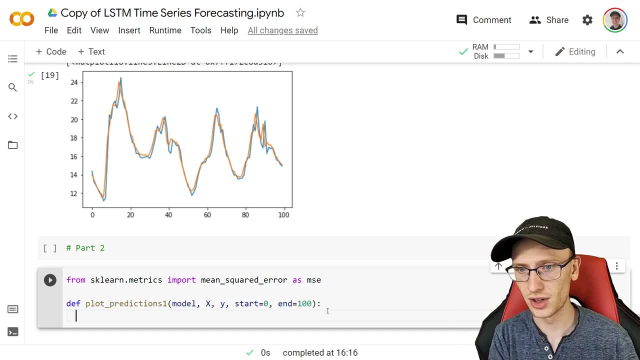 entire set, but the plot is only over the indices specified. Okay, so we're going to get the predictions. that whoa, definitely not predictions. So predictions or Preds, whatever predictions is, model dot predict x And we're going to flatten that as before. 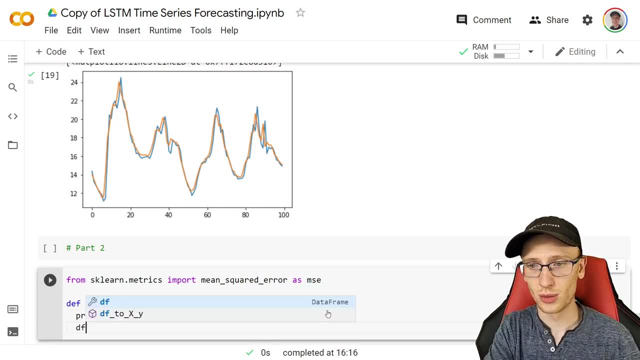 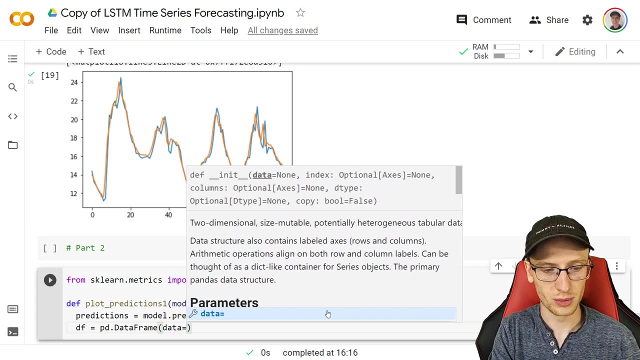 this is really just copying from what's above, but putting it into a function. we're going to make a data frame out of this and do PD dot data frame with those two columns. So that's data. we make it this dictionary we set data equal to. it's going to be predictions And 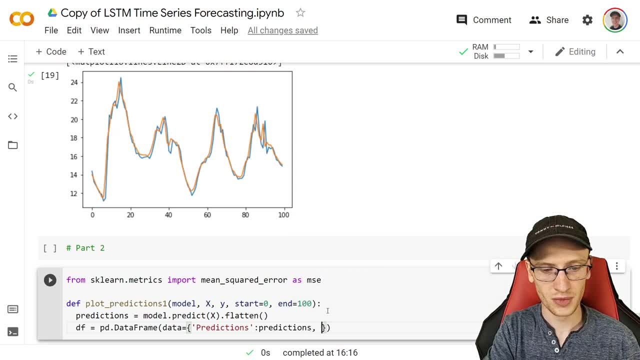 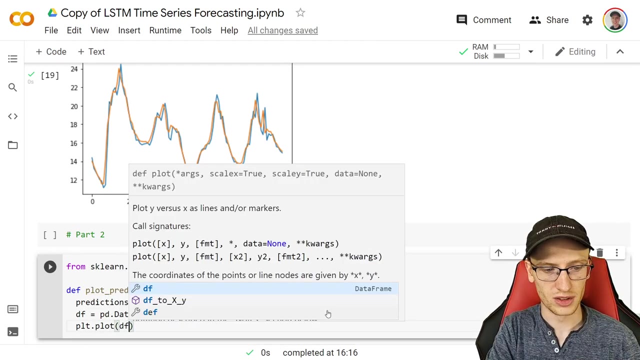 predictions is going to be made up of predictions, And then actuals is going to be made up of actuals, which is why, okay, that vector there. And then we're just going to plot these things: PLT dot plot, And then we're going to plot DF sub. we're going to just plot both those columns. 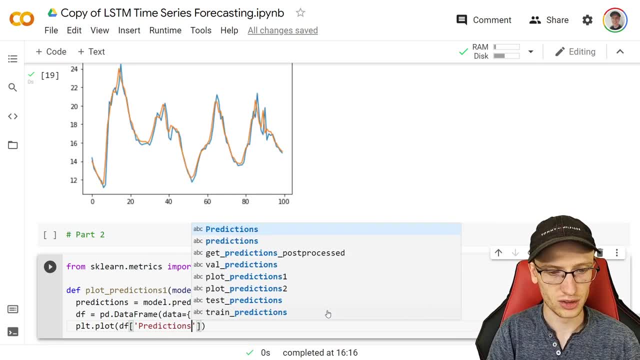 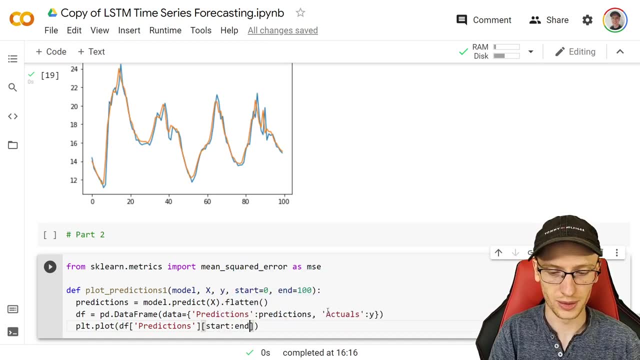 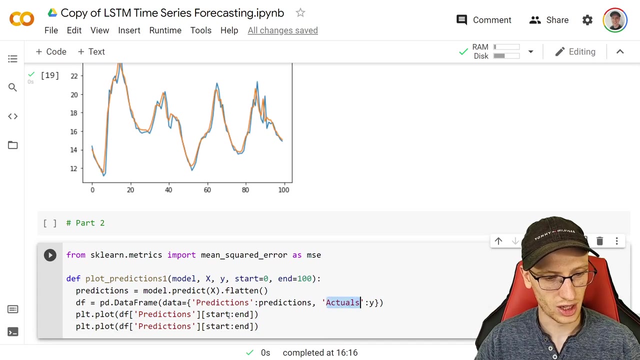 So we'll do predictions, that column predictions, And yes, so how much do we actually want to plot? we only want to plot start to end And we're just going to copy that. copy and paste that, because it's basically the same thing, But we're going to plot. 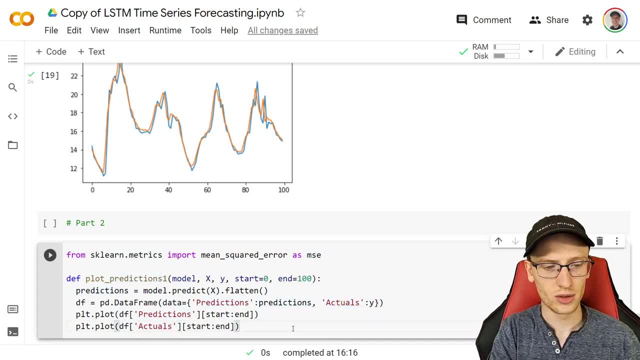 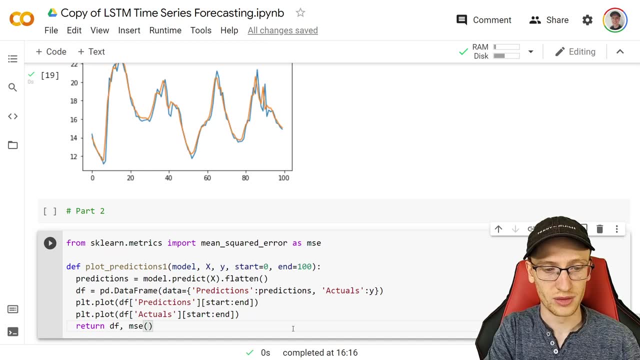 actuals as well, Okay, and we're going to return a couple things. we're going to return the data frame itself as well as the mean squared error of the whole thing. So of actuals, that's going to be y, actually of y and the predictions, Okay. 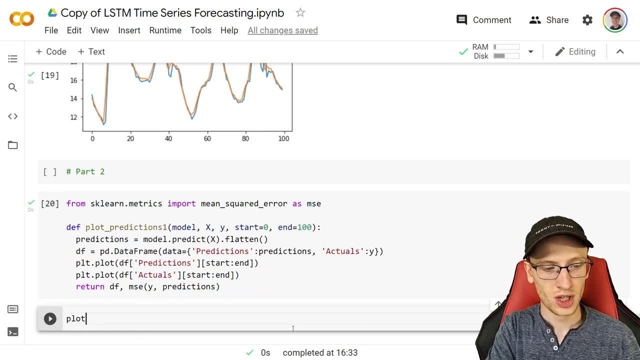 So if we call this like so, if we do plot predictions, most notably we care about it on the test set of information, So we'll pass it model one, our first model, and X test one and X or y test one. And if you really recall, if you literally just did the other tutorial, 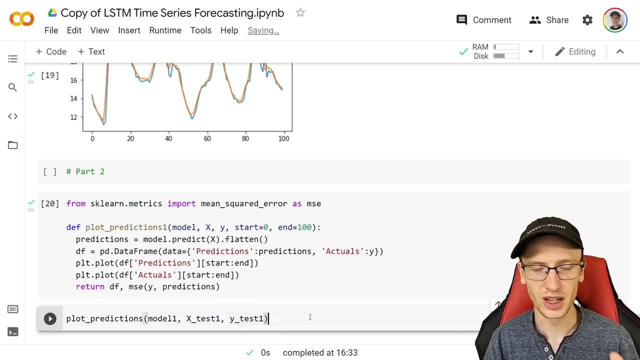 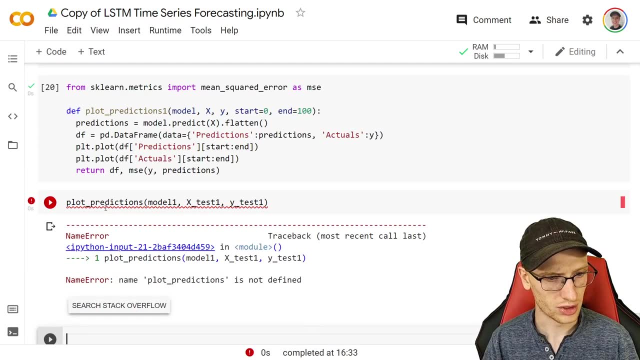 you'll notice probably, these variable names are ever so slightly different. I changed it just to just a little bit to match up with the rest of the code a little bit, but it shouldn't be anything crazy. You guys probably noticed that I spelled predictions wrong somewhere. Oh no, I just have. 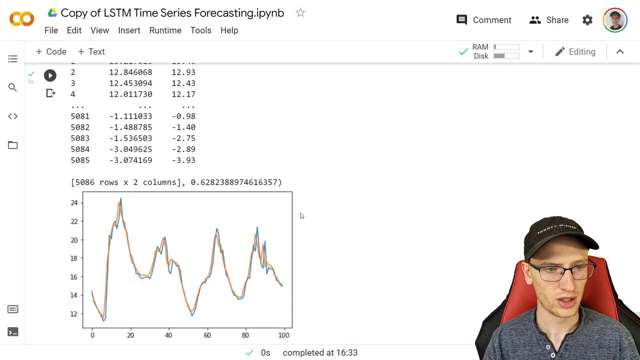 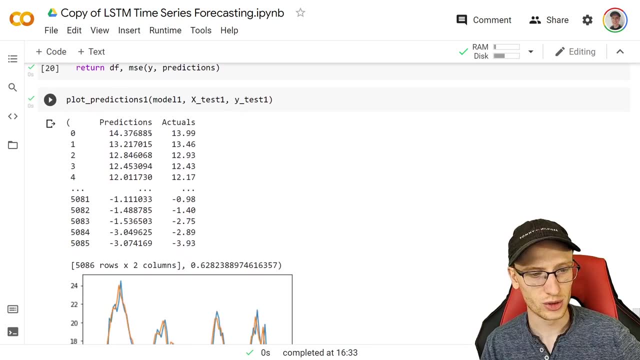 missing a one there And plot predictions one. There you go. So it makes it that's just how it's going to plot a data frame when it's plotting other stuff as well, or show a data frame predictions- actuals. you can see they're very close and the lines together are very close. 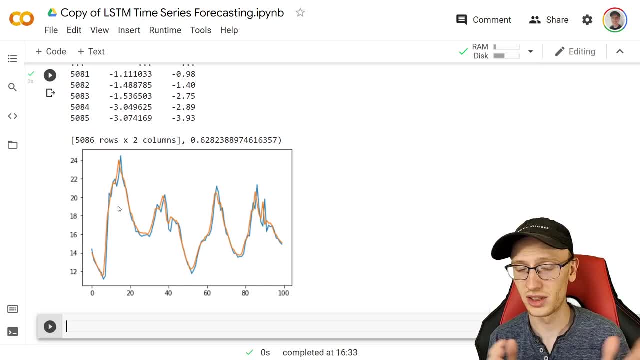 Now again, I was pretty lazy on making the graph. if, as practice, you can absolutely make this a title, some x and y axes and a legend to show which one is which, but I don't really care For the most part, I just want to show that they're pretty close to each other. That's the. that's the main. 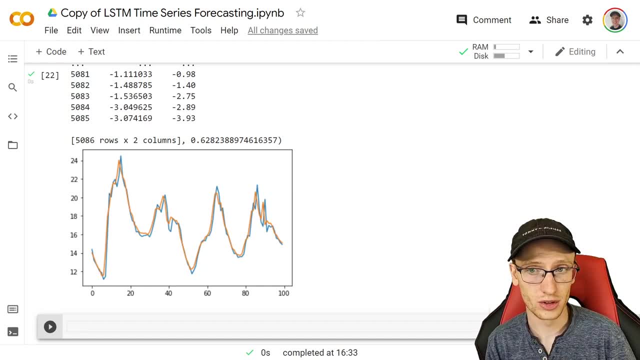 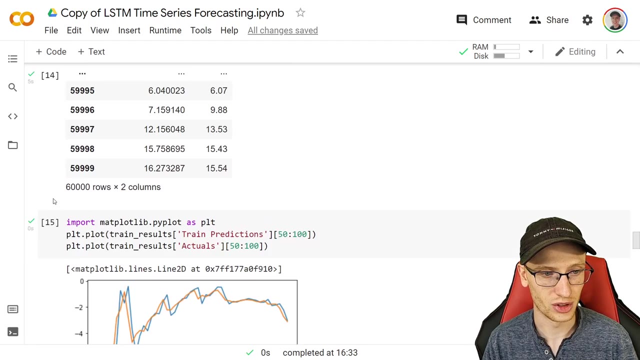 part of this. Okay, so that was one thing I wanted to do, And we'll use that a couple times. Now we are going to make a convolutional neural network model, So we're basically just going to place the LSTM stuff And so just to show you how easy this is- and actually it's how I would do it if 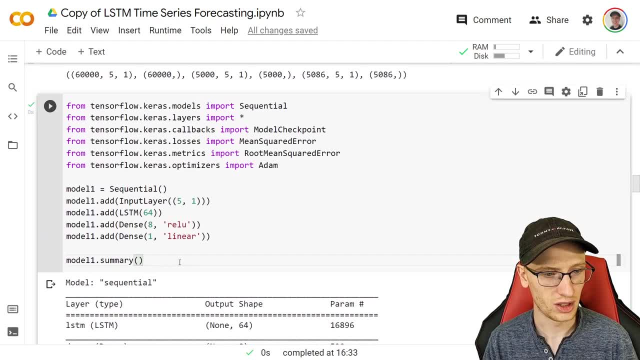 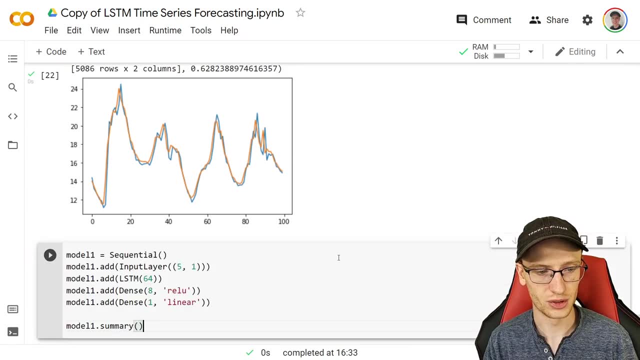 I was making it from scratch as well, like we are going to show you how easy this is and actually are is. I would take the take the model, because a lot of it's going to be largely the same. I mean, you can play around with a lot of it by yourself. feel free to do, do whatever you can with. 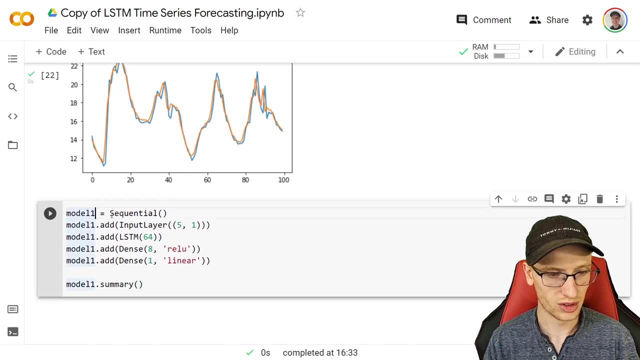 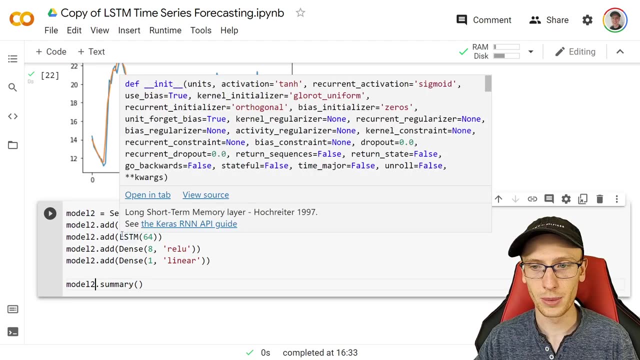 it, But we are going to make the turn the ones into twos. you're going to be seeing a lot of that today. I think we go up all the way to model seven and you can optimally do more yourself, But here so we're happy with five by one. So recall that this is the, the time or the window. 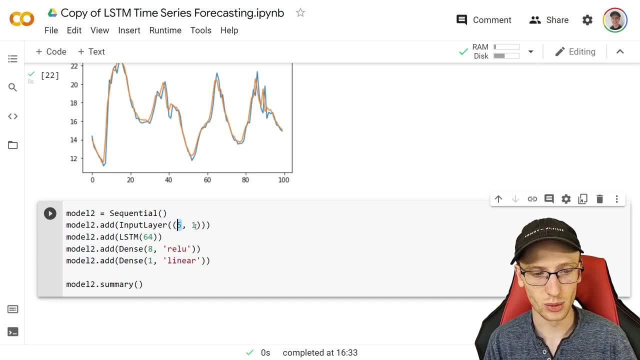 length. we chose the last five hours And the one here. well, one one's often just for formality And for being picky. it wants it to wrap it in a list saying no, we're actually only doing one variable Today. 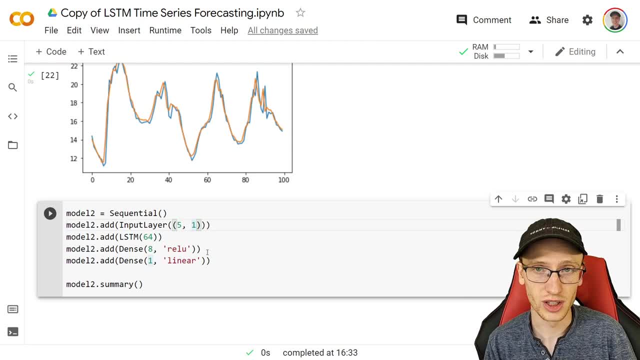 we will be changing that, which is going to be exciting, but not yet. This is still our input and it's only taking the temperature, That's the only variable- more looking at five times. Okay, so now the interesting part is we're going to replace LSTM with a conf one D, And this is 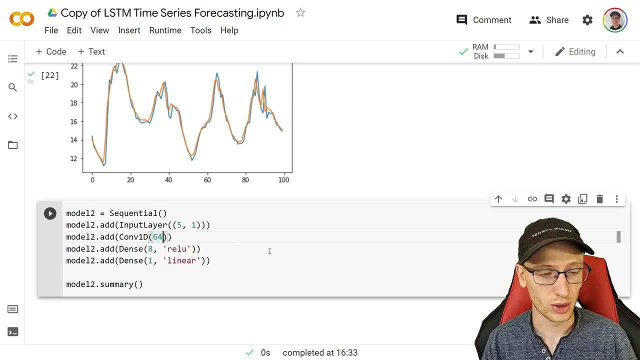 basically the sliding window thing. we slide this window around. So how many times do we want to slide this window? Or actually, how many windows? they're all going to be the same length, but how many windows do we want to slide across? this is going to be this first number we can stick with. 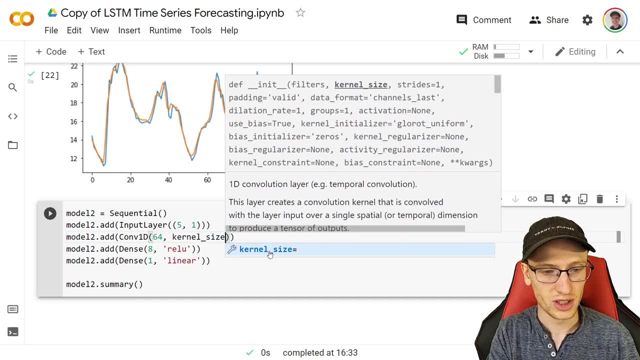 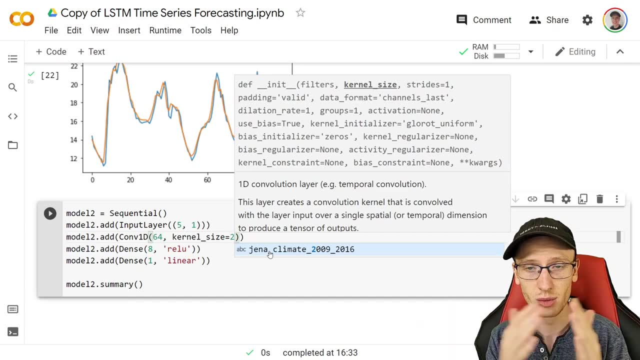 64, that's fine. And kernel size. this is basically the size and it's kind of weird I'm using the term window twice here. the window for the input is length five. we look at the last five hours, But then this window, we actually we actually slide this network window across this thing. So 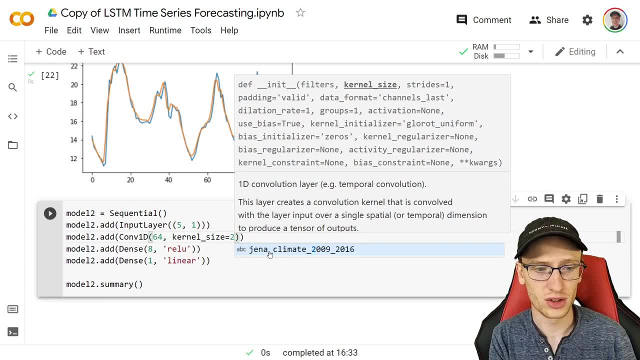 you can think about it as this: Basically, if we choose length two, so kernel size is two. that means- and actually I guess I should use the word kernel instead of windows- is less, less confusing, but people often say window here, this kernel. 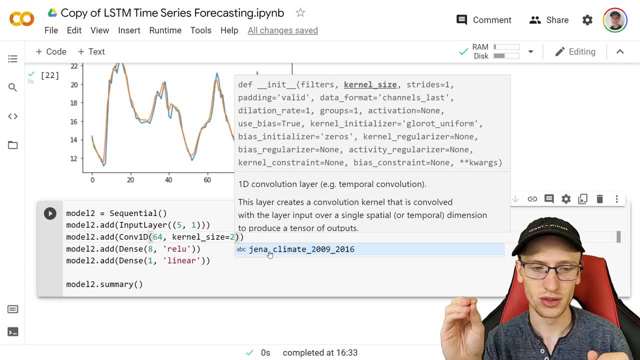 we slide it across and it takes. it goes in order of the input for those five things. It says, okay, take these two things and turn it into one, take these two things turned to one, And so if we're doing kernel size two with a window of five, it's going to fit into the first and second spot. 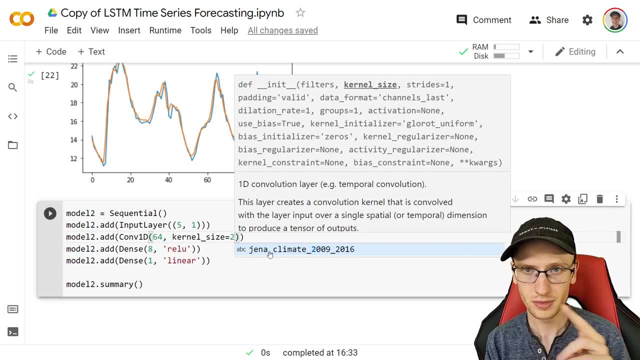 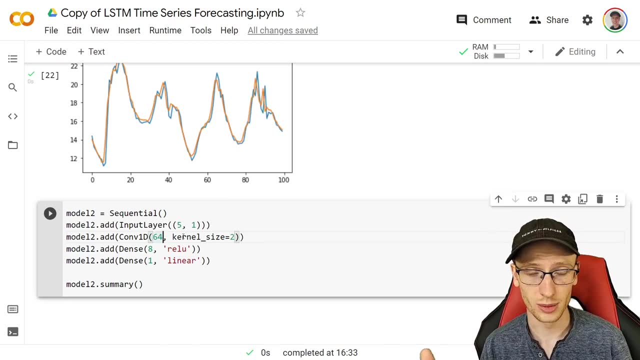 second and third spot, third and fourth spot, fourth and fifth spot. that would be four locations that it could fit, And so it's actually going to turn this into a. so it's going to do that 64 times. So 6064 by four is what it would. 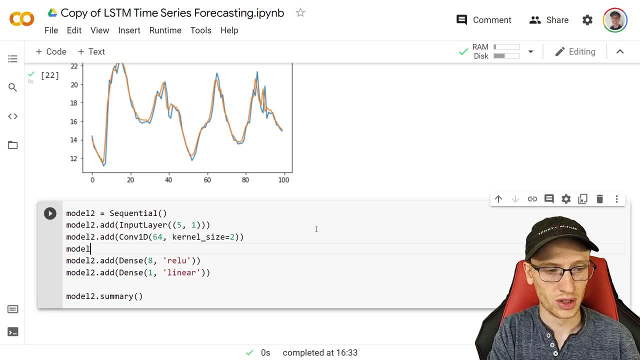 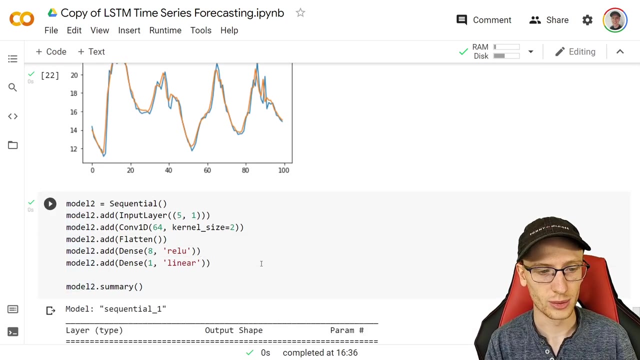 turn that into, And then after that we would need to do flatten model to dot add flatten, because we don't really want it in that, this weird kind of two dimensional form, And we'll flatten it so that we can convert it to eight relu's, as before, And our summary: 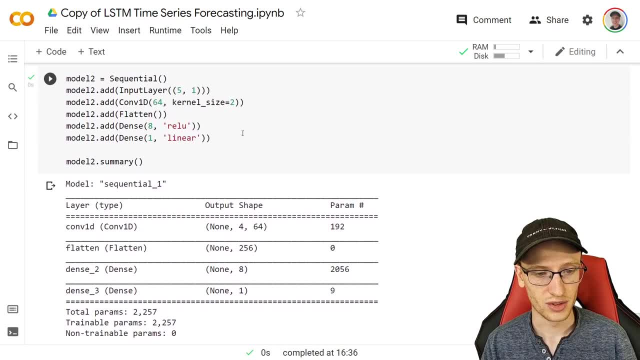 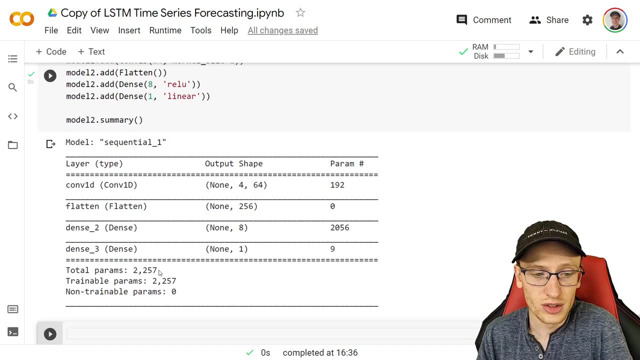 is as follows, as we said. so it's going to take five by one, and then it turns it into four by 64, 64 by four, really this same thing. And here total parameters is 2257.. Isn't that just incredible? 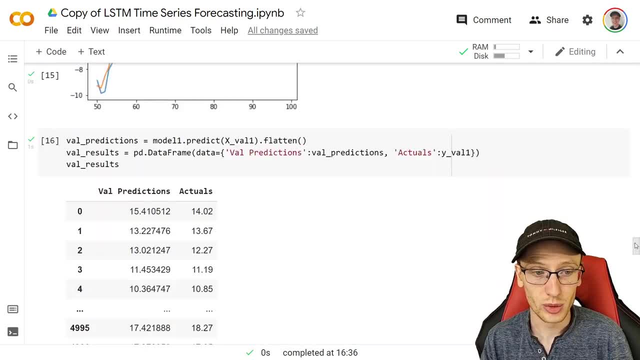 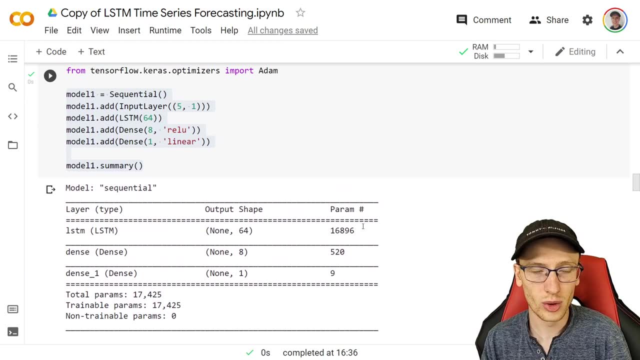 like 2257.. If you recall, and we like low parameters for the most part, the course complexity in the model helps us be accurate. But that is way, way, way less parameters than this thing- 2200, compared to 75,000.. So that's a lot less parameters than this thing- 2200- compared to. 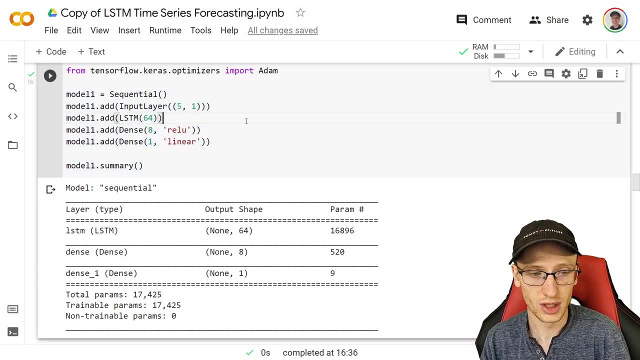 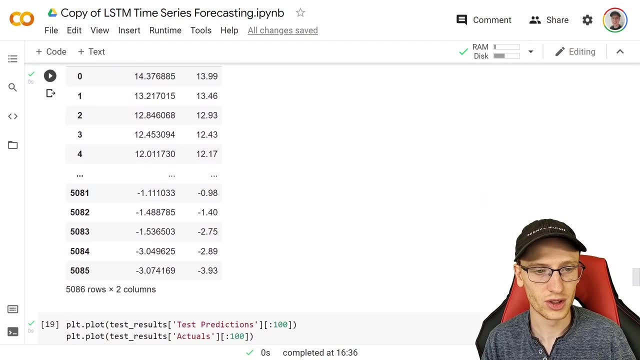 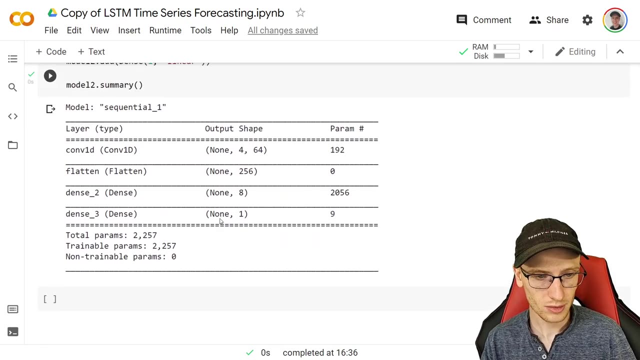 17,000.. Even though I both I chose 64 for both of those things. So that's incredible. GRU, which we'll actually see after as a replacement to LSTM, it's another recurrent neural network And that one will have basically a balance between the CNN and an R and the LSTM. But anyways, 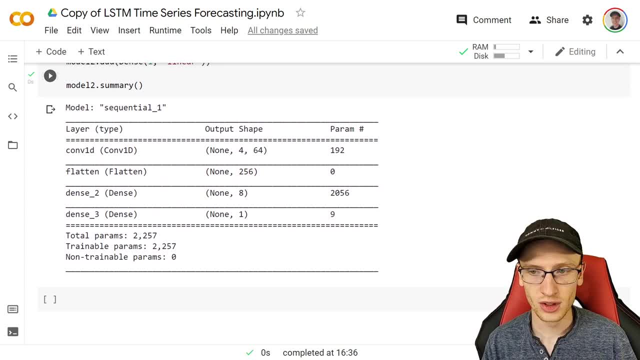 for now. yeah, this is really really good that it's low parameters, because it's it'll make the model run faster, easier to train and and many other things. Okay, so, after we've made that model, we are going to- and I'm just going to choose make, I'm going to be copying from this: 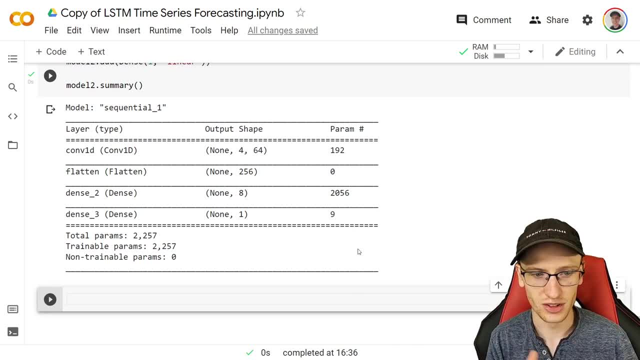 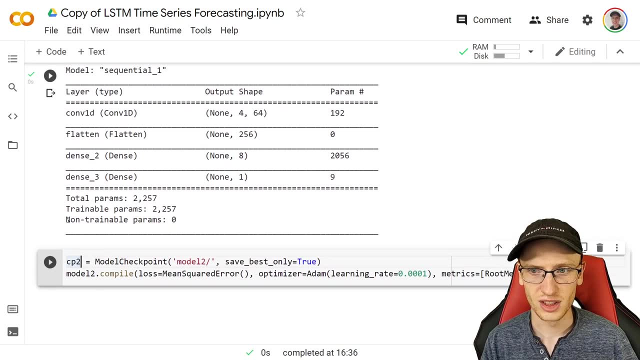 other notebook. it's actually just copying from the same notebook as above. I just don't want to give you the headache of scrolling up and down. we're going to take the, the checkpoint code, which is that's a CP two, which is kind of confusing because we haven't done a CP two yet. So actually, 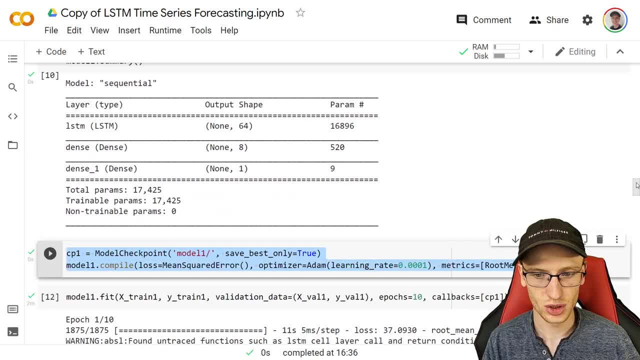 let me just show you CP one and we will translate that. we will convert that in CP one. So I just lied, I said I wasn't going to scroll up And I did. Really, all I'm going to do is I'm going to. 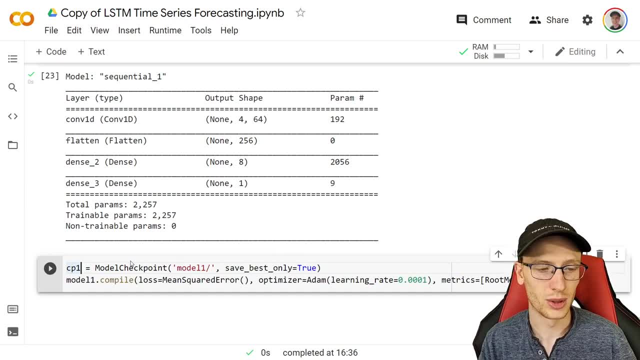 doing here and I'm going to be less picky about this later on. So we're going to do it a bunch of times. But CP one, we're changing that to CP two, we're going to be saving model to model to dot. 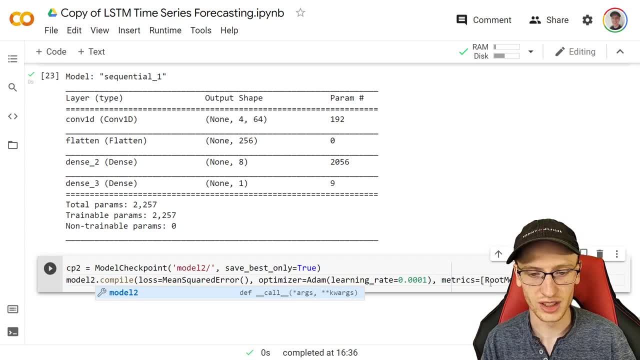 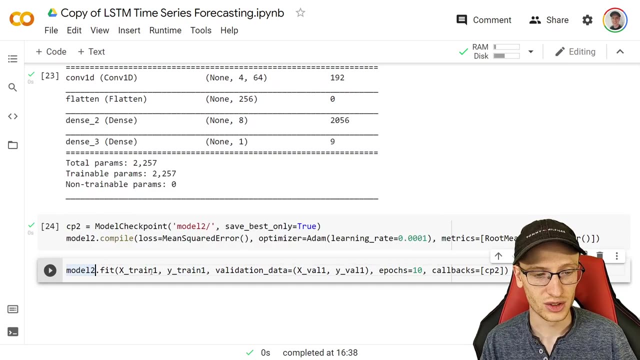 compile mean squared error is fine, optimizer with this learning rate is fine, and so on. Okay, compile that And we're going to copy, and I'm just going to make this exactly as it is in my other notebook. here you can follow along pretty easily. model to dot fit: x, train, y, train. 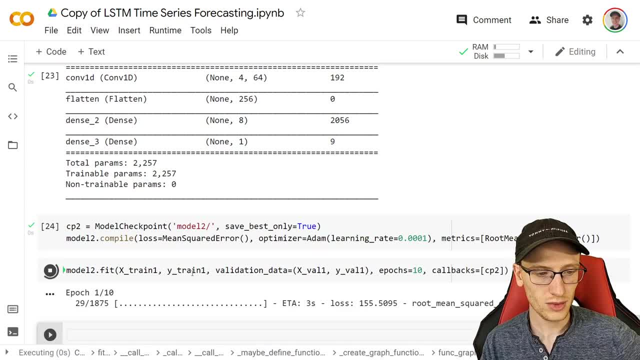 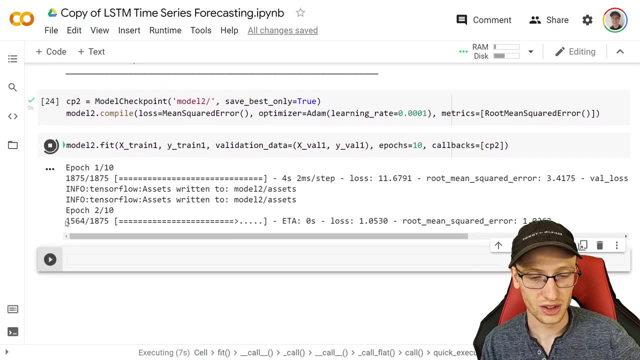 x value, y val and make that the callbacks. So we'll fit this convolutional network model And we can see it trains very quickly. the loss is going down as is expected, and desired root mean squared error as well. That's just the square square root of it And that's going to go for a little while. 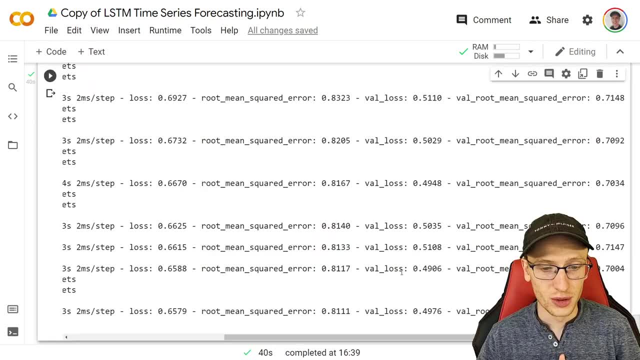 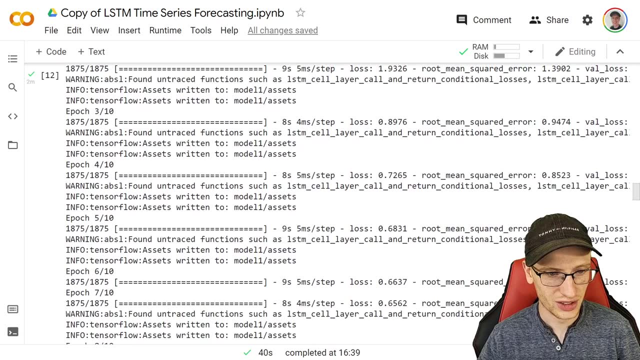 I don't really want to keep talking for the next minute or so. Okay, I'm back. So, val loss. it went down to about point four nine, which is great If we compare that to our earlier fit above. I try not to do this. I know it's a big headache to scroll up and down. 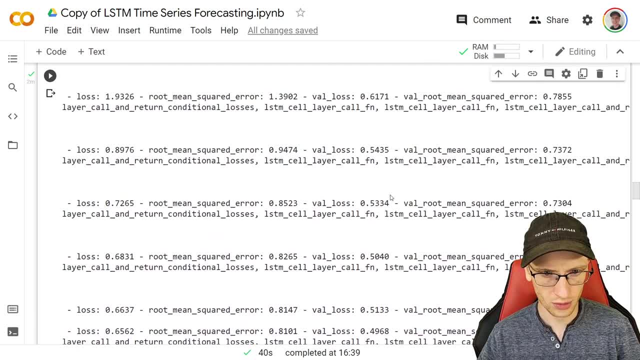 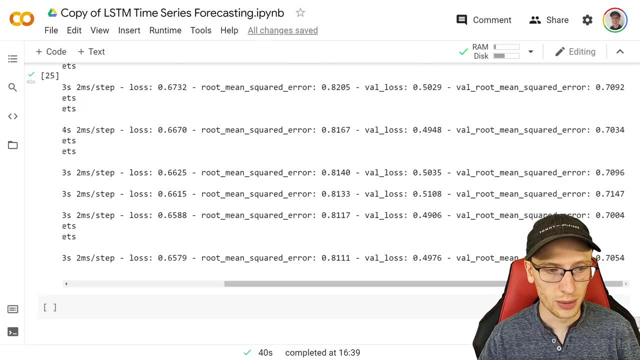 Val loss we got to about, you know, 4.87 before seems to be the best one, So that's pretty awesome. They're pretty much the same validation loss, Very, very similar, But the complexity of this model is significantly decreased. like this model would run a lot faster, most likely. 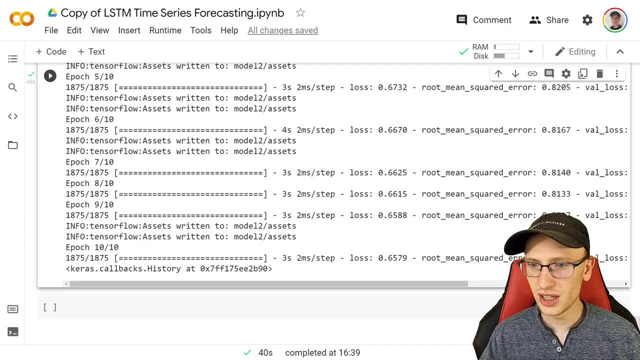 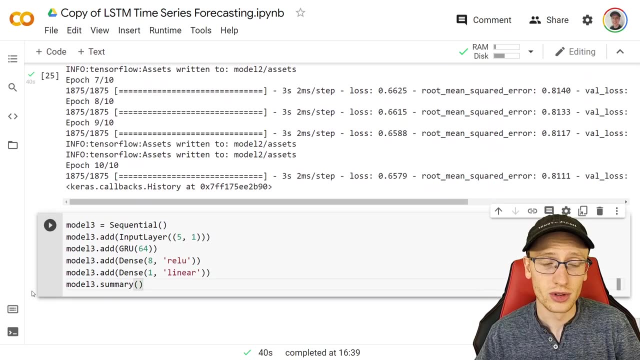 So we would probably prefer that. Okay, so CNN is a great option to think about when forecasting. And just another warm up before we move on to more variables is replacing it all with GRU, And GRU stands for gated recurrent unit. it's basically a simpler LSTM And I just copied this code in. 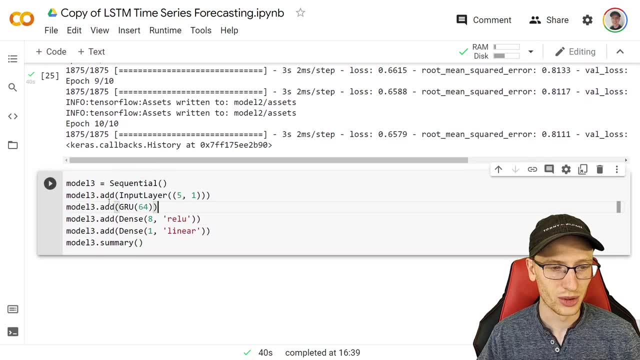 because it's really the exact same thing as the LSTM code with model I called it model three, And same thing takes the same input, except the LSTM is replaced with the word GRU And our summary should look very similar, Except here we have 13,000 parameters. 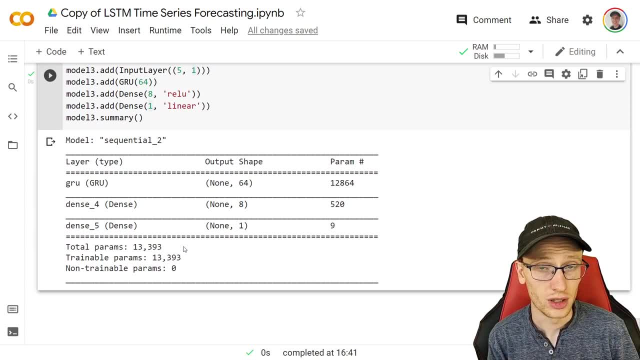 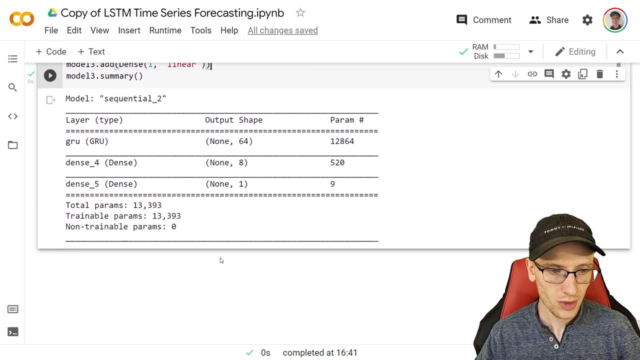 which, as I said, is between the CNN and the and the LSTM. So it's it's much more like the LSTM, Though it's fundamentally a lot more like the LSTM, Okay, So, yeah, so it's another recurrent neural network And it's- it's a decent option. The reason you might want to use it is because 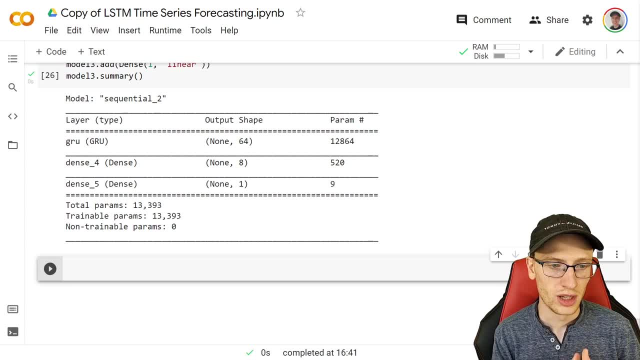 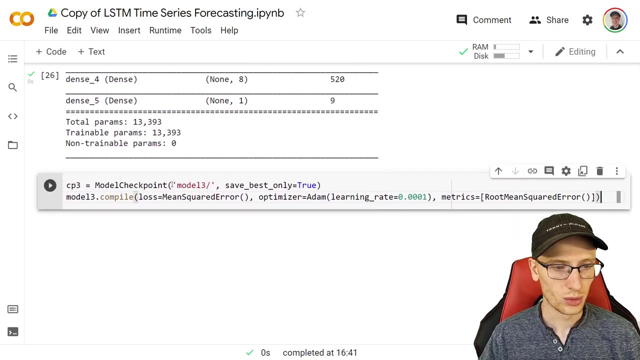 you know, complexity is not always a good thing. It's. you know, it makes it heavier and a more more slower to use model, as well, as you're more prone to overfitting if you have more parameters and more complexity. So, yeah, you might want to use GRU every now and then. So we're gonna get. 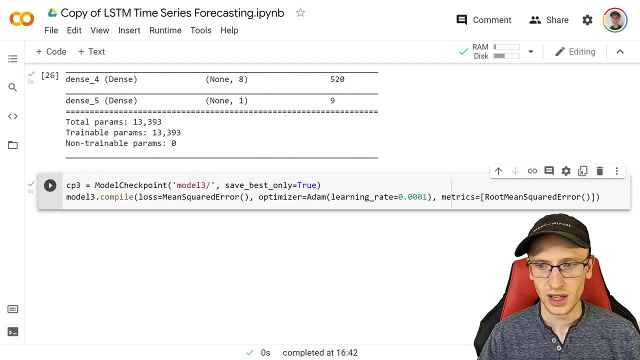 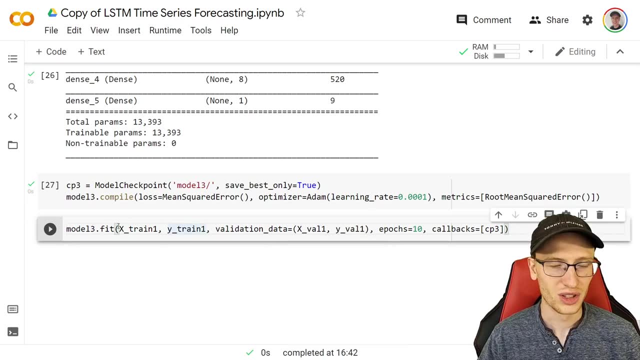 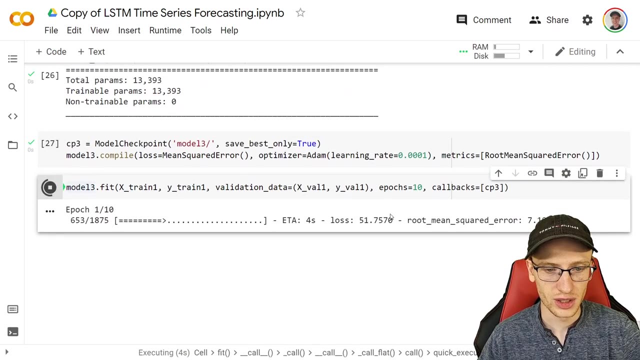 three, three, three, and that's fine, And I will train model three as well. I apologize for getting code out of midair, But it's really just it's it. you can follow along with it pretty easily. if you've seen the other stuff, I think, So I'm gonna let that go And yeah, losses going down. 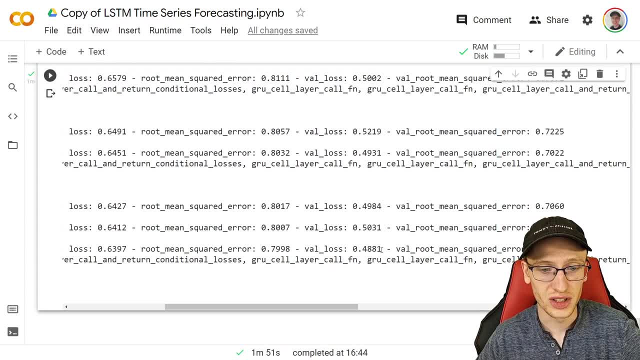 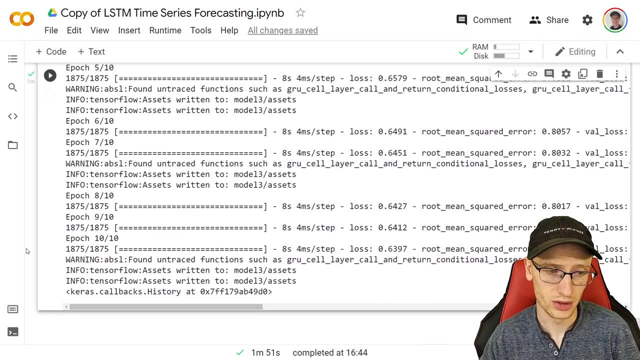 down, down. Okay. so on epoch 10, we got the. the validation loss is about point four, eight, pretty much the same as the other ones, And so, again, we would prefer this model over the LSTM. we'd probably prefer this, prefer the one DCNN. 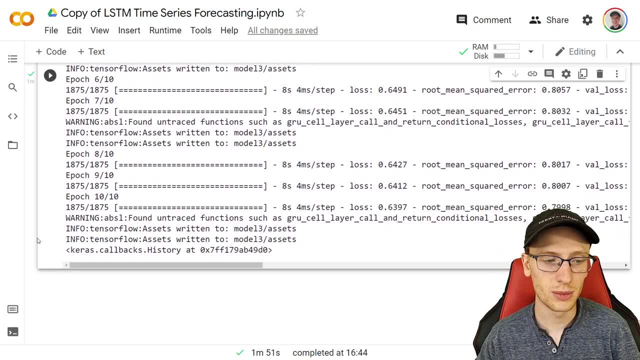 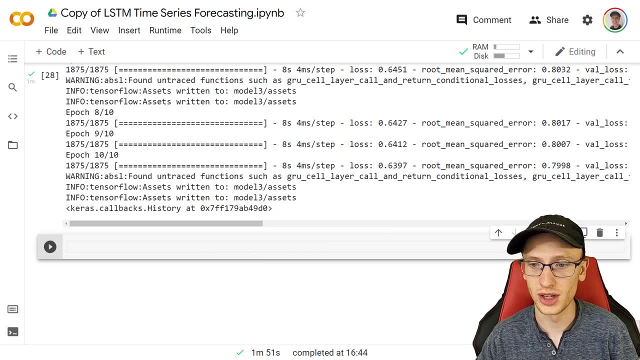 Most actually, but we definitely prefer this over the LSTM Because it's the same, pretty much the same- accuracy and idea, But it is it's less. it's less parameters And that's generally better if we can do that, Okay. so now we're going to move on to the idea. 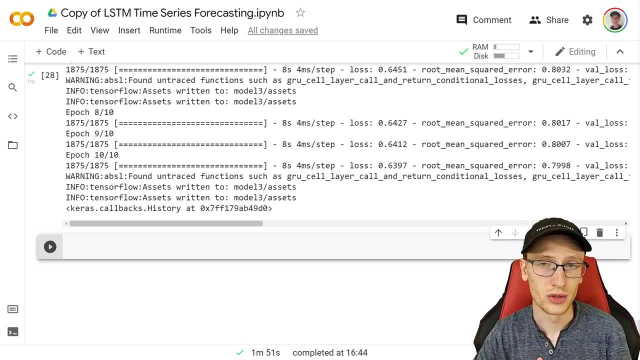 basically two ideas in. one is using multiple variables, So we only use temperature. before we looked at five steps of it, But we only used one temperature or one one variable, So we're gonna use other variables as well as this idea of translating a time into our time. 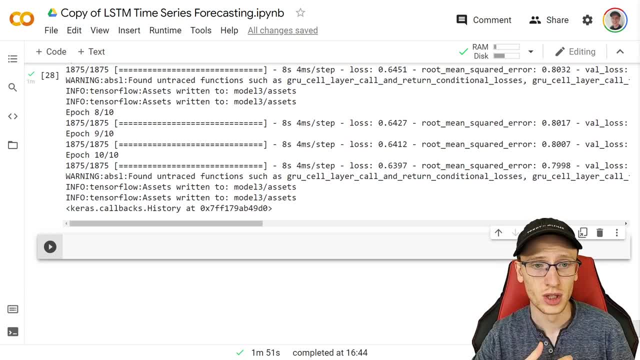 stamp into these usable signals. we're going to convert it to this one timestamp. we're actually going to get four columns of interesting, very important features out of it, which is the day signal, both day sign and coast signal. So there's two columns there: day sign, days, day coast. 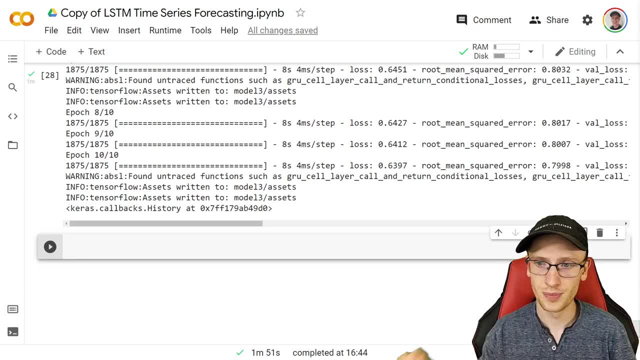 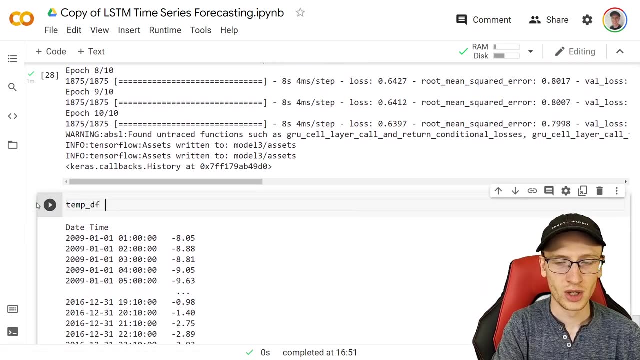 as well as the year, year year sign and year year coast. Okay, so to do this, we are first going to add a seconds column to temperature. Firstly so, if I just remind you, we have two columns here, And so we can make this new kind of data frame, which is temp. df is equal to 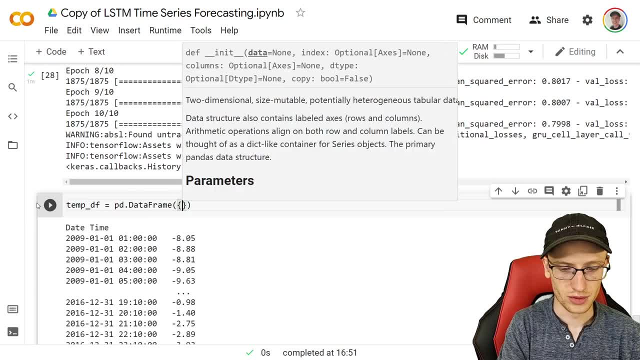 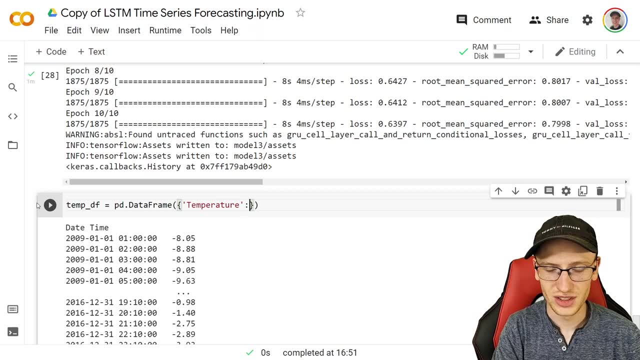 the PD dot data frame out of out of temperature And this is a little bit weird, that we're just making a data frame with one column which is kind of like a series, except there's a reason for it. So PD dot data frame like that. if you want to see what that is, it's just 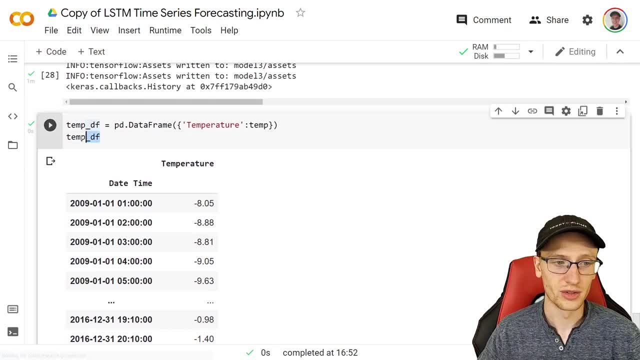 it's just the same thing, but it's going to output it like it's a data frame, because it's a data frame. Okay, so we have that And we can see the index, this, still this, this timestamp here, which is going to be very useful So we can add temp df. 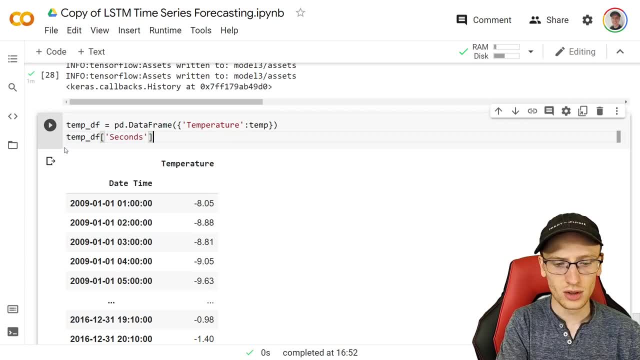 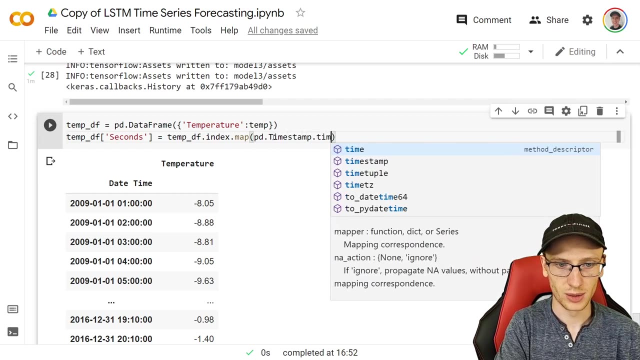 sub seconds. seconds is equal to temp. df dot index. Okay, that's that. that's that date timestamp, date time column there And we can map PD dot timestamp, dot timestamp. Okay, and it's a little bit weird how that's what that does, But here. 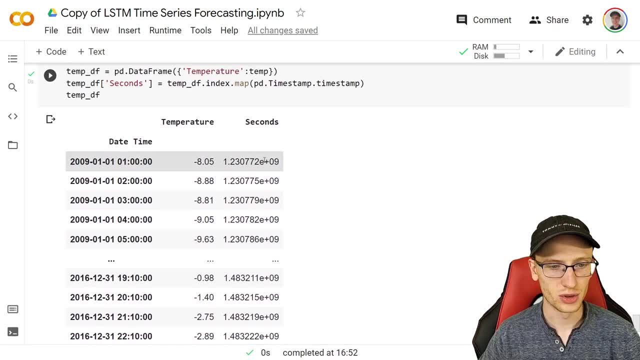 if we look at this column, this, this new column, here we have seconds which looks like some really big value. it's 1.23 times 10 to the nine or whatever. So very big value. And what is it? 1. 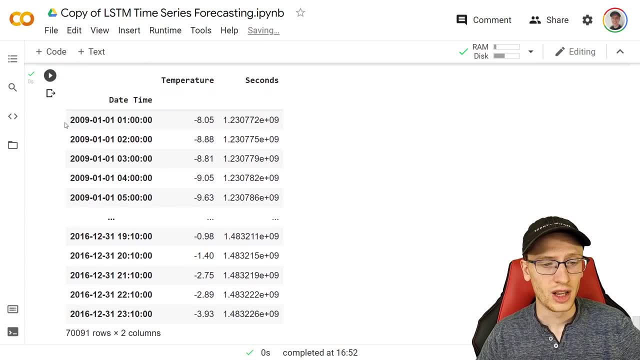 billion, I guess 1 billion seconds, I guess, if I have that right. And so why isn't this zero seconds? because this is the first time we have. basically, it's actually not. this is not zero seconds because this is all from some earlier timestamp, But it doesn't really matter The point. 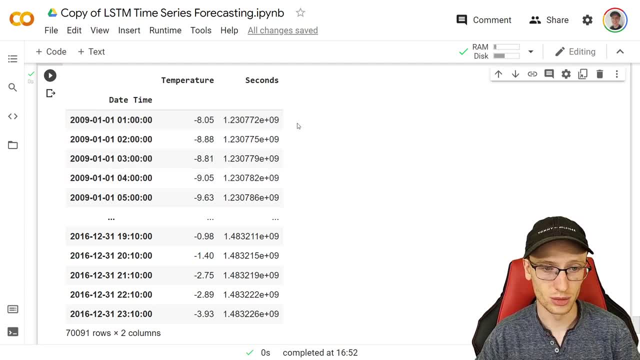 is. this is just some increasing value, that's according to what the timestamp is. So you could, if you wanted to subtract some value, to get this down to this, down to zero and then so on, if that makes you feel better, but don't really, doesn't really matter. Okay, so we have this now as 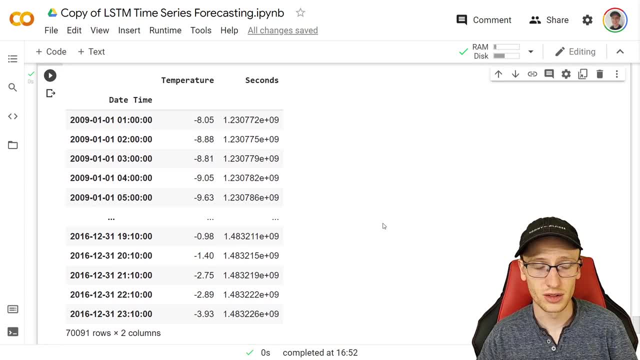 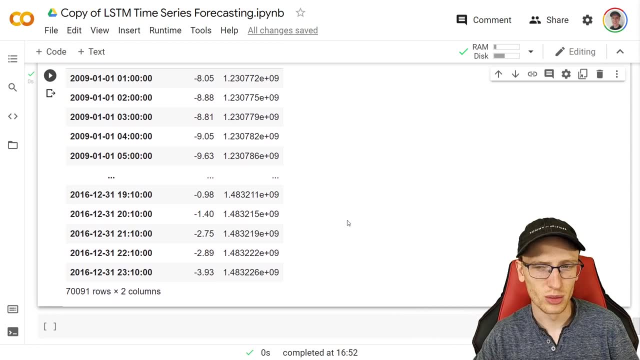 seconds, And so this is a big stepping stone to converting this to day sign, day coasts and your sign, your coast signals. And I know if you haven't heard that before, you don't really know what I'm saying, But it doesn't really matter. 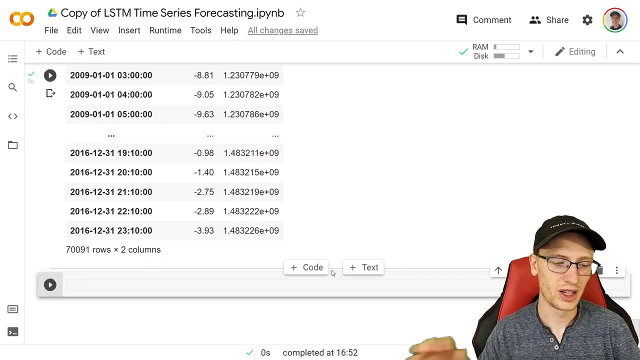 I'm going to plug in. well, okay, I'll write this out by hand, just so you can get an idea for it. So we're going to get two numbers here, which is day and year, Basically the number of seconds that are in a day and the number of seconds that are in a year. 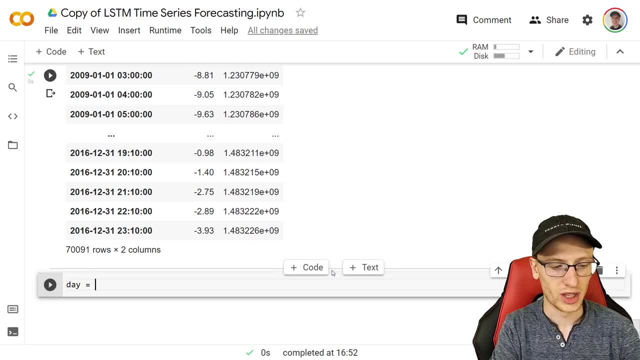 So it's a lot. So day is going to be well. we have 60 seconds in a minute and 60 minutes in an hour and 24 hours in a day. So 60 seconds in a minute, 60 minutes in an hour, 24 hours a day is the number of seconds we have in a day. 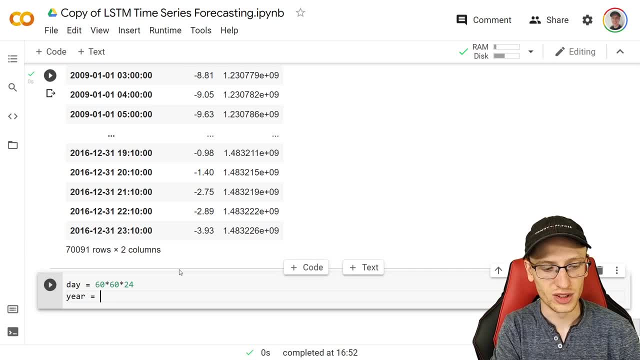 And then if we have day, then we can say year is equal to, and it turns out not to be 365, but more like 365.2425.. It's kind of weird. That's what it is: Years in a or days in a year. 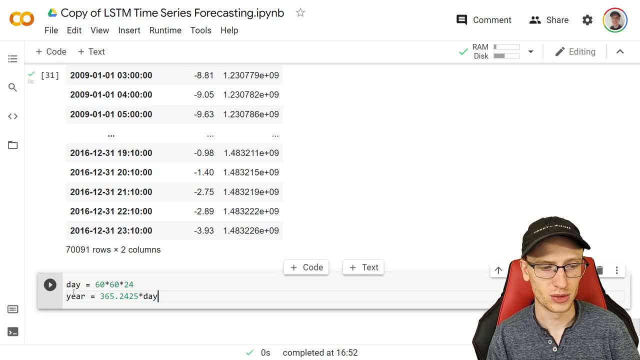 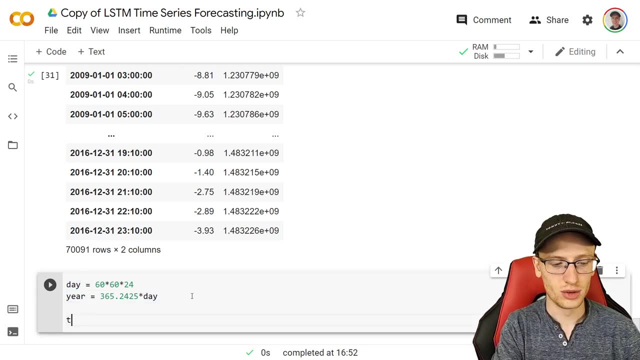 And so if we multiply that by the number of seconds that are in a day, this really should be called number of seconds in a day, but just day for short. So this would be number of seconds. So it turns out we can use these signals to do something like temp, D, F. 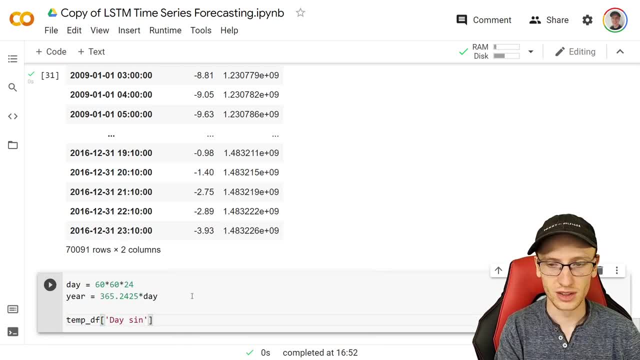 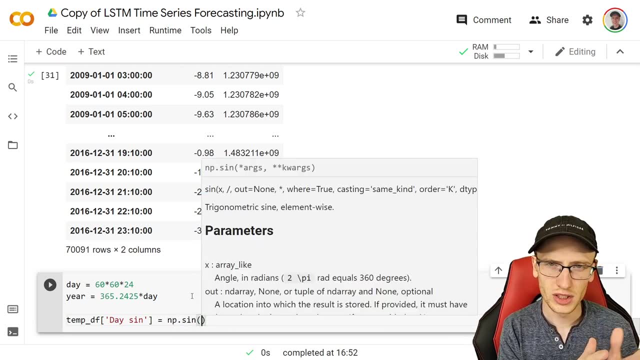 We're going to add in a column here. We'll add first the day sign signal, And this is going to be equal to well, something about sign. unsurprisingly and not really going to explain how this works. too much, Go ahead and read about it on your own. 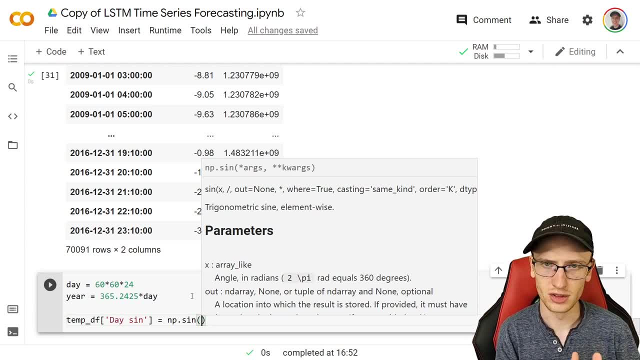 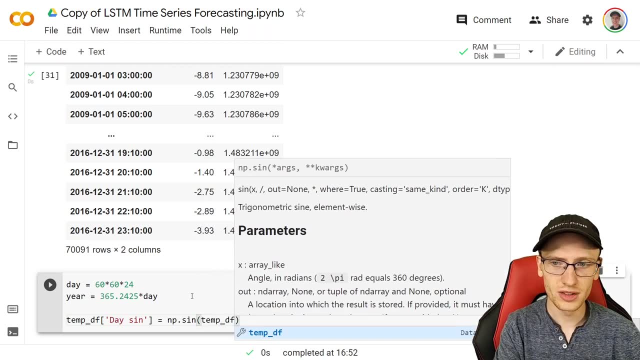 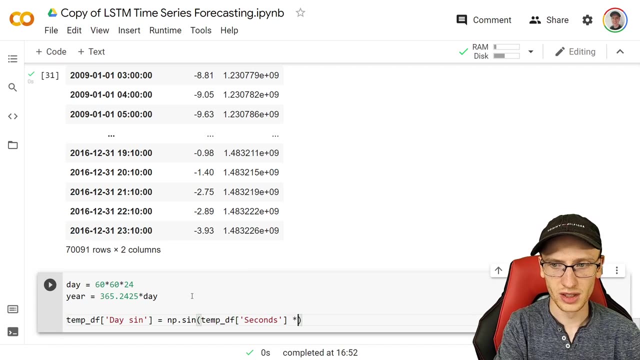 If you want to, basically converting period signals into sign and time into period sign and cosine signals. But we're going to add in, make this some sign Where we do temp, D, F, sub seconds, seconds, that, and then we're going to multiply this by two times pi, or num, pi, dot. pi is stored in there. 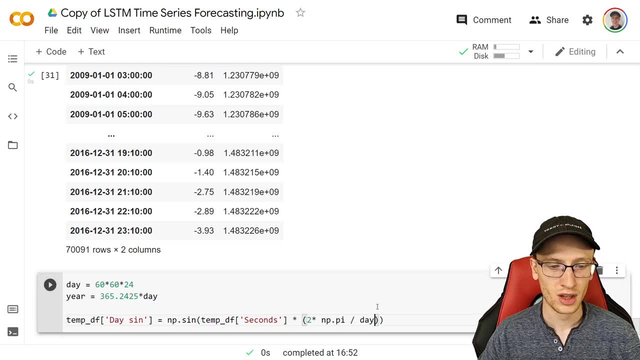 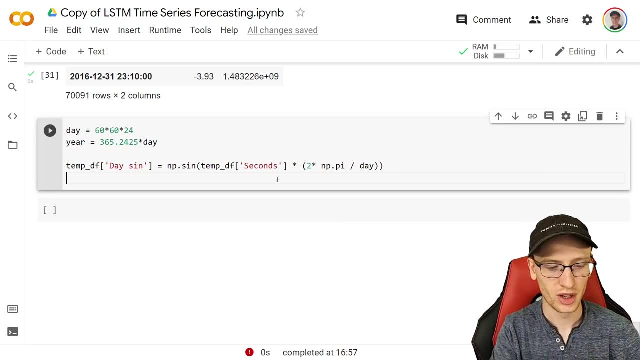 And then divide that by the number of seconds that are in a day, And it turns out that this gives you a nice sign signal. Sorry for the mess up there. I tried to do something off screen and it didn't work, So I'm just going to not do it. 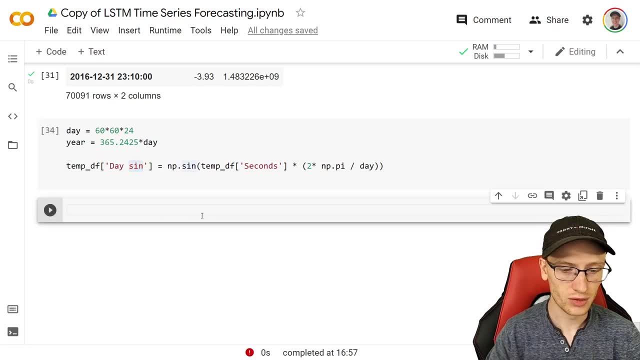 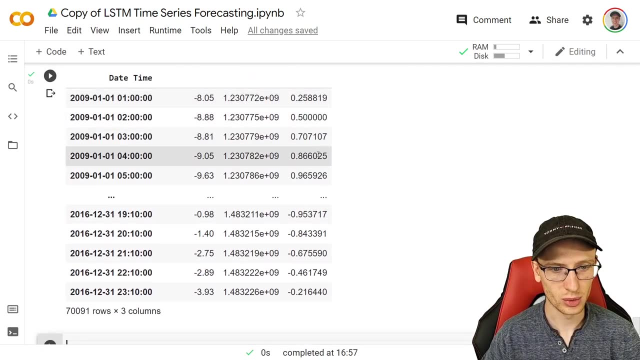 So, anyways, that's our sign, signal for the day And we can look at it if you want. with temp D F, I actually ran that, ran that cell, and we can see here 0.25, 0.5, 0.7, 0.86,, 0.96, and then it would start to go up, and then it would start to go down, and start to go up, and start to go down. 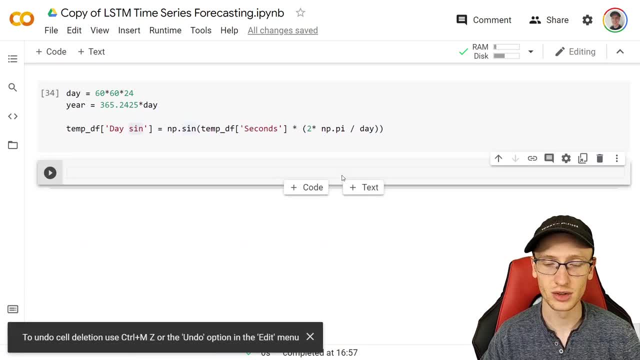 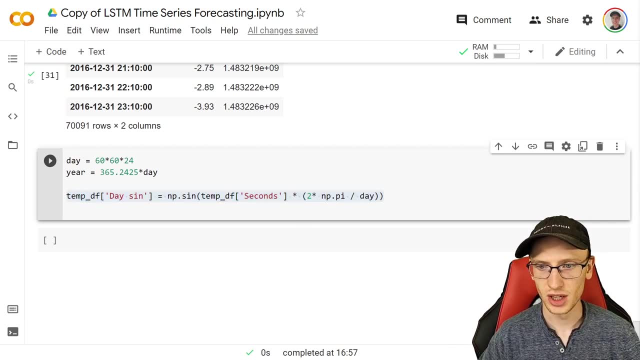 So we turn that into this nice, this nice period signal, the sign signal, And we can do the same for a bunch of different things. So I'm just going to copy- actually, I'm just going to copy the other three in there, because I don't really see a point of writing them out for you- 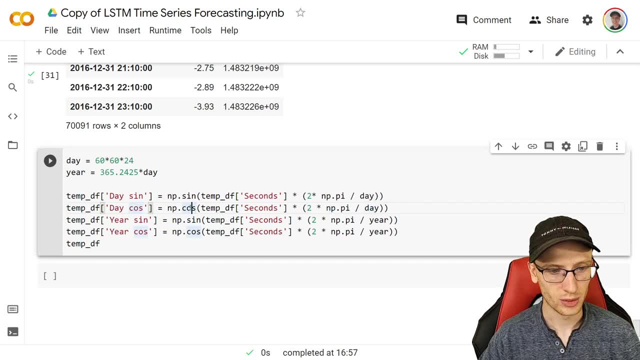 I'll explain it. Day cos is going to be the same, except with cos, and stick with day And year sign is going to be the same, except stick with sign and replace that with year cos, cos, year and year. Okay, 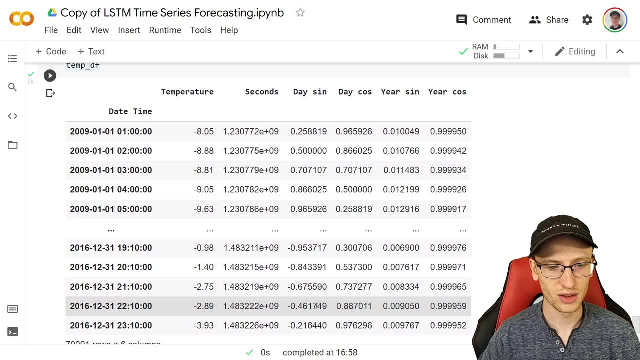 And if you wanted to output the whole data frame there, then here you can see. they're very nice signals. And what's also nice about this is there's not going to be any other pre-processing. We actually didn't have to do any pre-processing before because we were only using one variable. 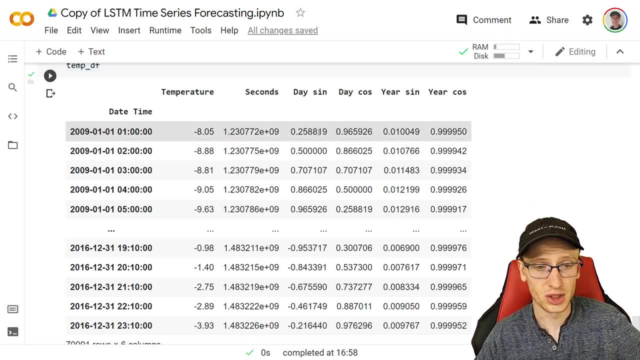 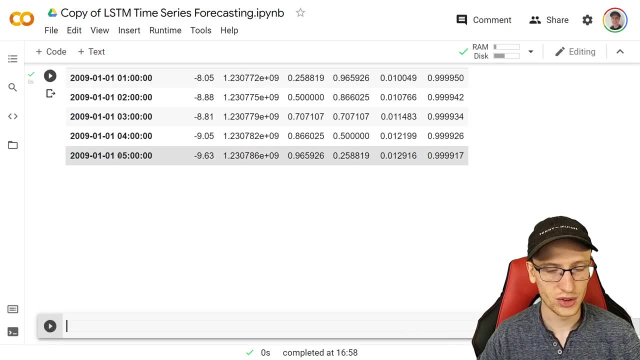 We will have to do this now, But these are already in the type of range that we want. That's going to be. we're going to be very happy with that variable, So I'll stick with that And then just put dot head so we don't have to have the whole thing in the notebook and carry on. 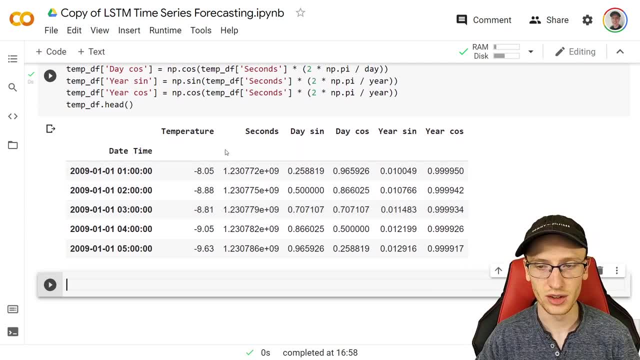 Okay. So now that we have this basically in our new data frame here, we don't really want the seconds column because that's not going to be overly useful to us. You probably could include it in there, except there'd be some weird co-linearity because it's based off of these signals. 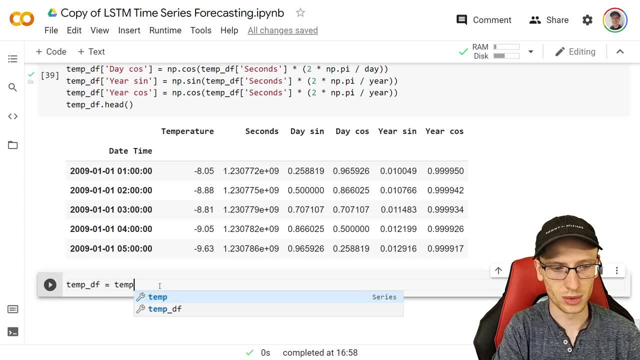 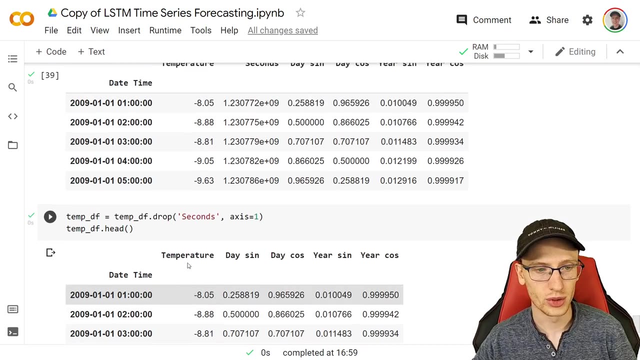 So let's not include that We're going to do. temp df is equal to temp df, dot drop seconds And then axis equals one, And this reminds me after I show this that this is gone. Why actually weren't we happy with just the seconds column in general? 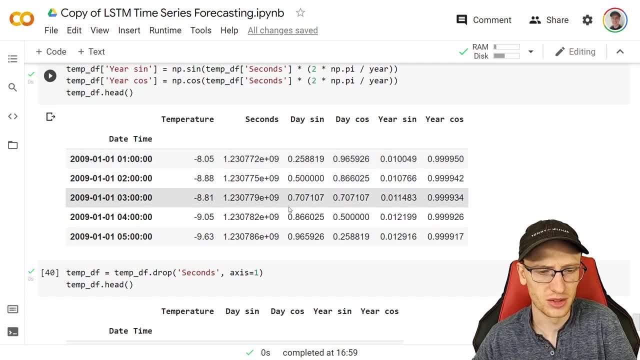 Because this is some positive value. We could have done some pre-processing, like divide it by the max value and then have values between zero and one for each of these. Well, the reason is that there is this period data where, basically, as this time goes on, the temperature is going to go up and down, and up and down, and up and down. 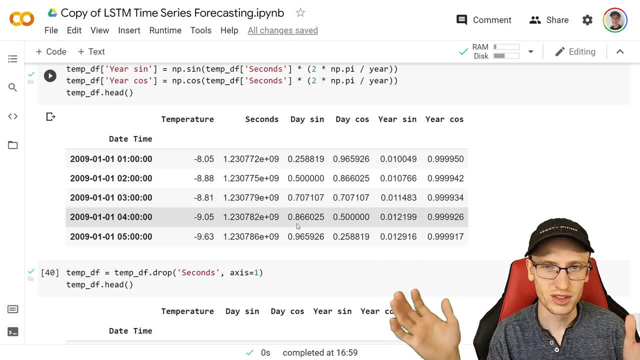 Except this seconds column. This is just an ever increasing value, And so it should really wrap around where, basically, if you have a time, a seconds, that's equivalent to that's very close to December, So say like late December, and you have a seconds amount that equates to, you know, early January the next year. 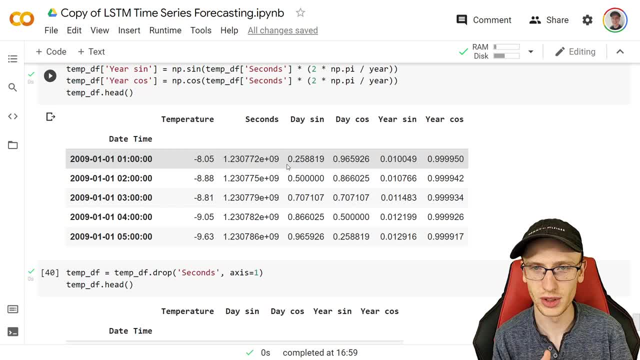 The seconds thing. this doesn't show that, because it just shows the one number is bigger than the other. But really they should have a very similar. They should have a very similar Temperature value and including the fact, more importantly, if we were to increase this three, four years in the future, well, this time in December, should this amount, this value for the column seconds or whatever we're using it, this value should be very close to whatever it is in that December. 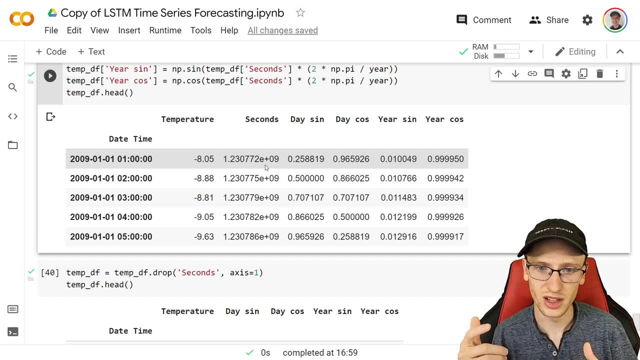 Because the point is that we're reflecting this kind of period data- What time is it in the year, Not how many seconds it is, How many, What time is it in the year or what time is it in the day. So here today, 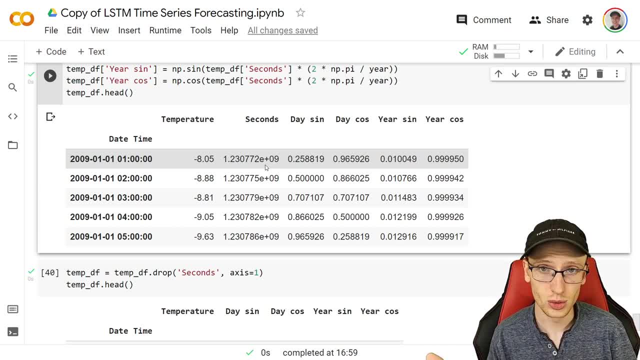 It should be roughly similar to what it is two years in the future at the same time, or tomorrow at the same time. So we have to reflect these values somehow, And so we do that with with this translating seconds into day sign, day coast, year sign and year coast. 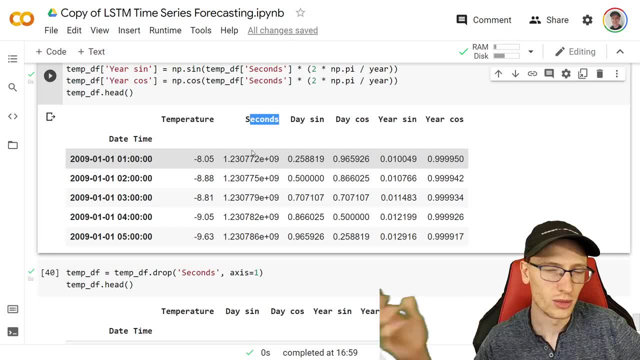 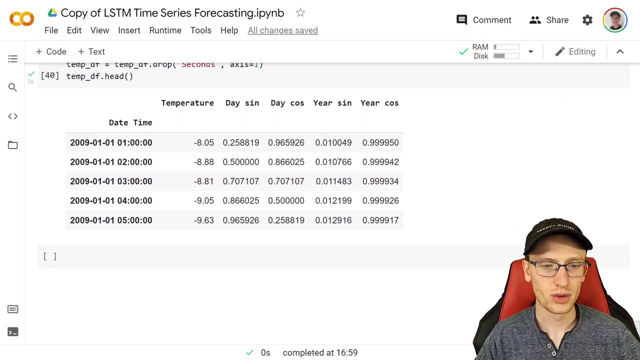 So I hope that makes sense. The intuition is that this should wrap around, not be some ever increasing value here. OK, anyway, so we've got that and let's move on. So the next thing we have to do is change Our, our function that we used to make our window. 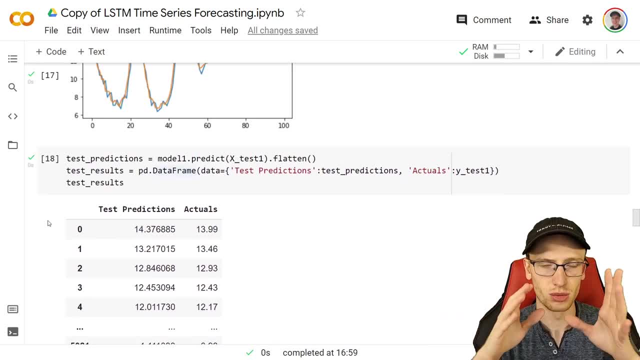 So it made our inputs basically turn it into, you know, these from this whole data frame into here's the five, here's the five and also our labels as well. So we'd have our matrix of five, five, five, five, five and then the whole vector of the corresponding outputs. 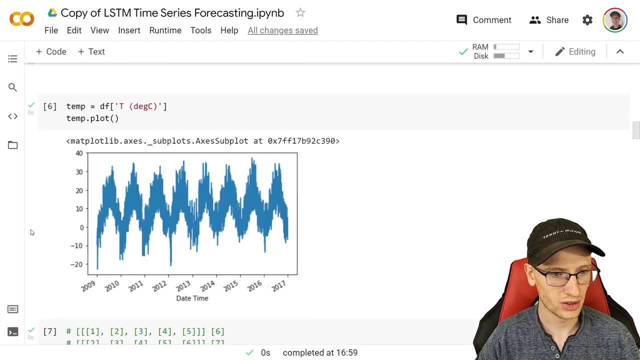 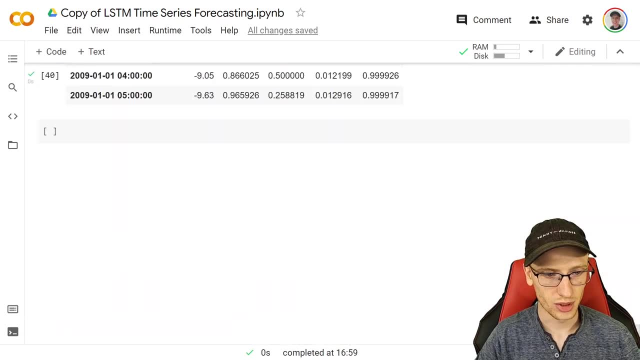 So to make this, make this output or make this input output pairs. we use this thing here and we called it like that And we'll see that soon. But anyways, going all the way down, sorry for the headache, we're going to copy that and this is the idea. 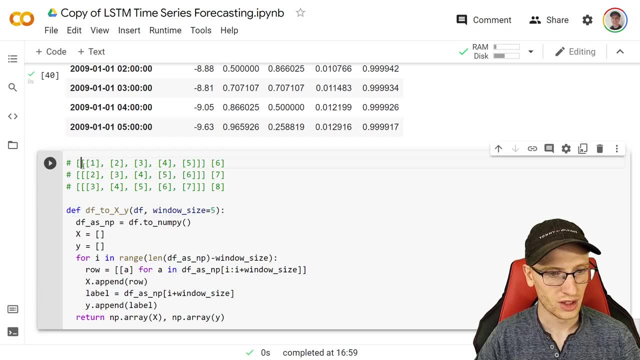 So just to recall, if you don't remember, the point was that each of these rows here, this is one row of information and this is this is the answer. The next temperature we have the temperature at one o'clock, two o'clock, three o'clock, four o'clock and five o'clock. 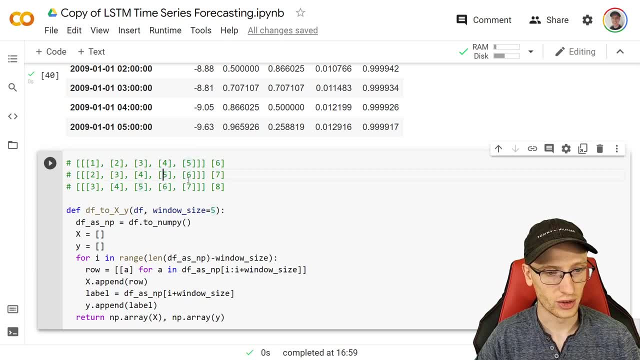 We're going to use that to predict six o'clock, two o'clock, three o'clock, four o'clock, five o'clock, six o'clock. We're going to use that to predict seven o'clock. So this is about making turning the data frame into this function. 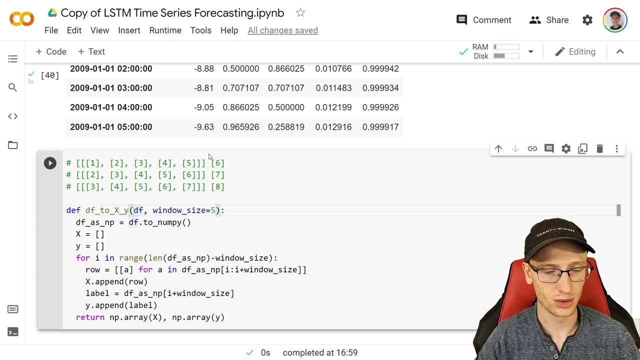 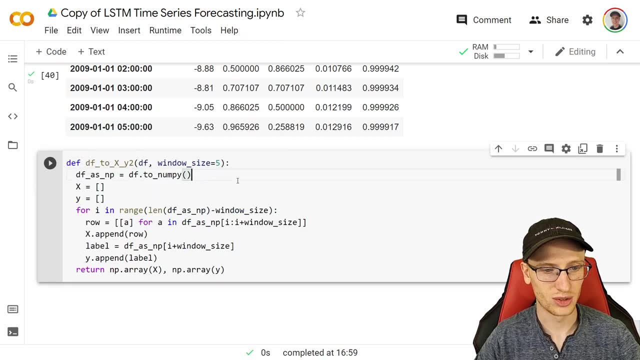 Into this format. That's what this is trying to do. This whole thing is X and this whole thing is Y, So I'm going to get rid of that, since we already have it, And now we're going to call this a DF to X, Y, two just to, and it's just for our next model here, and window size equal to five for sure. 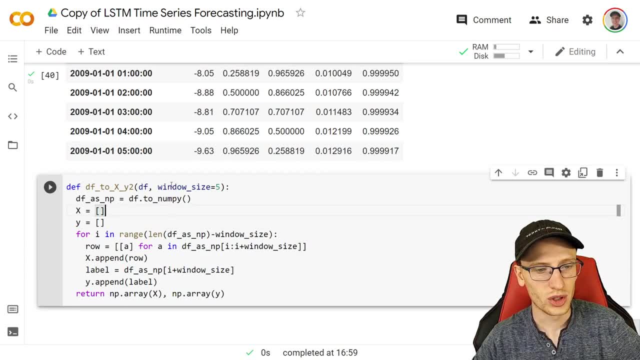 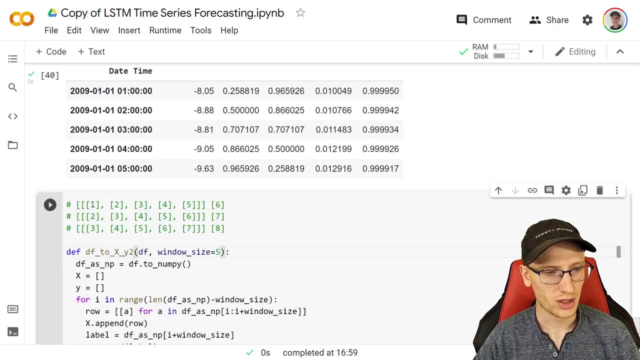 That's. that should be fine as well. Uh, but the difference here is that we are appending, So remember actually. well, I just got rid of it. Yeah, actually I want to keep that for now, because what we're using here is this is really T one. 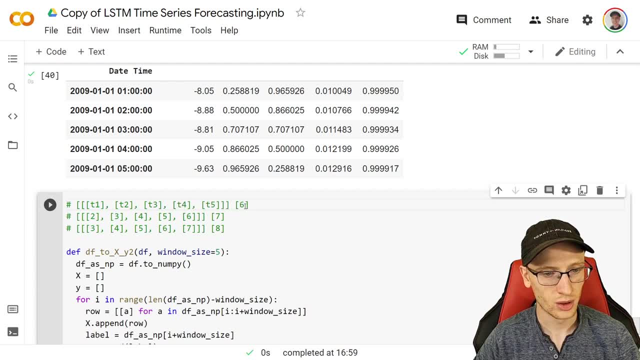 Temperature at one o'clock: T two, T three, T four, T five. We're using that to predict T six and T seven and T eight, or at least we're using this, this, this stuff, to use seven for predict seven and this done to predict eight. 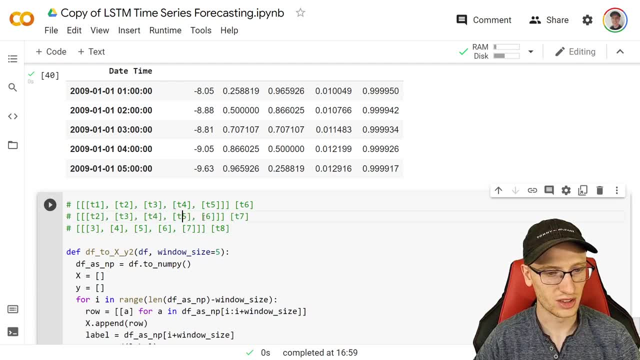 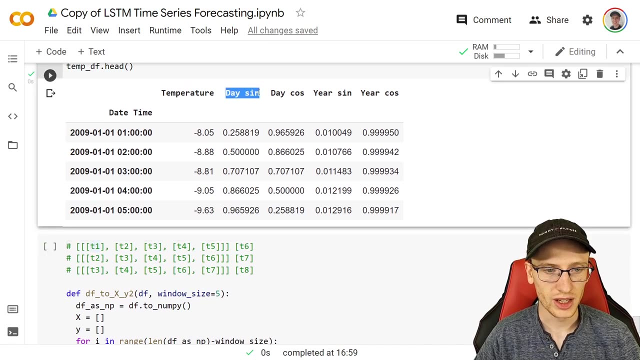 So if this is all temperature data, I'll just add T's here. It's going to be the same same idea, except instead of predicting or instead of using just the temperatures, we're going to be adding these other columns and assume you know they're actually we're going to be adding 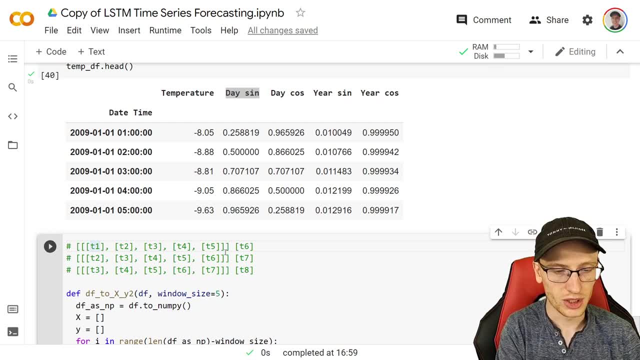 All four of these things, but I'm only going to show you one is: uh, this would be DS for day sign. So this w we're going to want to put this here: D sign at one o'clock and then day sign at two o'clock, and then so on. 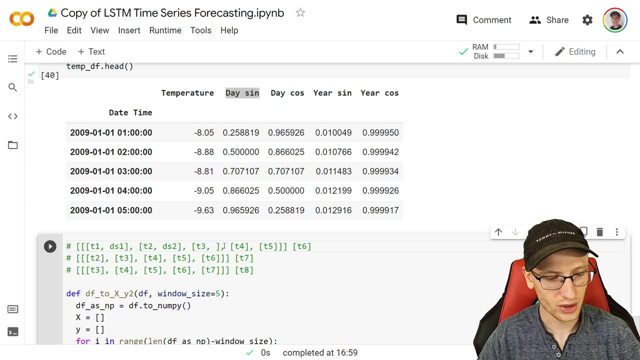 So I'll just copy that in, And I think this is worth the time. skip ahead if you're annoyed by this, Uh, but I think it's worth for beginners to understand really the format of the data here, And once you get a hang for this, then, uh, then you're really good to go. 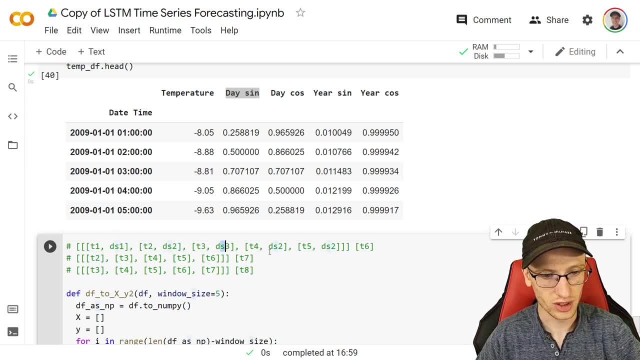 So day sign at one o'clock, They sign at two o'clock, they sign at three o'clock, they sign at four o'clock and they sign at five o'clock. and we're using that. you know you could try to predict these other values, although that's kind of stupid, uh, cause it's time and you know what the time is. but we could use that to predict whatever we want. 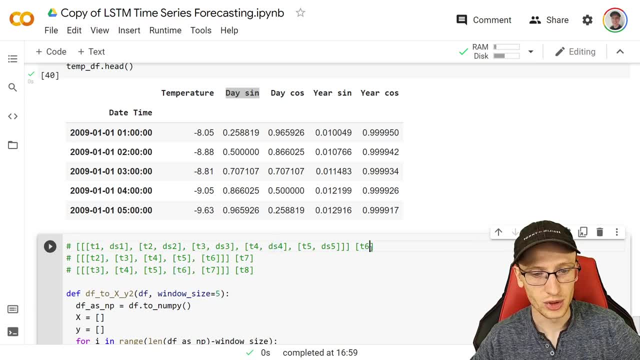 We're only predicting temperature. We're going to use all this stuff to predict that at T six and T seven and T eight. So we're not going to change that. That's what the label is. We're not going to change the label. 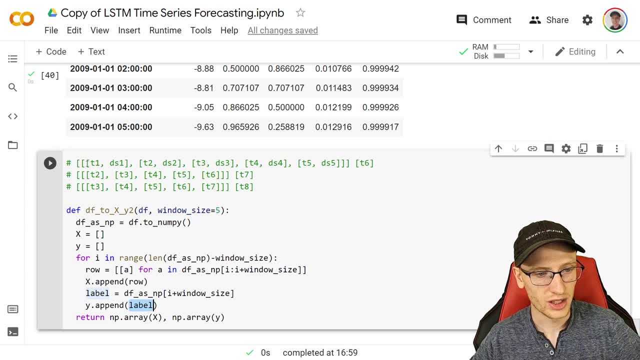 It's going to still be the temperature, but here we want to be adding in this row This whole row of data rather than just the list of the temperature. and here this'll be: this'll be D S two, D S two, and this will be D S three, and so on and so on. 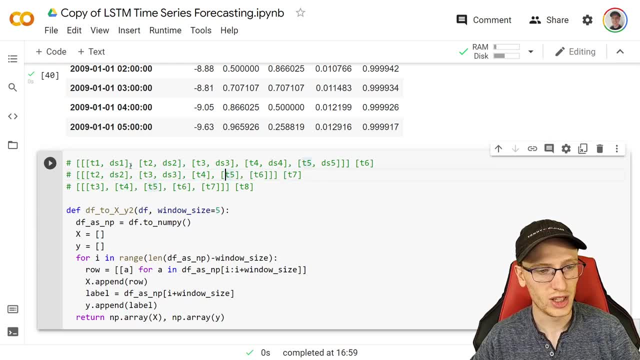 It'll match. It'll always be this number here. So in each of these, uh, basically in each row where you want to have the following type of data, we want it to be a list. So one thing, two things, three thing, four thing, five thing, where each value okay. 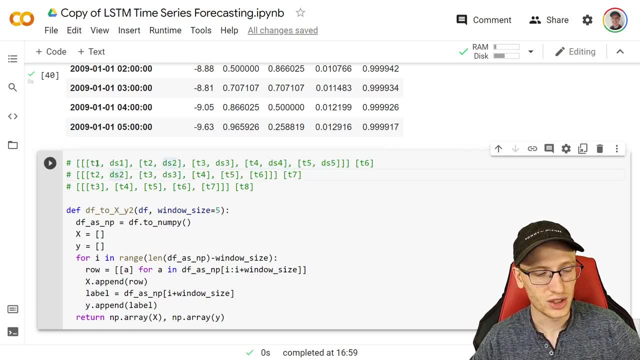 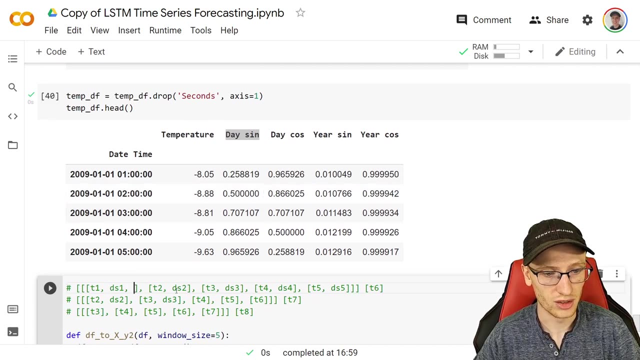 Or each thing in there is a certain time step And each item is itself a list where the first thing is the first variable of interest, The second thing is the second variable of interest that we also have in here. for all of them We would have date D, D, C, one, and here we'd have DC two and here we'd have DC three. 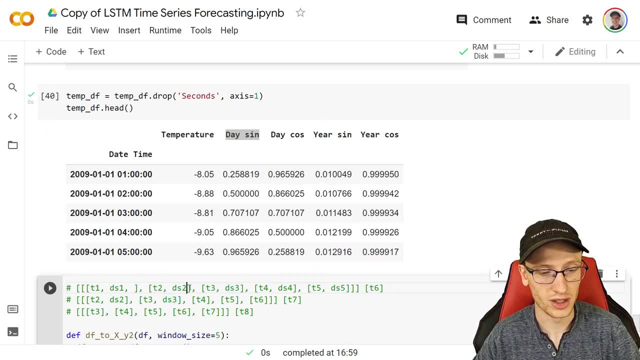 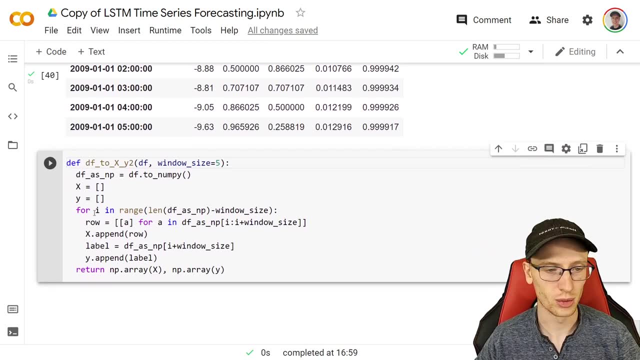 And we'd also have Y S, your sign one, and Y S two. Okay, So we want to make this function and I'll finally get rid of this. Hopefully that made sense. If that was boring, I hope you skipped through it, Okay. 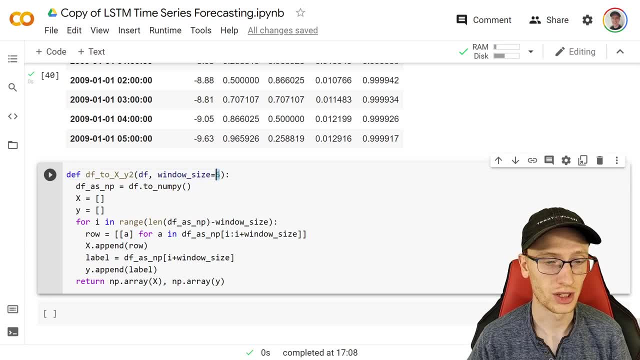 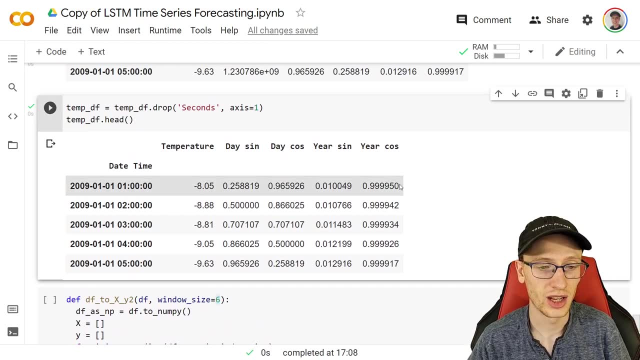 Let's write this function. So, if you recall what we were doing- and I changed the window size here quickly to six because otherwise we would have a five, one, two, three, four, five variables and a window size is five as well- 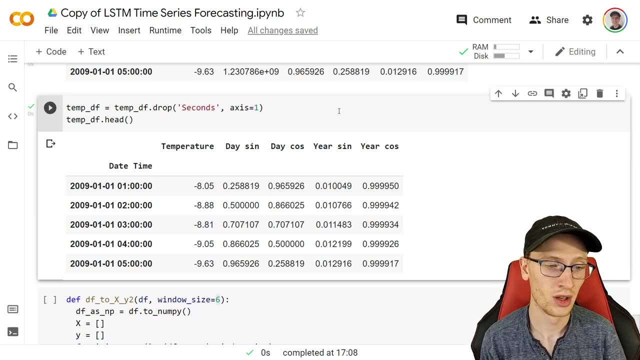 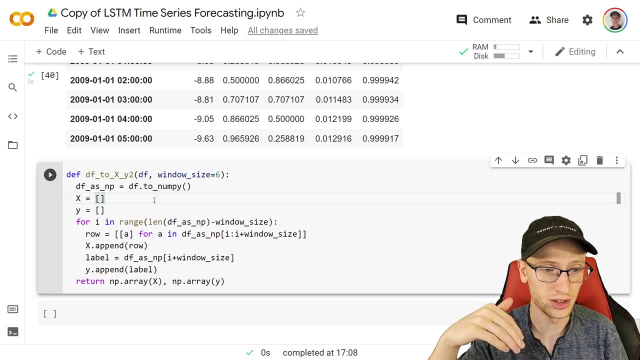 I want those to be different values because I want to see how the shape turns out to be Uh, and so we're going to be building this thing up: X and Y more. X itself is going to be. its shape will be the number of training examples by the number of time steps that we're using. 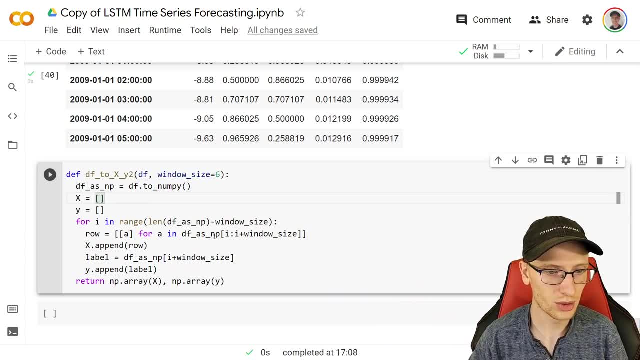 Times D: Number of variables that we're using. So, uh, if we recall what we were doing for the other function we have for I in range, uh, we go. basically we iterate through the data frame with an index. 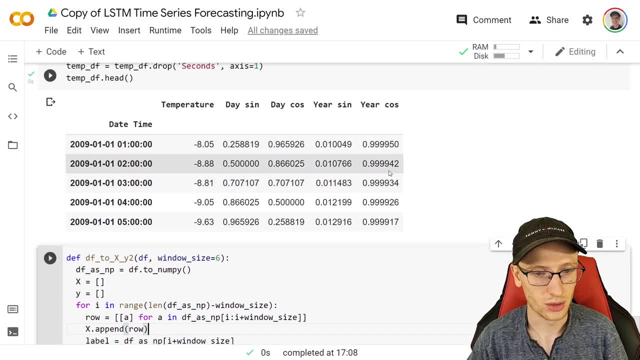 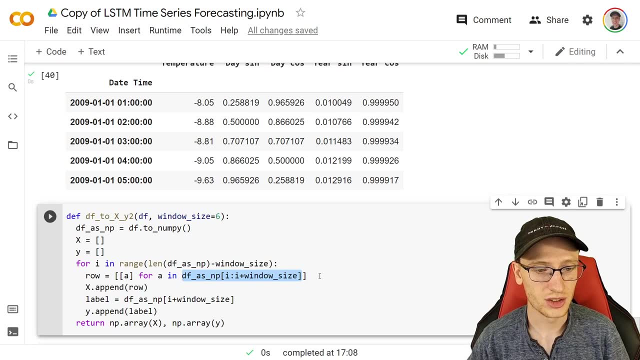 And so we go through once, and then two, and then three, and then four, uh, and then each of those. in each of those, we actually grabbed this thing: DFS NumPy I, until I plus window size. So what that does is, wherever we happen to be, wherever our starting point is, say, our starting point happened to be here. 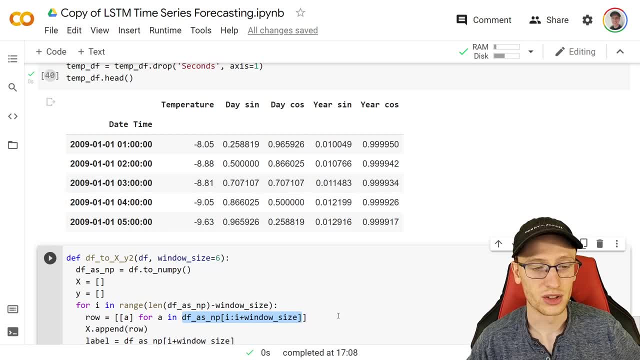 I was a zero, We would grab The next, uh, whatever- piece of information, the next window size piece of information we'd left be left with, basically this matrix in here. That would be this whole thing, would be, um, some, some cut of the matrix. 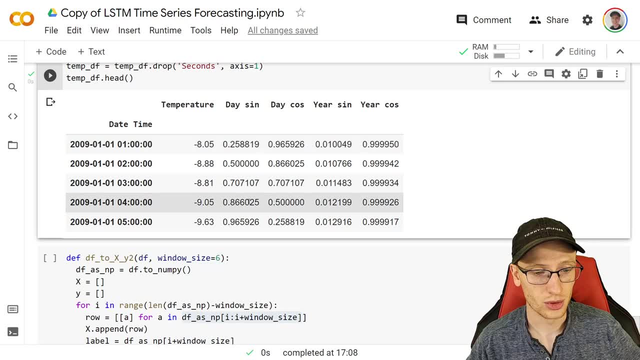 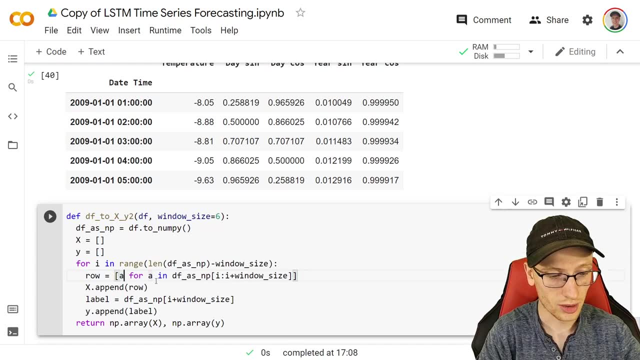 And what it is is that each of the rows is the time steps in order, And so what we can do, it turns out that we can actually just do, uh, if we replace this with R- and it doesn't matter what variable name you use, but it's R, because each of these are a row of information. 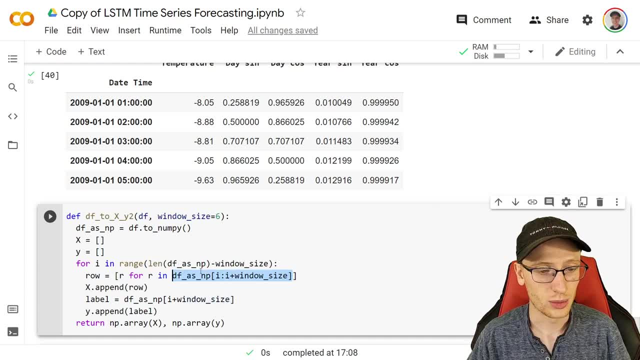 If we just do, If we just grab this thing, that matrix, that split of the matrix that we want, and then we say, okay, row is our, the whole row for our information, And so our row is not going to be made up of just values. 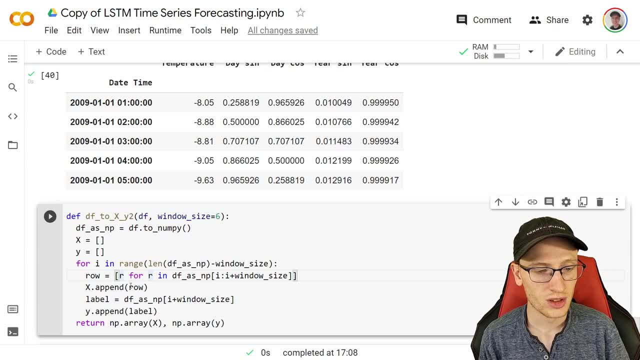 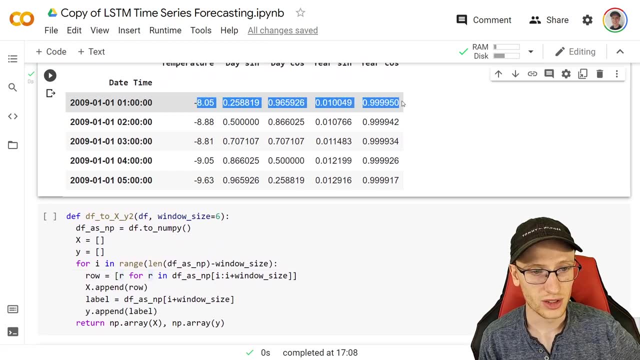 It's going to be made up of lists of values, And so here, this itself is going to be a list, because it'll be, it'll be one of full of these things. Okay, So it's basically R is going to be all of that. 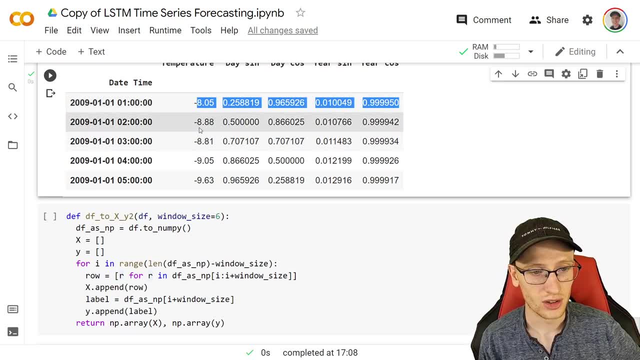 And then again, if you, since this is a four loop in here, The next R is going to be all of that, and then all of that, and then all of that, and then all of that, and so on. So basically it makes it this, uh, this whole thing, this list of lists here, where each of the inner lists is going to be going to be one of these. 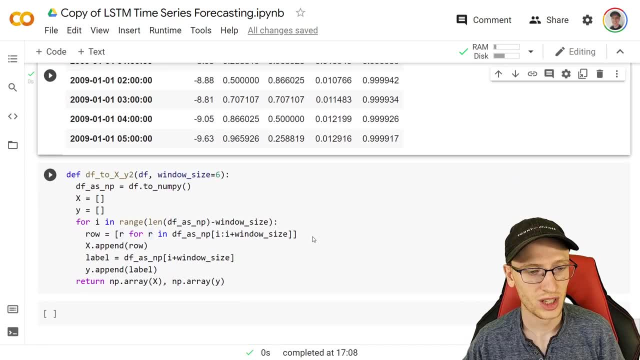 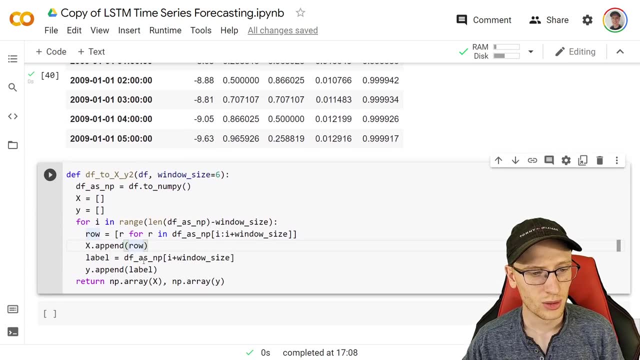 Okay, A little bit confusing And that's why I try to take this really slow and seriously. So you get how the input is made. We're going to each time append this row and then label is going to. well, DF is NumPy I plus window size. 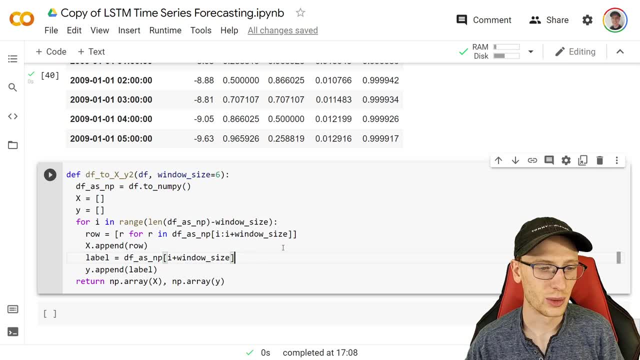 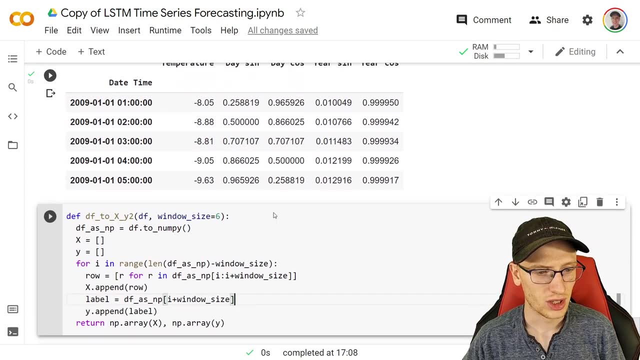 It's going to be the next, Uh, the corresponding output, And so well, uh, if this is an, if this is a, a data frame, here, this is a matrix. What that's going to be doing is actually grabbing, uh, making it the row, the whole row itself. 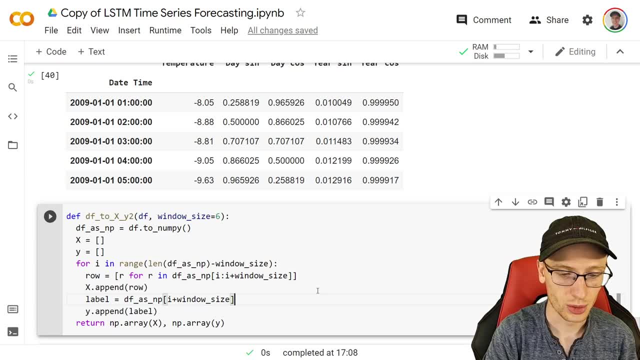 So what we need to do is translate that into the variable of interest that we want, And remember this: if we're wanting to forecast multiple variables, we could actually make this multiple piece of information, as we will later, But we want to make that sub zero so that we append the right. 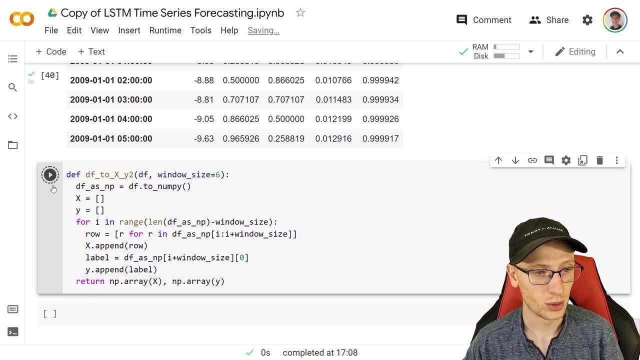 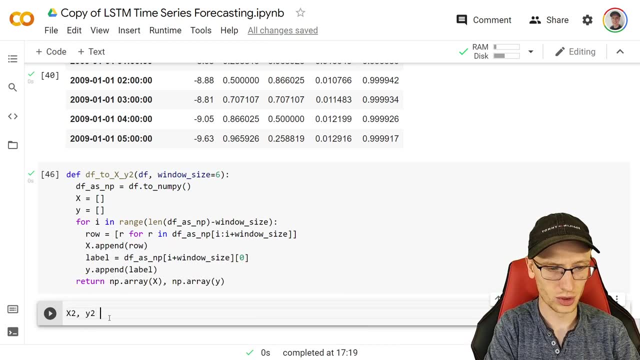 Label on there, just just the temperature value. So if we do this, we run that and we grab um. actually, I'll just write it out for you, It's pretty easy: X two, Y two. we're just doing twos because, uh, mapping changing, switching with the twos from before, they're stick sticking with the twos from before. 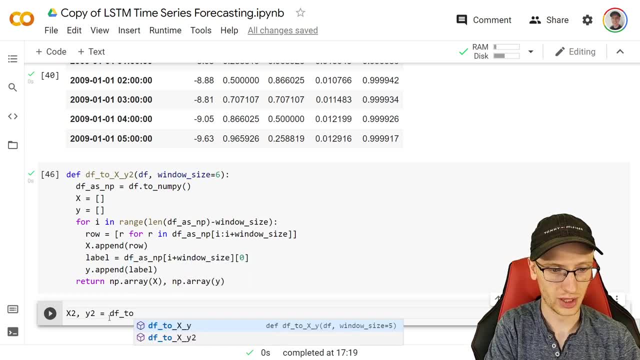 Sorry about that. Uh X two, Y two is going to be DF, two X Y two and that will be. we're going to pass in the DF which is, I believe, temp. uh yep, Temp, DF, temp, DF. 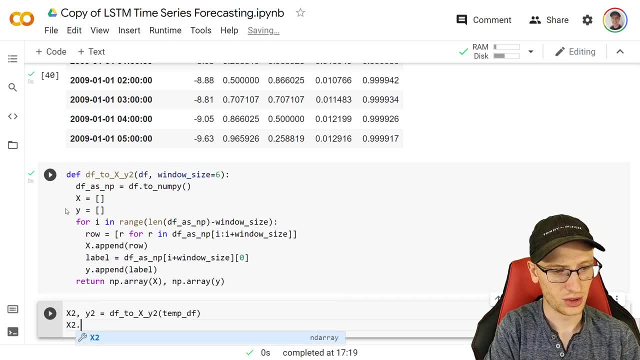 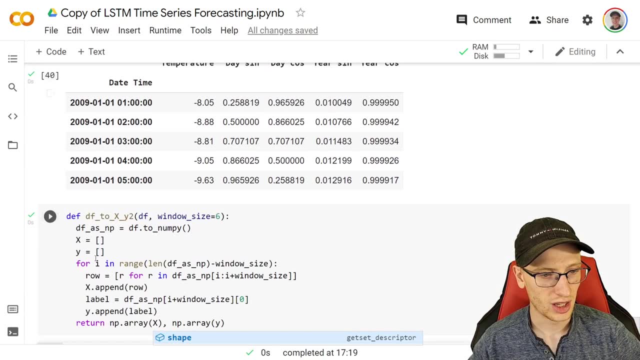 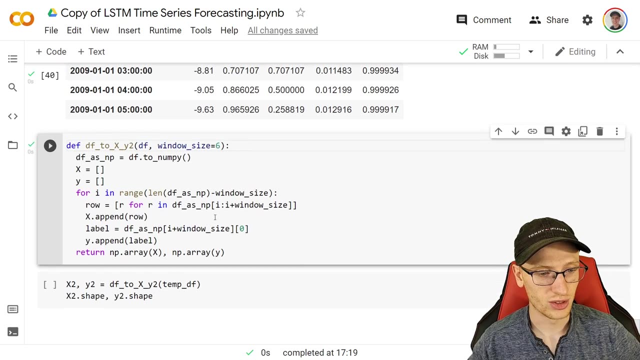 And the window size is six is totally fine. And then if we ask X two dot shape, Y two dot shape, we should see: well, however many training examples. And for X two, we should have however many training examples by six, by five, because we're using six time steps and we're using five variables and Y two dot shape. 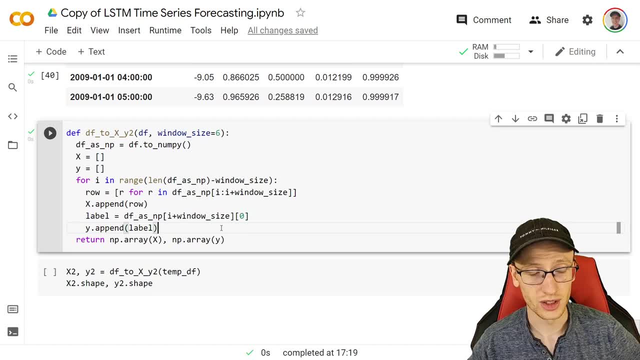 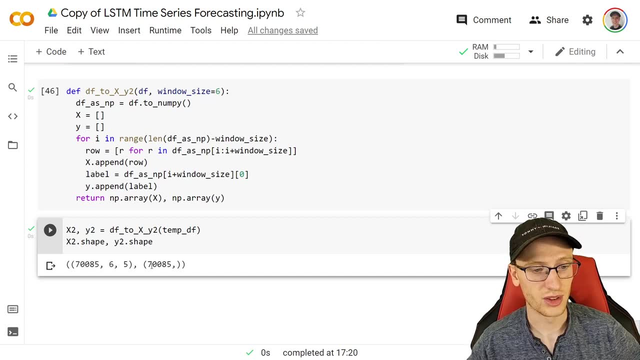 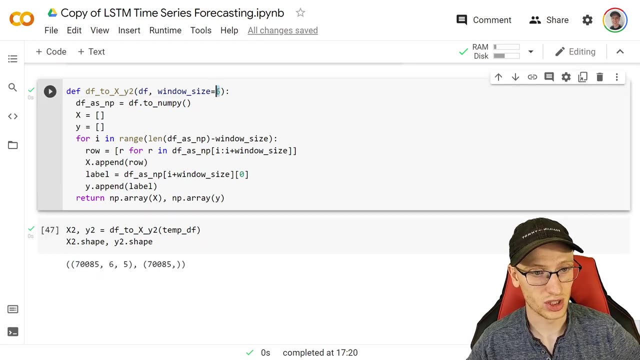 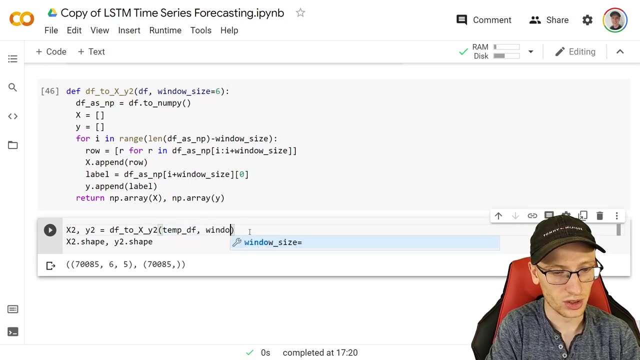 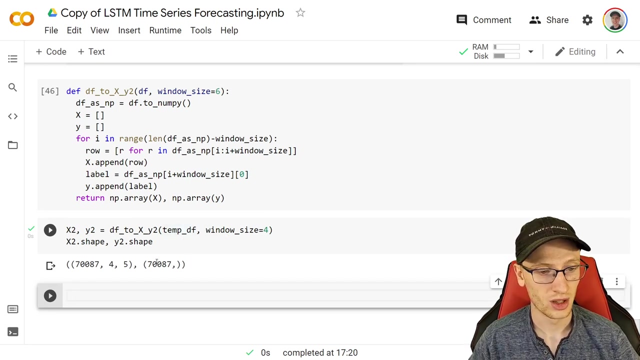 Since we're just depending a value- it should be just the number of training examples- is is the value that we have. So here, X, two dot shape, Y, two dot shape, 70,085.. Again, just to make sure you know: number of training examples, the number of time steps that we're using. so to switch that to four, if you want to switch it to six after um, actually there's no reason to switch it in there, um, here I'll just specify that the window size is four and here now it's, we're using four steps to predict the next information, the next value, uh, and so we changed the training number of examples a little bit. 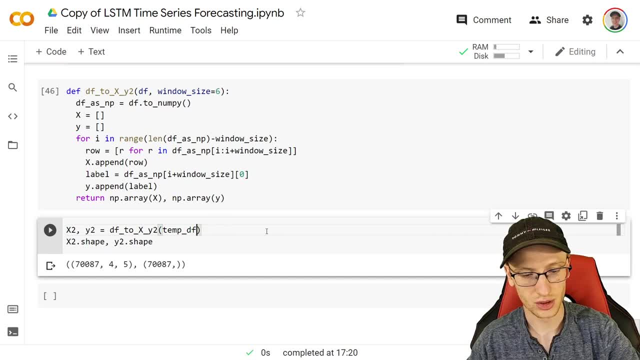 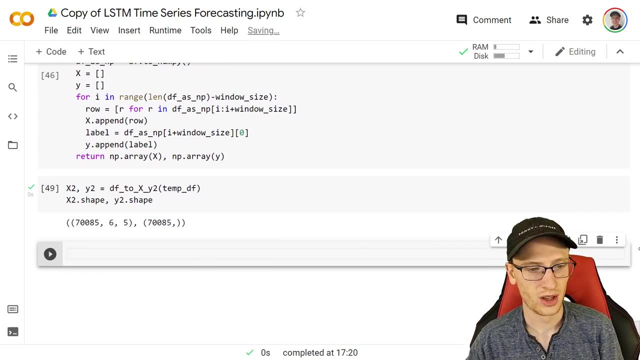 Okay, I'm going to stick with that with six and just, uh, actually Remove that. So there there is our matrix of inputs- I calling it a matrix, It's kind of weird, That's really a tensor- and um- and our output as well. 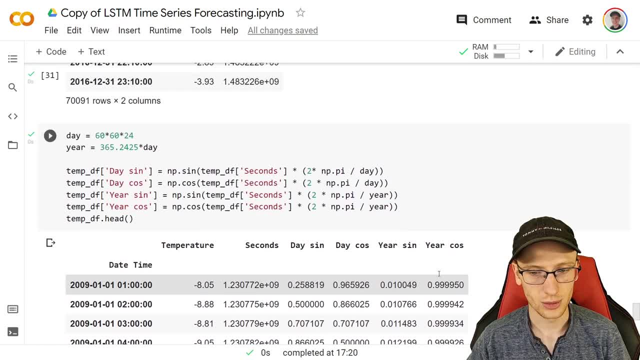 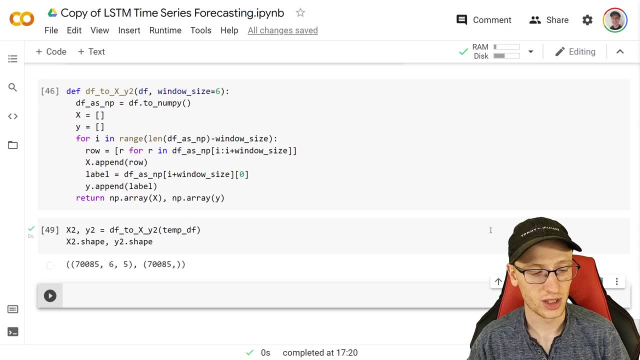 So, now that we have that, we are going to, uh, really just copy the exact same thing that we have way above and, to not give you the headache, I I'll just copy it itself. We're going to be splitting into train test and validation sets. 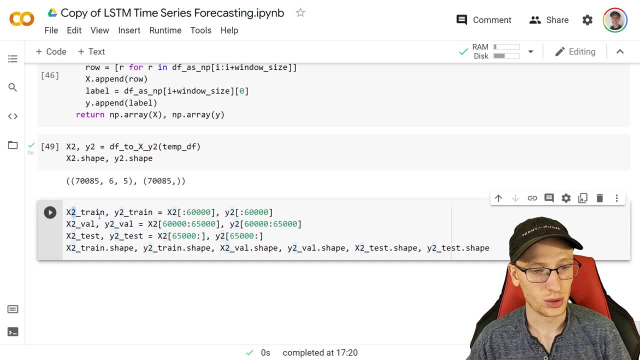 And I'll remind you how that's being done. Uh, we're also calling these with twos, So we're just saying X two train is going to be, uh, this thing, X two up until six. So we're going to be doing this in order where we have trained as chronologically in order, we're training on this, and then validation is in the future and then test set is even in the future, like after that. uh, and there's a reasoning for that. uh, and that reasoning is because you know, in, in practice, when we actually go to use this stuff, we don't have data in the future. 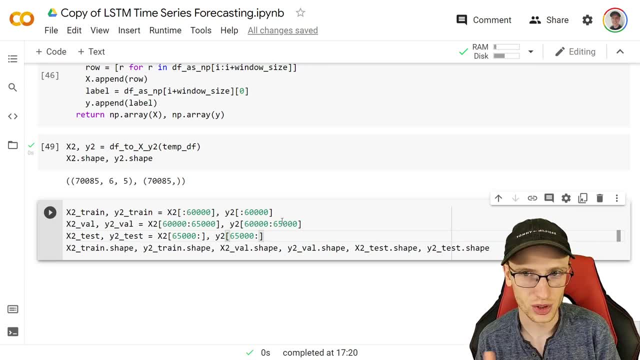 So we want our model to be able to predict- you know, you know- future data better than it can predict past data. We don't really care about that Very much. So anyways, X two train is X two up until 60,000, the first 60,000 rows, uh, Y two trains, the first 60,000 information Val is going to be 60, 60,000, 65,000, uh, same for the same for input and output, and test is going to be just uh, the rest after this point and the rest, uh after this point for X and Y. 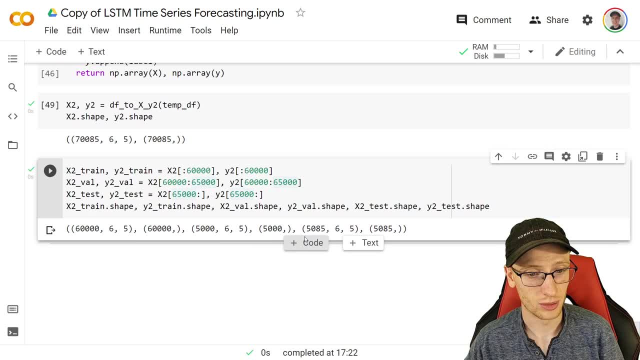 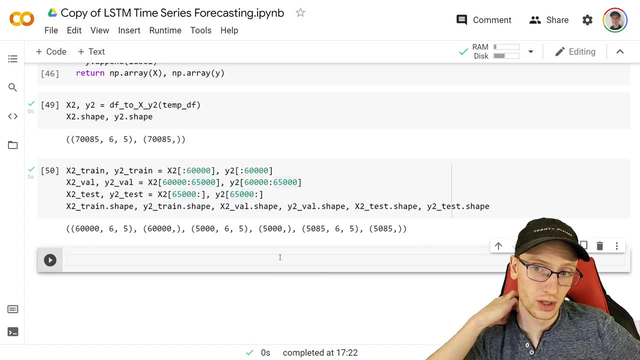 Okay, And if we see the shapes there, then, uh, we should see, uh, pretty much everything match, or well, yeah, everything match. Okay, So now, uh, we have, We have to do something a little bit uh, tricky and annoying. 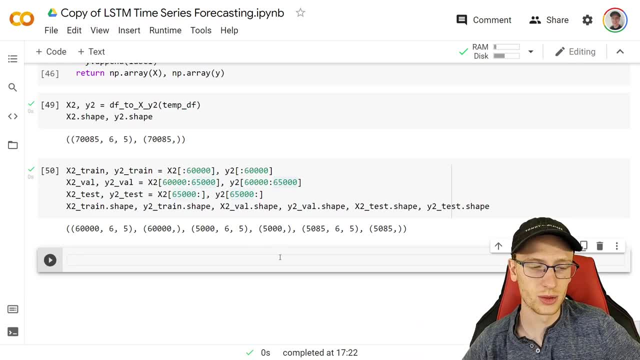 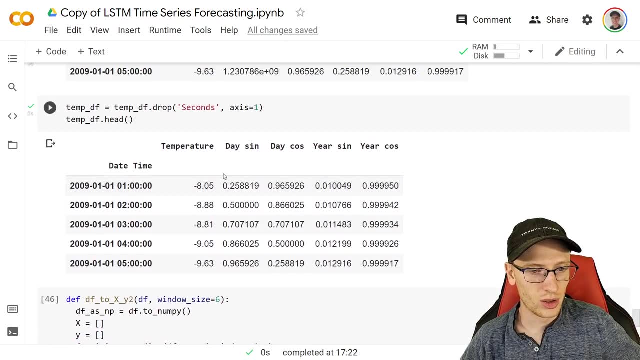 It's. it's mostly just the syntax looks kind of weird, since we're doing with tensors. but uh, hopefully you'll be able to picture and I'll try to explain. it is uh, pre-processing for this type of data. So, uh, you'll notice that these are on the scale of, uh, you know, temperature. it's in Celsius, Celsius. 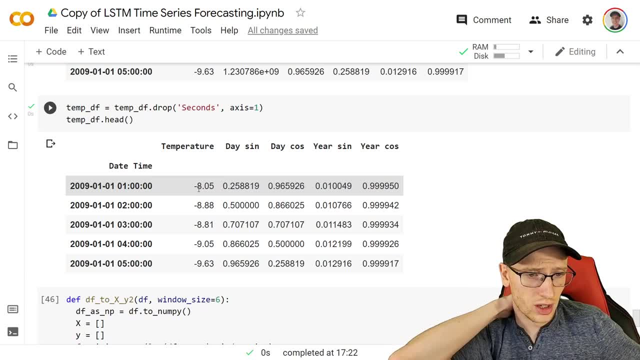 It's going, uh, you know, max like negative 40 or negative 30,, uh, up until like 30,, 40,, 50 or something like that, Uh, but that's still a much different scale than all of these other values. 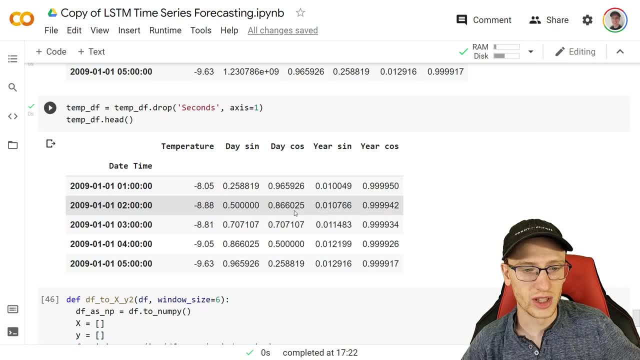 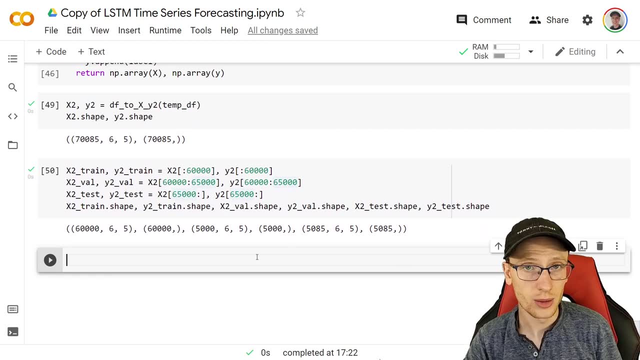 So we have to bring this temperature onto the same type A scale, like between negative three and three or so of uh, of these values. So how do we do that? Um, we want to apply the same exact function, So with the same numbers, doing the exact same thing, uh, to to whether it's the training test, the, the validation set of the test set. 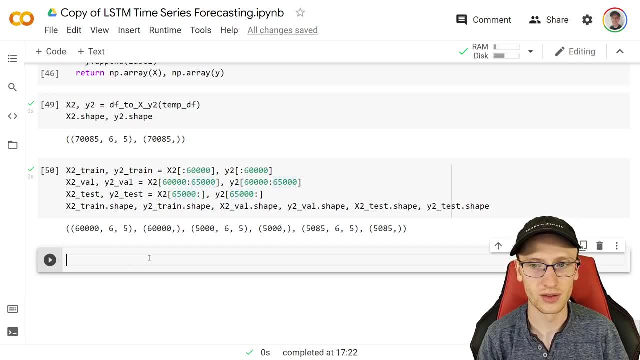 And so what we're going to use, uh, to make the function, is the training set information. So we'll actually gather and we're going to do just what's called- um, I always get them confused. Uh, it should be standardization, which is no, I forget which one it is. 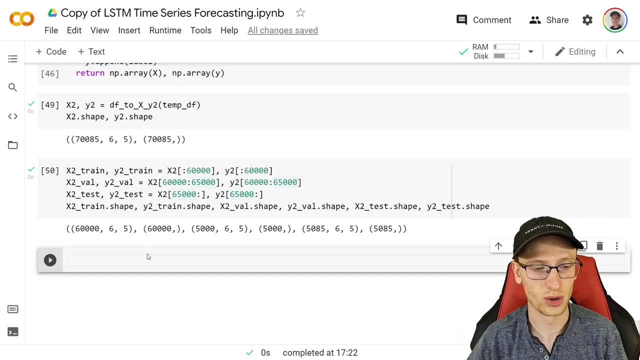 Honestly, Uh, the one where it makes a normal curve, whether it's standardization or normalization, Um, and I think it, yeah, it's standardization, um, because it's making a standard, normal distribution, and yeah, So for that we need the training set mean and the training uh, uh, set standard deviation. 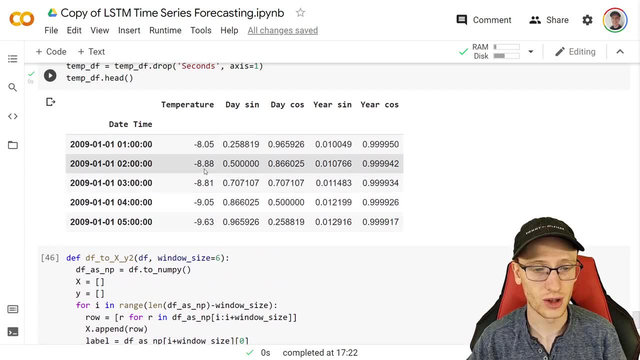 And that's going to be just for the temperature, because we only need to pre-process that column. Um, we'll actually need to do it when we use other variables that are on different scales. we'll need to do it for those as well. 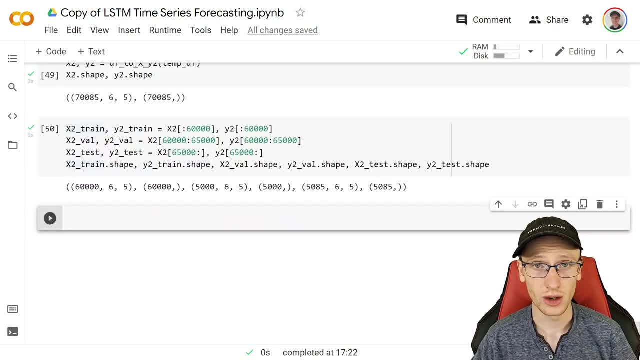 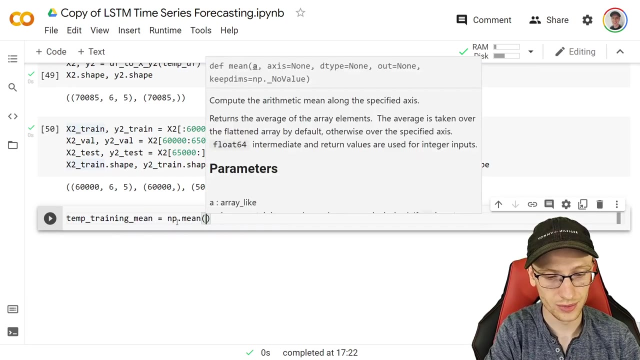 But for this example it's just I'm going to be processing the temperature. Okay, Now I want to do this through the numpy way, So we're going to be getting the mean as well as the standard deviation of temp. So temp is train, uh, temp is temperature. temp training training me is equal to the numpy dot mean of X, two X, two train. 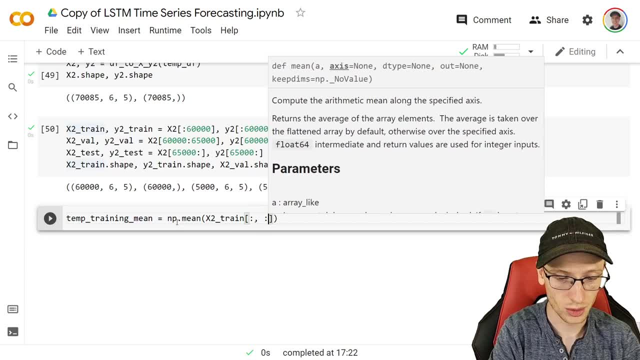 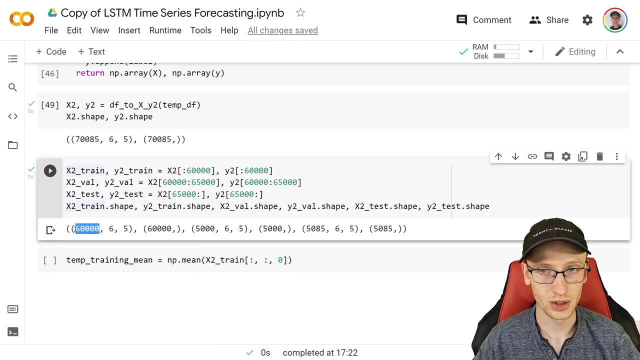 And then I'll just write it and explain: after colon, colon zero. So try not to get too bogged down in this. I know it looks a little bit weird. most likely, but remember, the first dimension is going to be The number of examples in this. we want it to be made up of all of them. 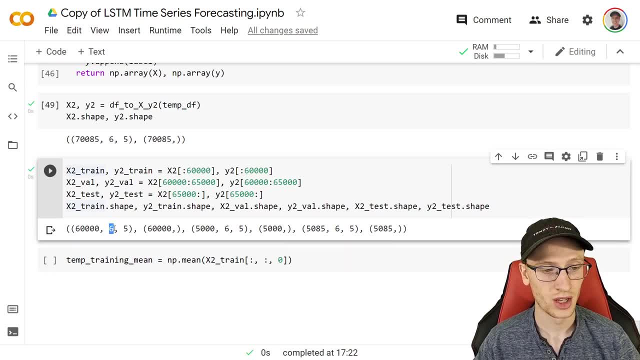 So I chose colon. The next one is the time steps And we actually we want all of the time steps because you know, we want the first hour and the second hour and the third hour and the fourth hour, fourth hour, And then of those spots we have five. and those are the five variables. which variable that we want? 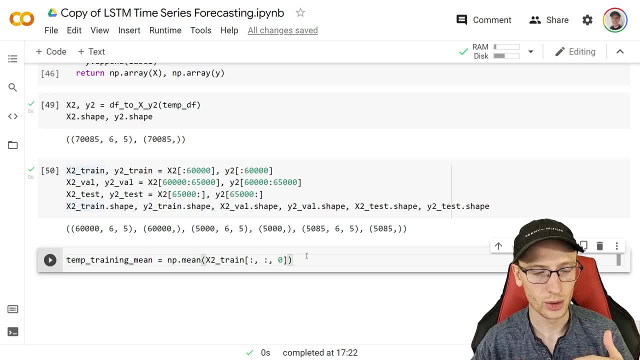 We just want temperature, And I know it's a little bit weird, but if you really think about it, this will be all of the training, uh, the temperature values that are in this. this whole thing Is all of the values, the, the temperature values that are in the training set, and we get the mean of those and that's what we want for making our pre-processing function. 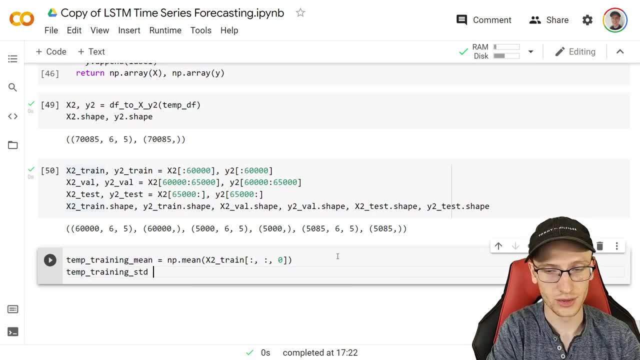 And we can do temp training. temp training, standard deviation is equal to numpy dot STD of X, two X two train. It's going to be exactly the same thing. It's just the standard deviation of the same thing: X, two train, colon, colon, zero. 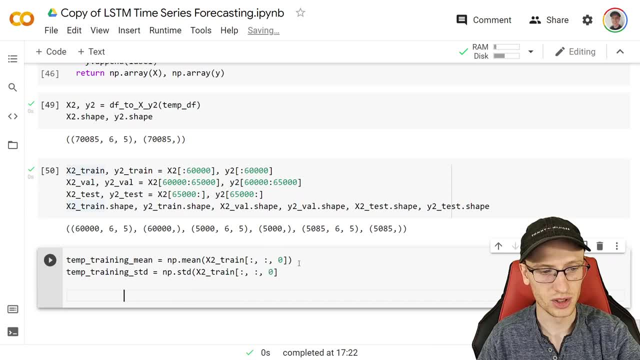 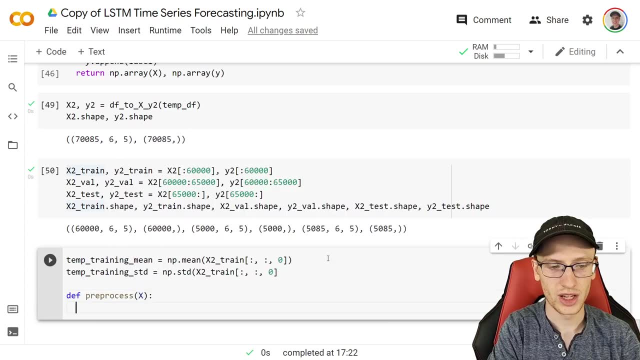 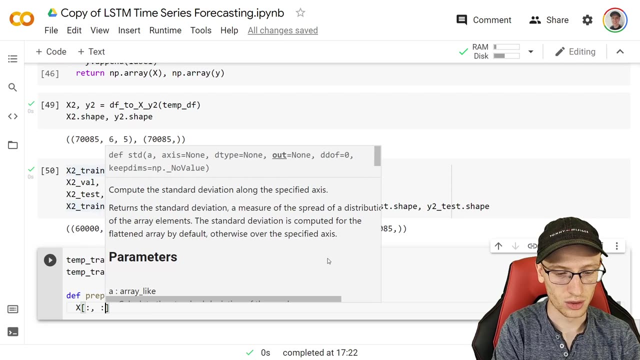 Okay, And now we can make our pre-process function based off of these values, And so we're going to define pre pre-process of X. So just any matrix, whether it's training test or validation. uh, we're going to make that so that X, colon, colon zero. 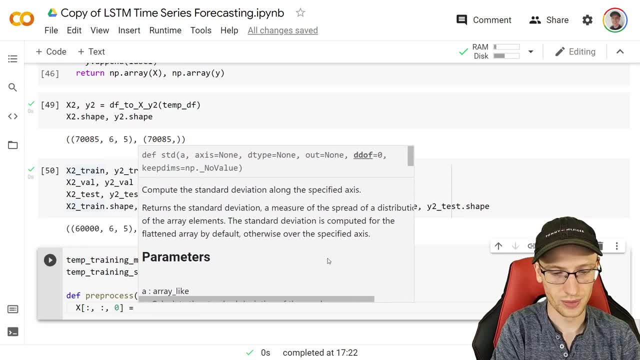 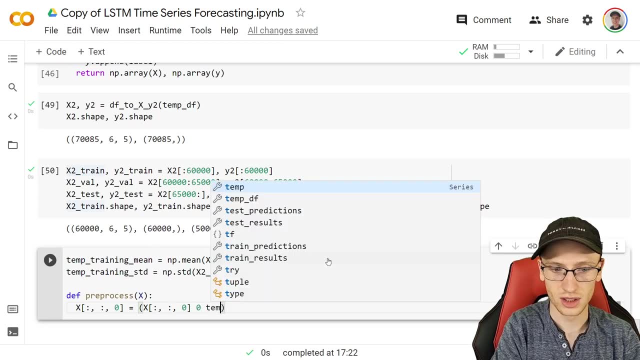 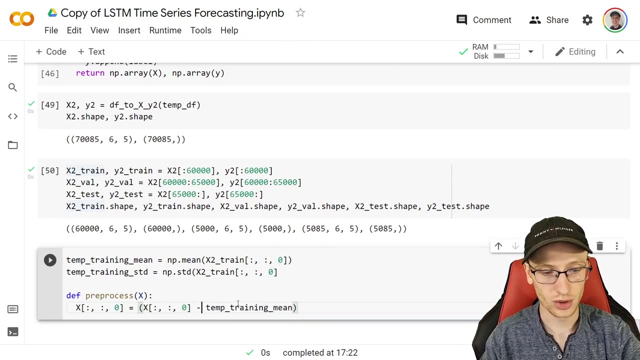 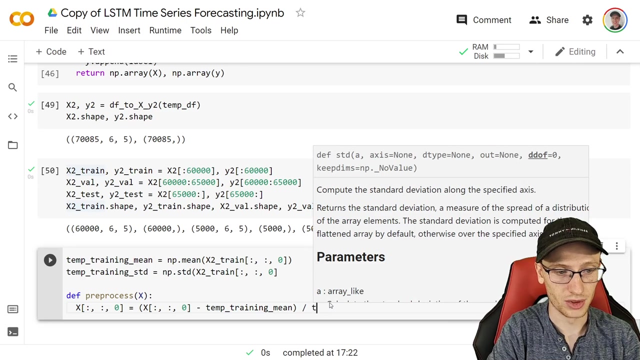 So we're going to set all of those values equal to itself itself, minus the temp training mean that we calculated. So this is dividing or sorry, that's not a minus, That's a zero. Um, so first we're going to take all of our values and we're going to subtract the mean, and then we're going to divide it by the standard deviation: temp training: temp training- sorry, STD. 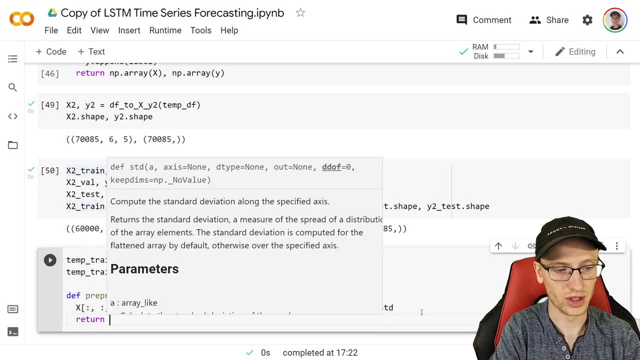 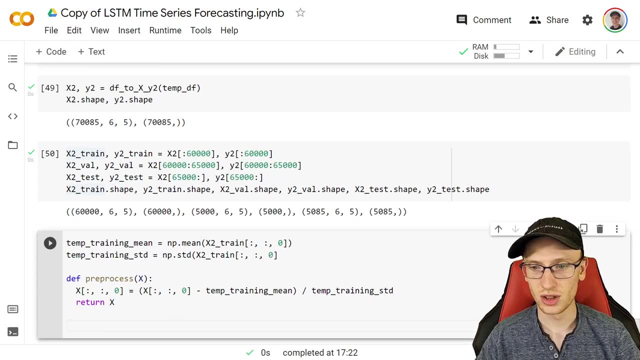 And that's how you, that's how you would do that, And then, if you want, you can return X here, but it is actually changing the thing that you've you passed in fundamentally Okay. So that is our pre-processing, and now we can just go ahead and do this for each of our variables. 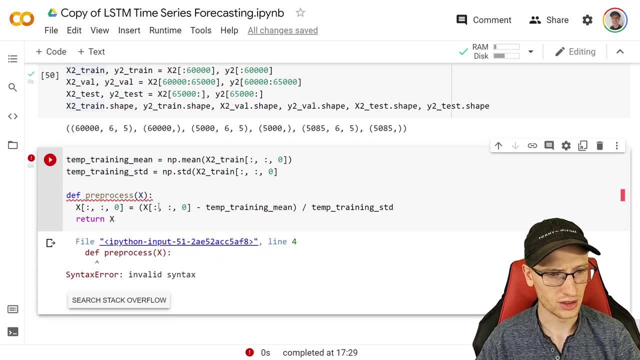 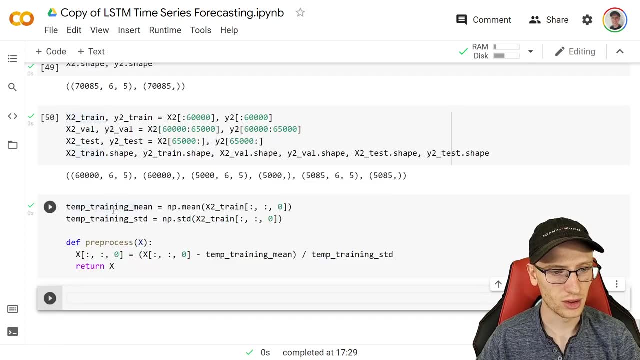 All right, Sorry, Uh, what did I mess up there? Invalid syntax- to find that, um, oh, I'd missed the bracket there. Okay, Uh, so yeah, that's the, that's the mean, that's the standard deviation. 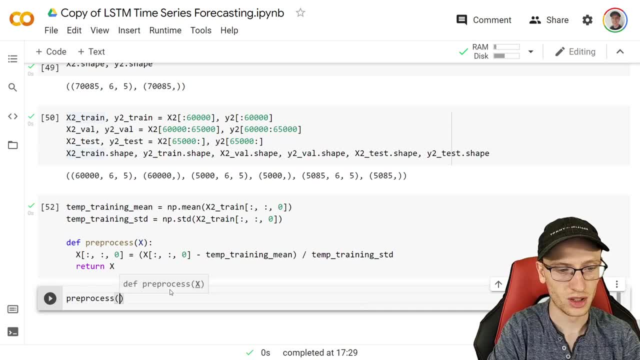 That's how we make a pre-process function. We can just call pre-process on X2, X2 train, pre-process on X2, X2 val and pre-process on X2, on X2 train. I think I said the wrong thing there. 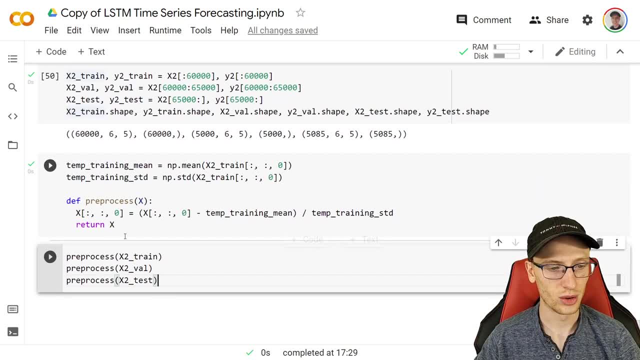 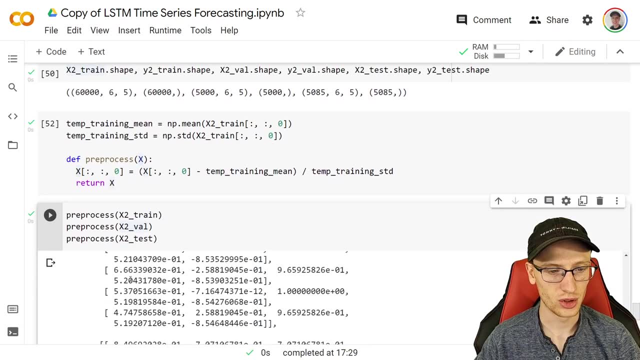 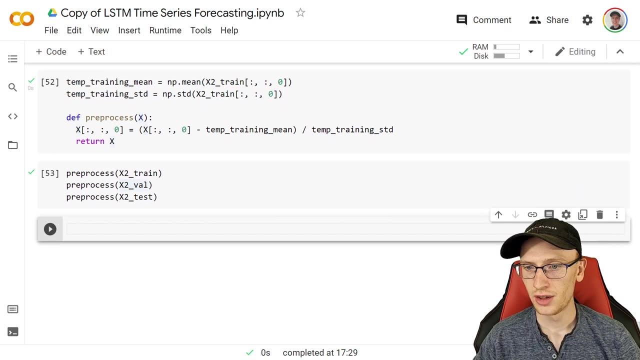 I am not sure, Um, to train val and test, and note that, remember, because I did it, I wrote it like this and even though we're returning X and we're not using it, Um, this is totally fine. So we do that and we can see that. uh, that's our information right there and it looks a little bit weird in that form, but I promise you that we'll be right now. 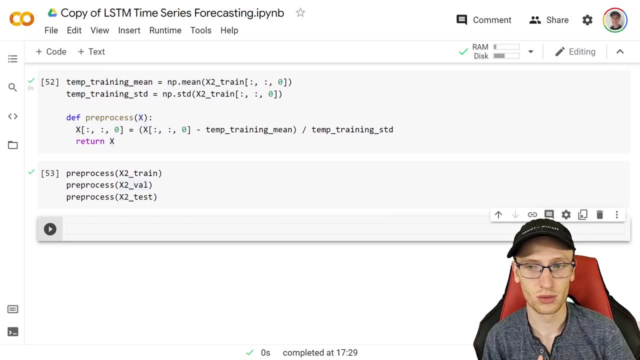 Okay, So we're going to make a model which, uh, which is really the exact same thing as above, uh, the the LSTM model, And I'm just going to copy it in for you and show the difference. Okay. 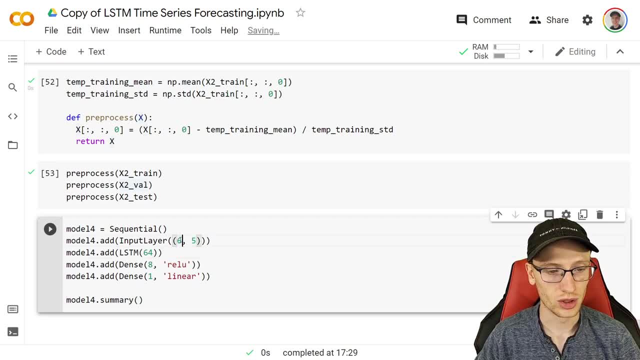 the only difference is going to be the input layer. We're going to have 6 instead of 5.. This used to be 5 and 1, but now we're going to change this to 6 and 5 because we have 6 time steps and 5 variables. 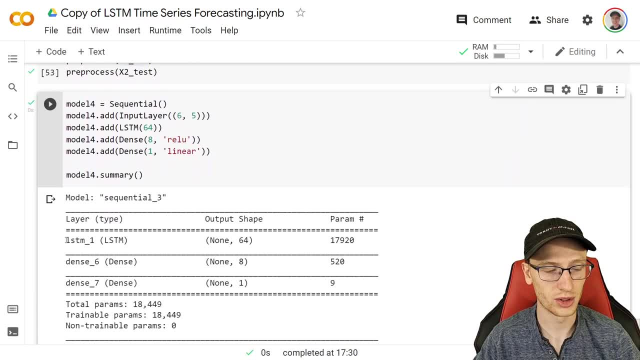 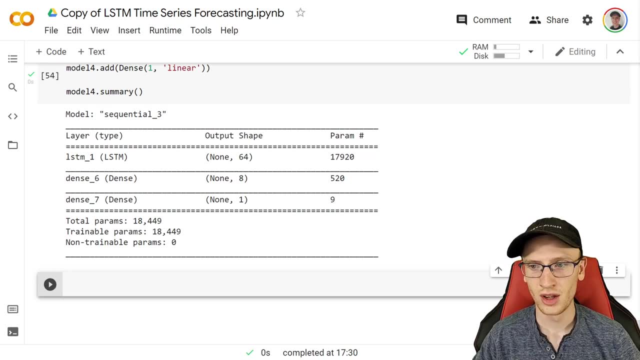 of interest And this happens to work just fine with our input, and I don't like how it's calling it 3 when we're calling it 4, but if we really wanted to change that, we could, but I don't remember how. Okay, and now. 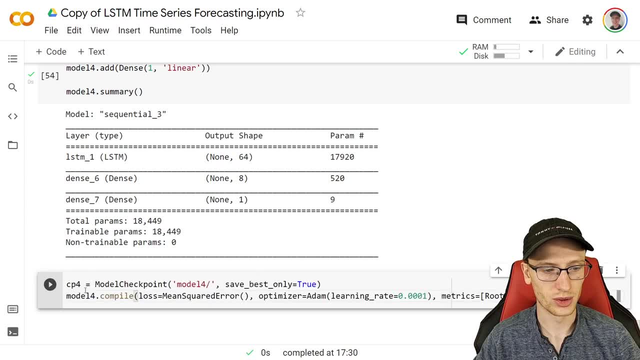 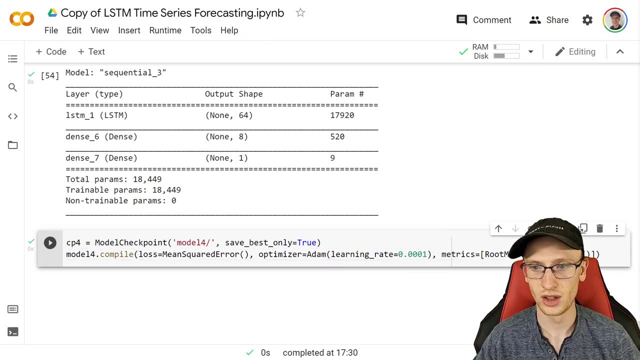 above. we're going to do just exactly the same thing, so really don't worry about this. Another checkpoint and another compile, and we're just going to compile that. It works exactly the same way. We're going to fit it with the x2 data, so model4.fit. 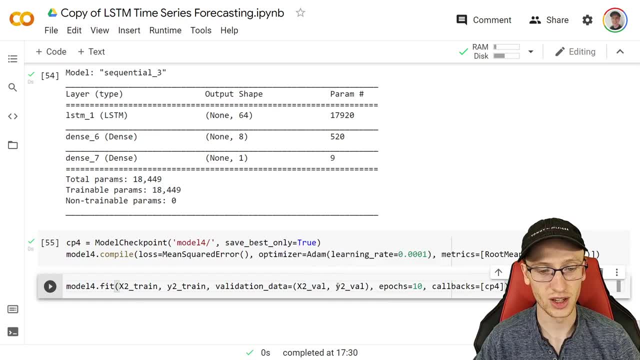 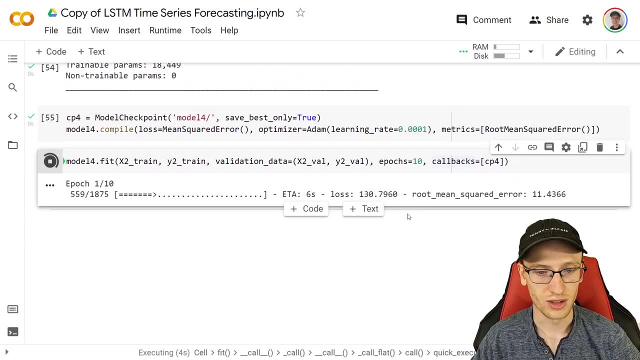 with the x2 train and y2 train, validation data of x2 val and y2 val and epochs like so, And I'll show you at first that this is going to work. As we can see, the loss is going down very rapidly and, yeah, I'll talk to you later. 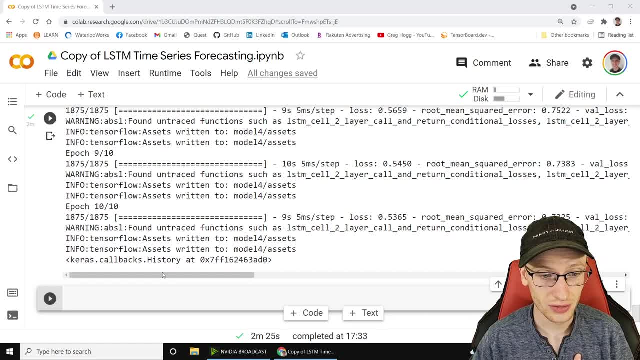 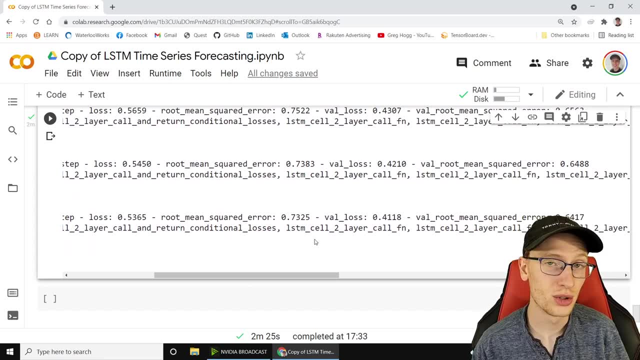 I'll talk to you at the end of the epochs. Well, it's at the end of the epochs and actually, fantastically, we have a validation loss of 0.41.. If you remember, we were getting about 0.48 or 0.49 with the other ones. so definitely a significant. 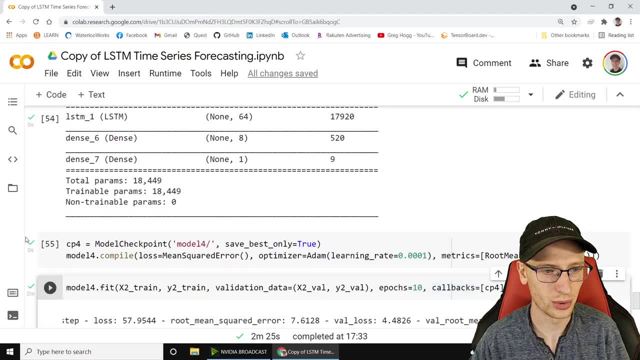 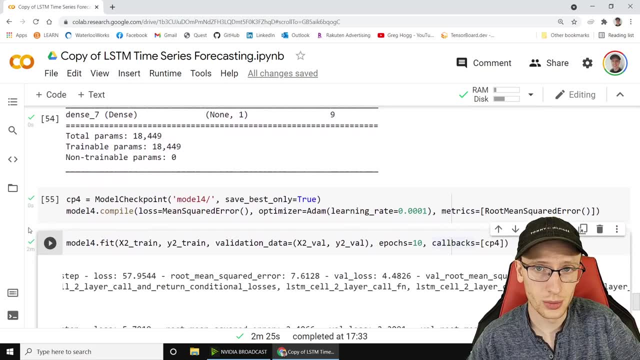 improvement with, honestly, not very much increase in the parameters. It was like 17,000 before and now it's 18,500 or so, So not much more heavy duty of a model, but a lot better. That is awesome. So now that we understand, 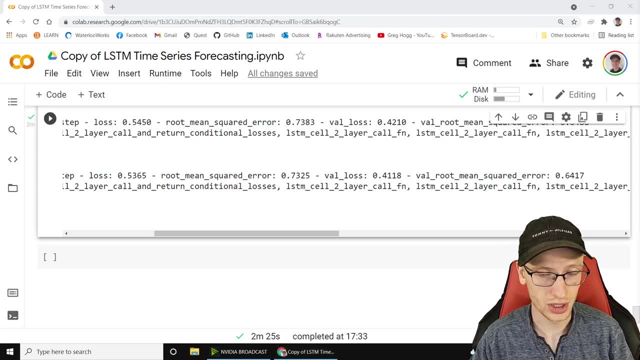 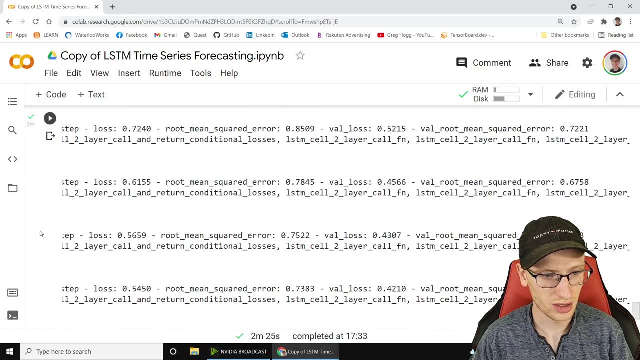 how to do that and we made a model. we are just going to use our plot predictions function, So I'm just going to write in plot predictions1, model4,. is that the right model? Yes, it is model4 with x2 test. 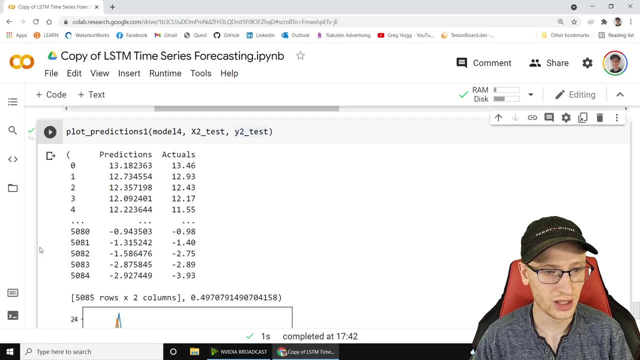 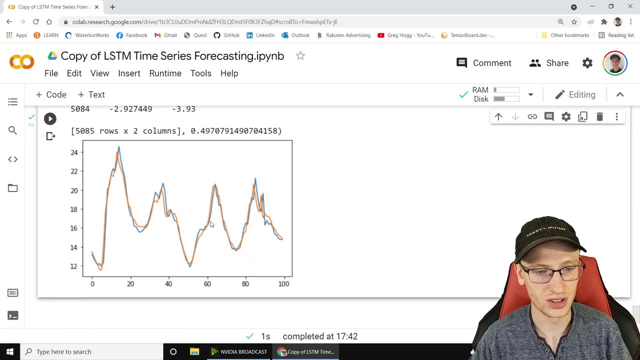 our input and our output for the test. and here we go. We can see here: the predictions compared to the actuals are very close and our models, you can see it's predicting very, very close every single time. So even better than before. we can see. 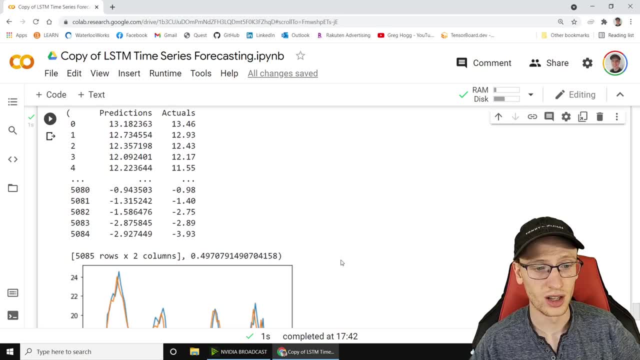 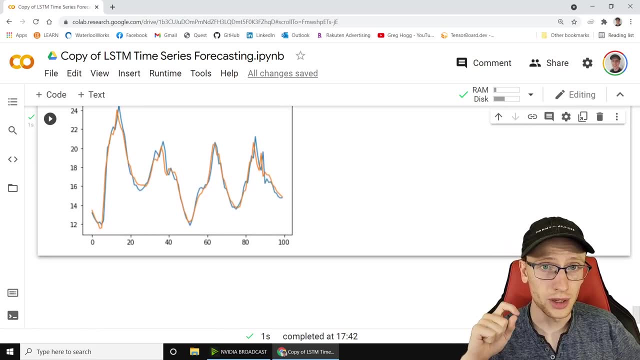 this is the valid test loss, I guess, is 0.49 and really, really awesome. Okay, so we are. we are pretty, pretty darn happy with that model, but I want to add one more thing in here, which is the pressure. Okay, so we are going to add in: 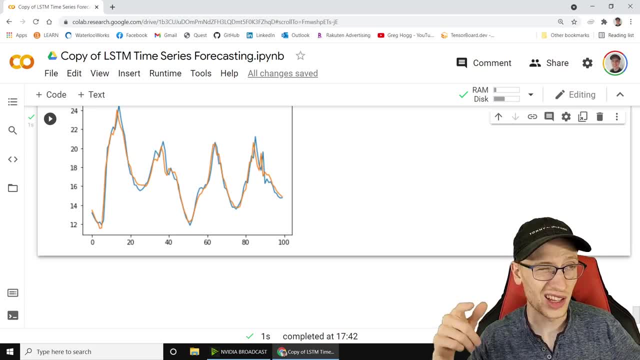 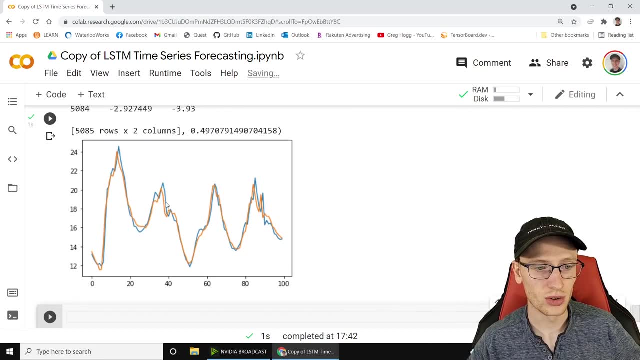 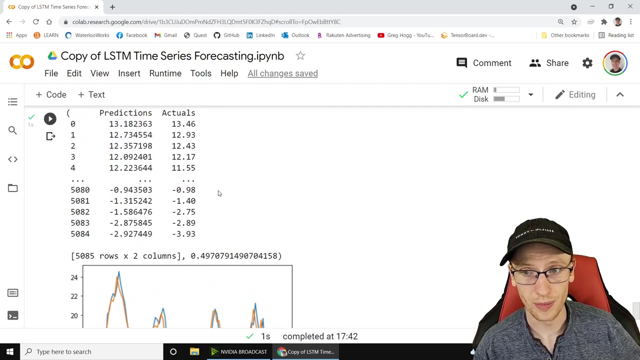 the pressure, as well as the pressure as an output. Okay, so we're going to add in the pressure, using as a predictive variable, but we're also going to try and predict it as well. So we're not just predicting temperature, we're going to predict the the pressure at each time step as well. So they're going to be. 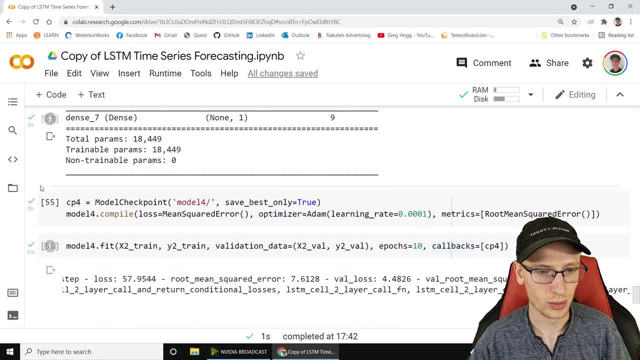 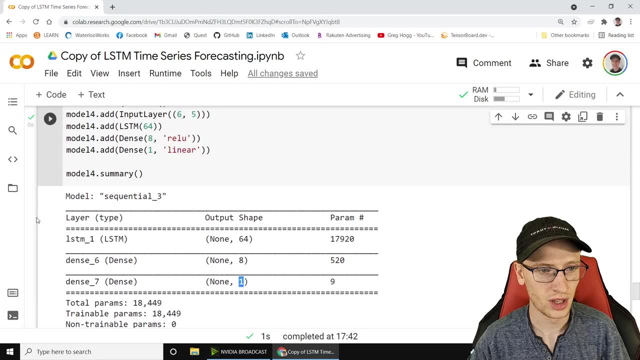 exactly the same as before, and that's why we're just kind of leveling this up more and more each time. except, instead of a one here, this is going to be a two. for our model, we're going to be opening two things, and we are also going to be 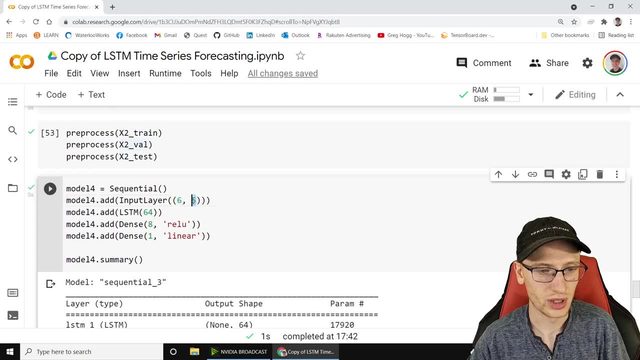 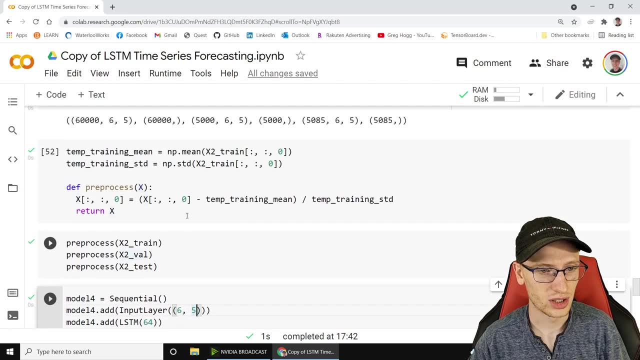 inputting. it'll be the same here, except we're going to be having another variable if we choose to use it as input. you really do want to use use it as input, so we're going to put it there as well and that's going to change our data. 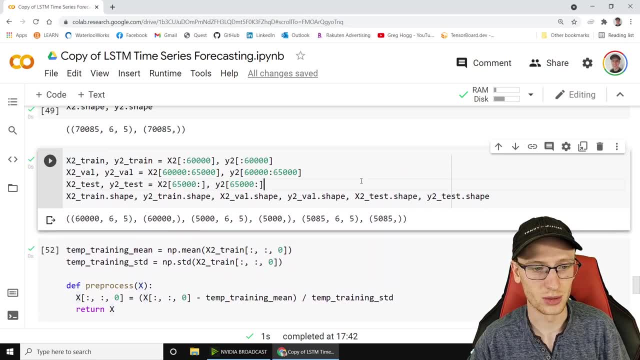 set here a little bit. It's going to have another variable, but that's really, that's really it. and the output. the output y2 used to be this long vector and we just had vector that values comma, but now we're going to have comma 2 because we have two different. 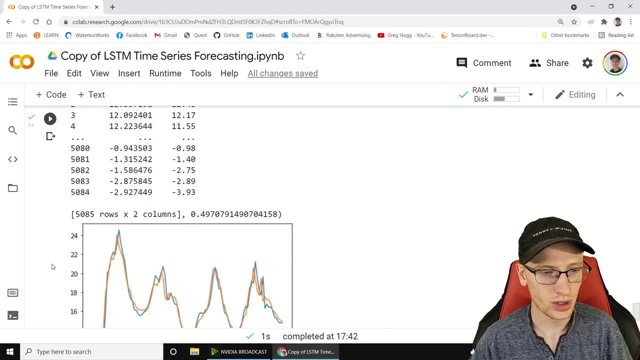 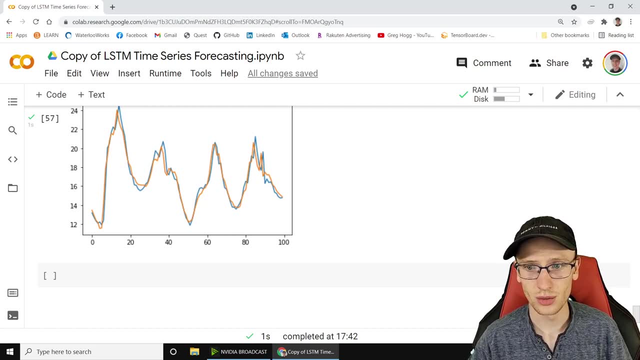 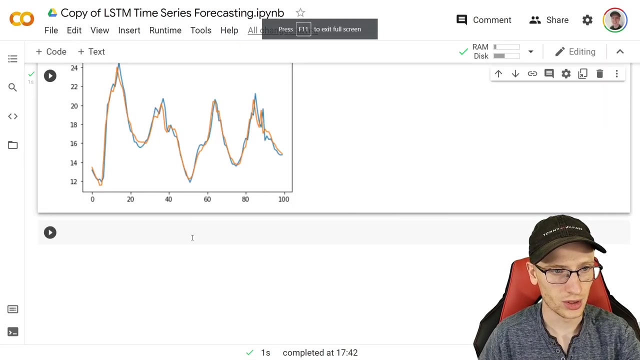 ones. Okay. so, knowing those changes, we're just going to go down and and make them one at a time. So okay, here we go. we're going to start with making that, basically adding that pressure to the data frame. So here we have P, temp, df. sorry that didn't type. oh, I forgot to make this f11. sorry about. 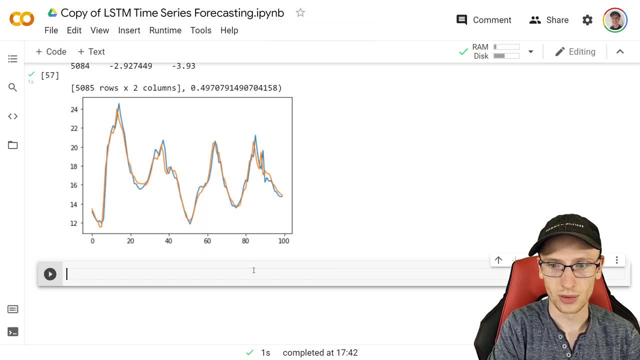 that Okay. so we're going to do plot, not plot predictions. P, temp, df, which is just the pressure and temperature data frame in one, is equal to the PD dot cat. we're just going to be adding this column into our other data frame. we're going to be 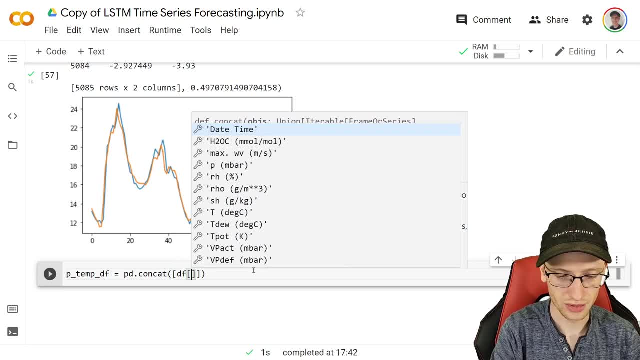 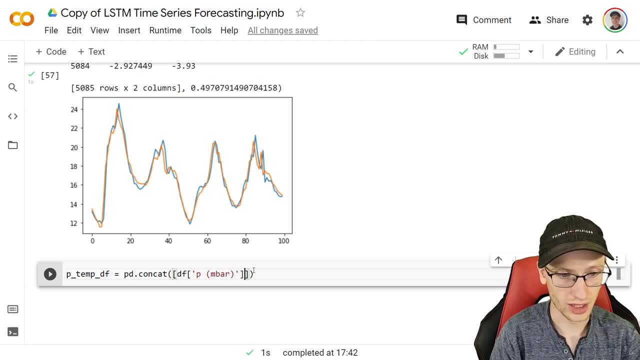 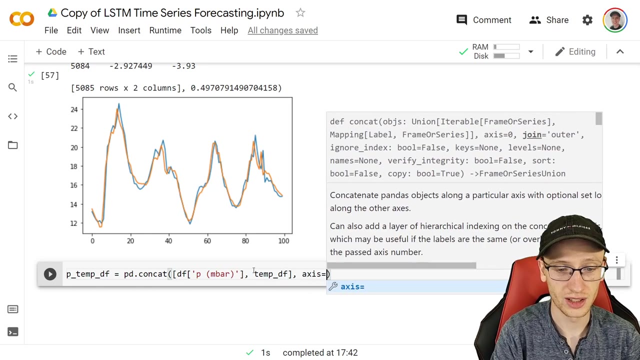 concatenating df. we'll just put it at the front here: df, P brackets, m bar happens to be what pressure is in the data frame all the way at the top. we're going to be concatenating that onto tempdf, basically horizontally, like this, or however you want to call it: x, x equals. one makes it so that p. 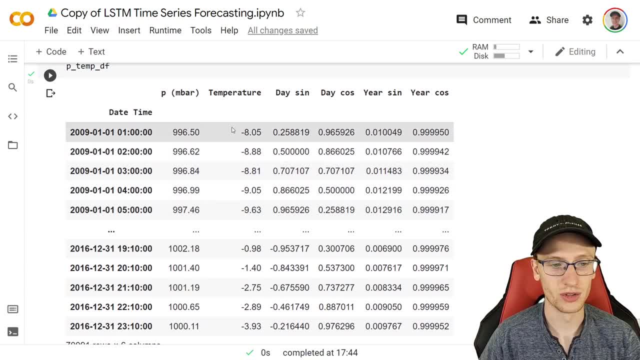 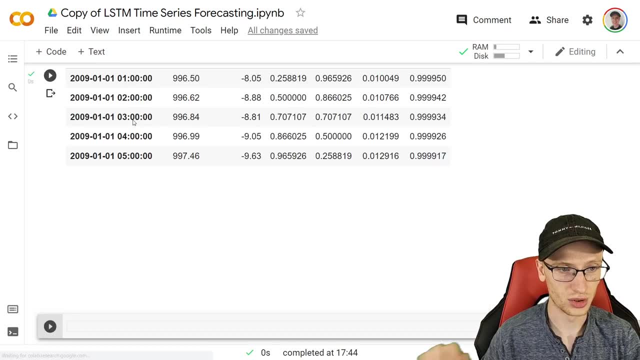 temp ef looks like this: okay, it's just some code that really adds it in that the column there. okay, so now, if we have that- and i don't really don't really like that- just show the head. it's too many, too many information all at once, uh, and now, so we're going to take that. they take that. 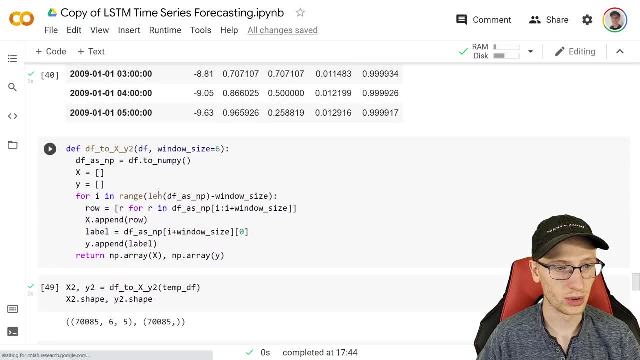 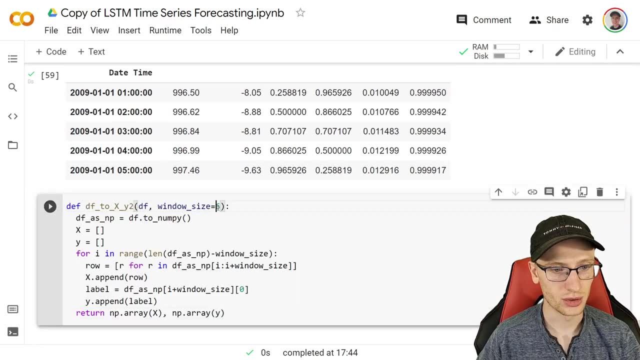 function as above the- uh, the window making one. we want to get our input and output pairs back, but we are going to modify that for our use case here now. i am also going to change the window size, just because, again, we actually made it so that we would have had six variables and that. 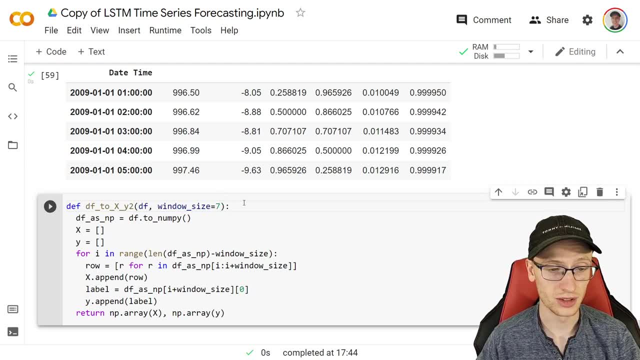 would be six by six, so we're going to do six by uh, or seven by six instead, i guess. and so here, what actually changes in this function. well, i'm going to call it three, just to make that easy, to make a lives easier, and it's going to be very, very similar. so it's still going to be this bracket r. 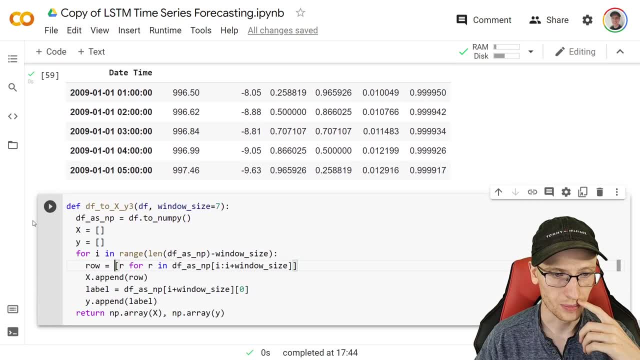 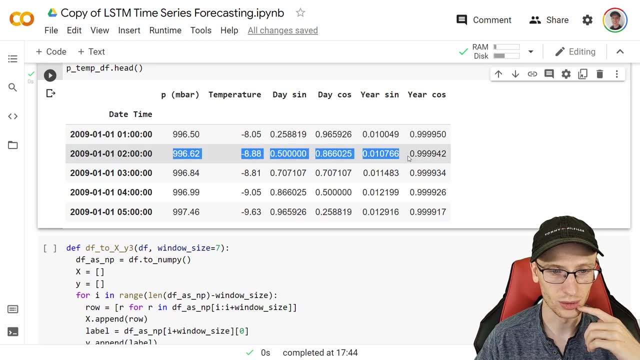 for r in this and it turns out the way we wrote this. um, it actually doesn't matter. we don't have to change that part at all, because or the input part, because it's still going to be: just append the row and then the row and then the row. so that's totally fine. the only thing here is that 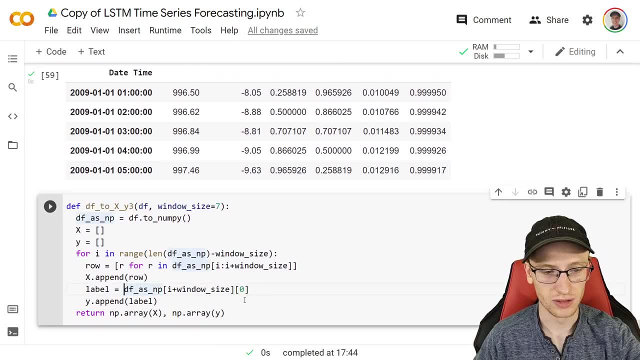 we want our output to be. we want to be appending a list where it's going to be. the list is going to be that. so the first thing, and that's sub deferred the. the second thing, like that. and there's other ways you could write this a little bit cleaner, but this is totally fine, like that, and append the label and make the array. 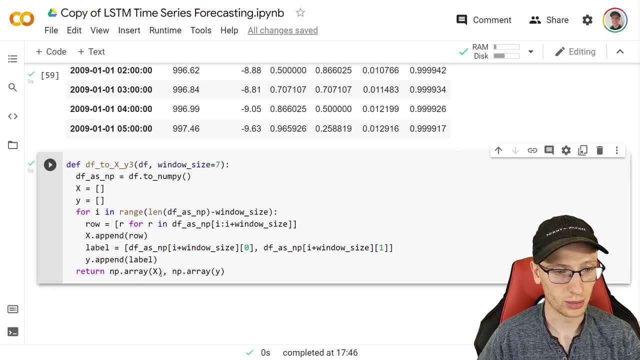 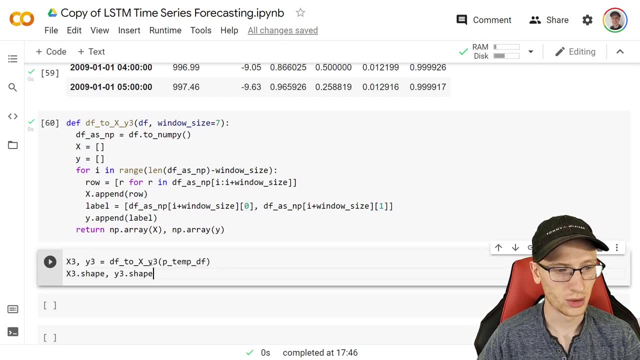 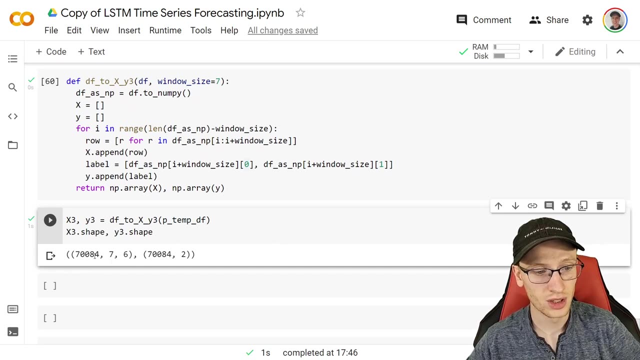 and that's fine. okay. so then if we, if we get our input output pairs- i don't know why it's there- i'm going to press this button a bunch of times, i just never. i never have codes in a code block somehow. so here, and i know, uh, krishna does that a lot as well. so 7084 by seven, by six, so number of: 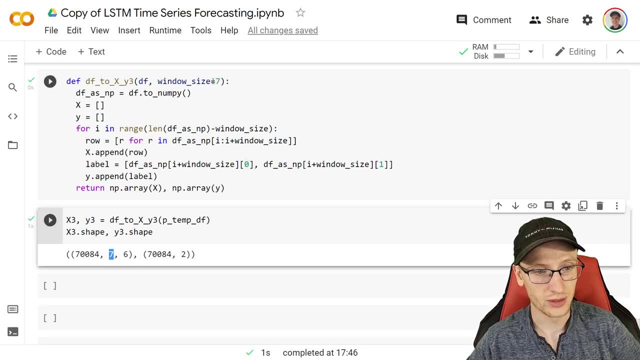 information or number of training. examples: times the length of our window, that we're using the last seven hours to predict the next hour, and then six variables, and then our output is going to match up, except we're going to be predicting the temperature and pressure all at the same time. 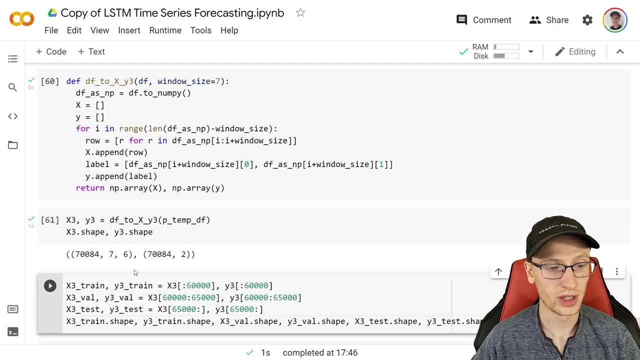 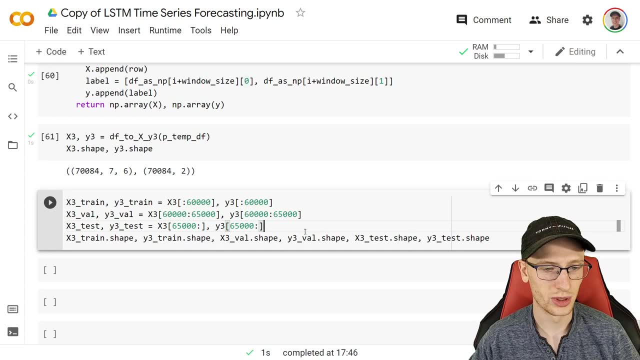 we're going to copy and paste this thing in here because it's really boring. it's just splitting it exactly the same way as train, train test and val. we could have wrote a function for this. we wanted to, but copy and paste is honestly fine for these kind of things and i'll 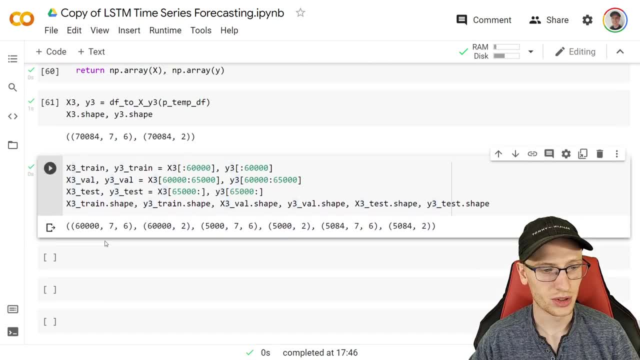 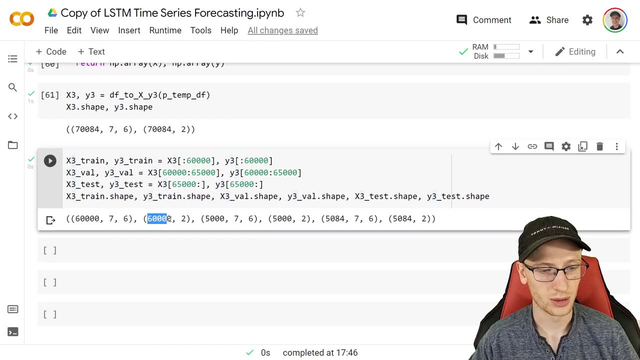 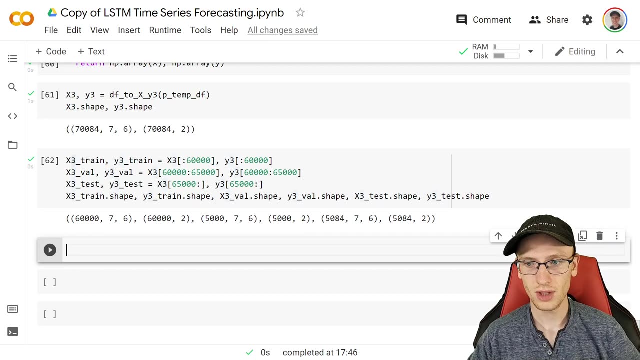 all it is is changing two to three, and that's literally it. and the shapes are as follows: seven training examples by window length, by variables, and then training examples by the, the variables, which are training uh, temperature and pressure, and it's like that for all of them. now we're going to 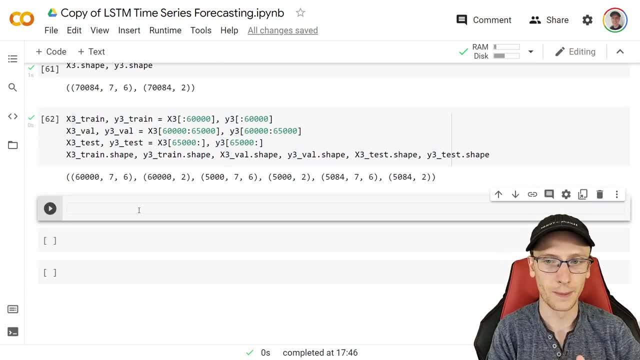 do something very similar. we're actually just going to write this out, but it's mostly mostly copy and paste from above for our pre-processing, and what we'll see shortly is that we actually want to. it's probably not that big of a deal, but we probably also want to pre-process our 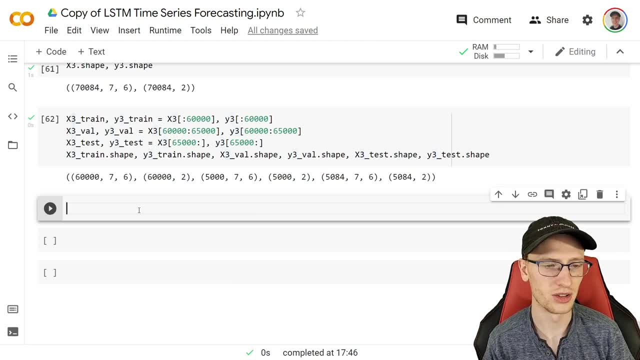 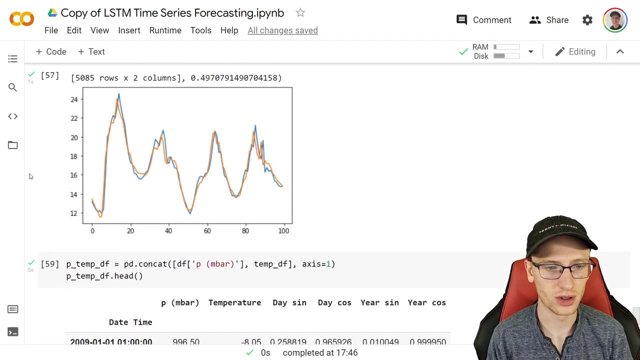 output as well, which has some complications- we'll see that- but it's not that big a deal. we want to pre-process our output as well, because now that we're, if we look at the different values on on temperature pressure here, they're a lot different. okay, so these, these values are a lot. 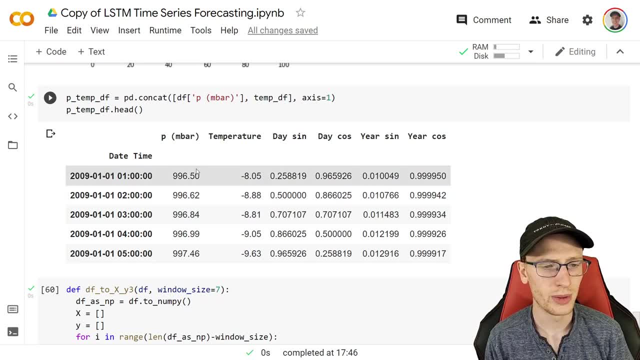 bigger than these and our cost function or our network may be tempted to to try to impact these errors a little bit in the other direction or in that direction, and so you'll notice that we've more than these ones, because that's going to increase the value of the loss. So we do want. 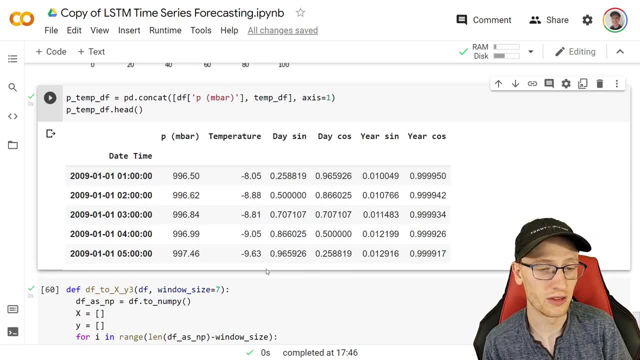 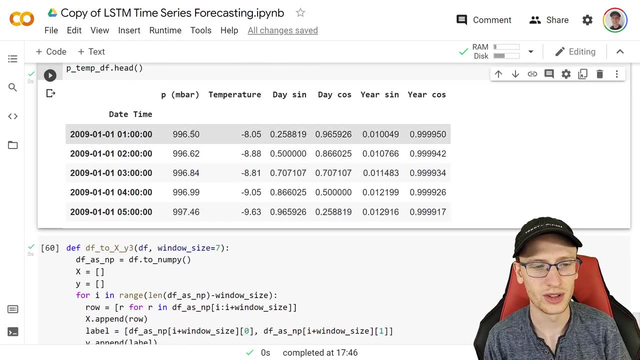 to try and put these on the same type of scale And we'll be able to restore that later with we'll call like post processing to kind of restore these values from the predictions as well, Since, since we'll be telling it basically try to predict only like between negative three and three and 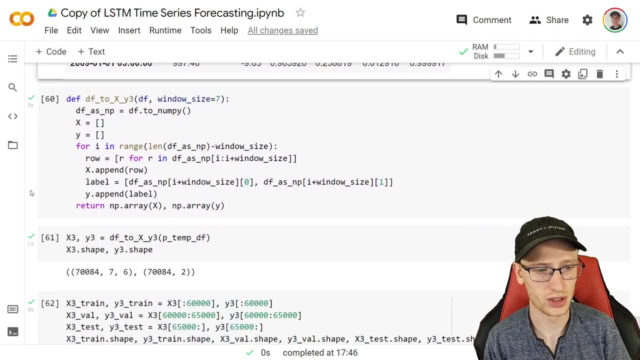 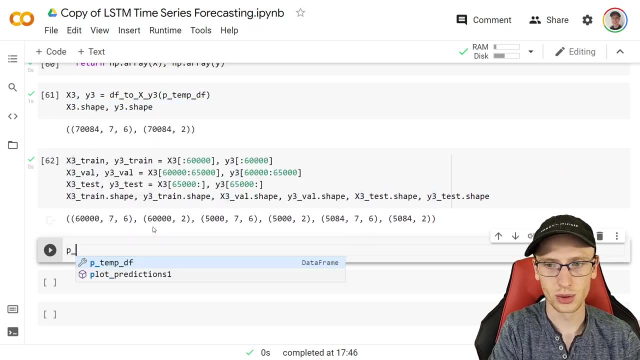 negative three and three. we want to be able to restore the actual prediction as well. Okay so, but for now we're going to just make up our pre processing the input as well. For this we're going to for need pressure training mean we'll just put a three there is equal to the 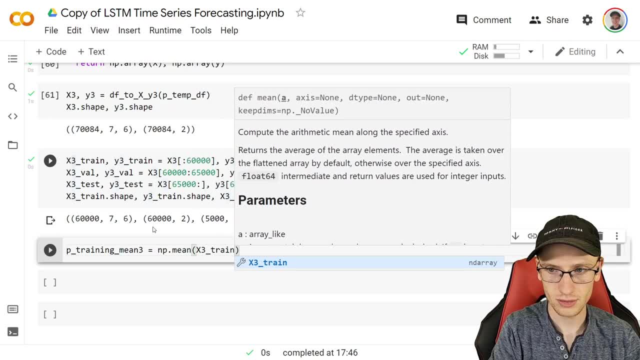 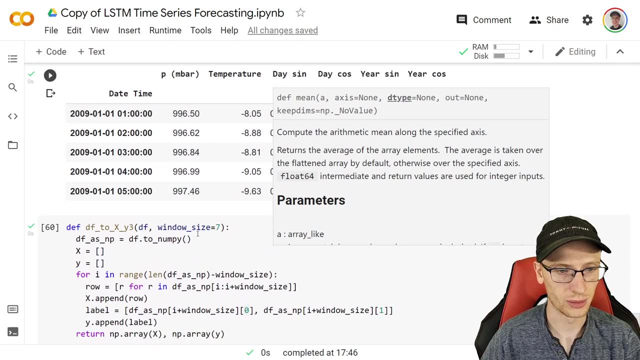 numpy dot mean of x, three train sub colon, colon zero. Okay, so now that actually took over as the first column there, So that's that's why that's the zero And we're going to copy that but replace. 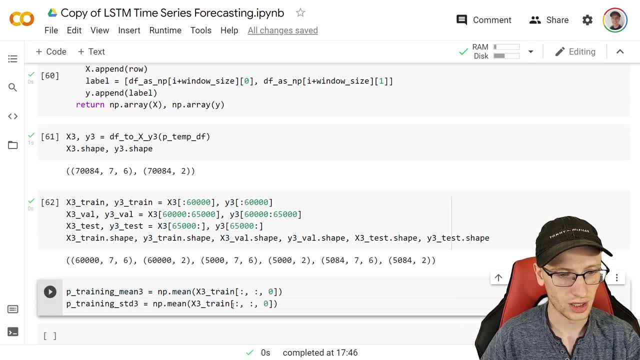 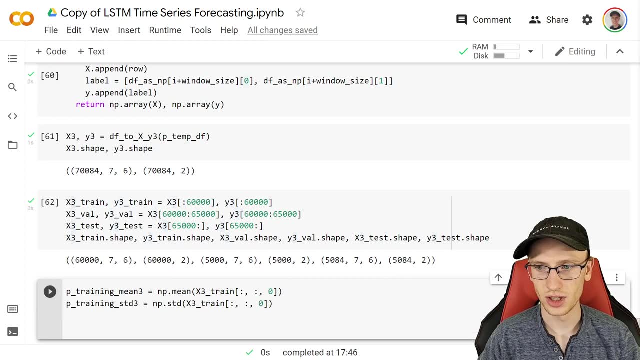 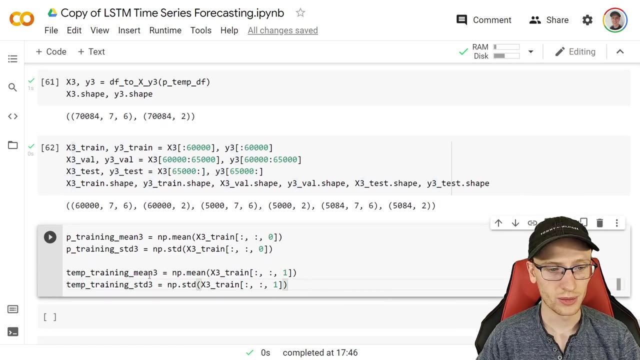 that with standard deviation, with an STD, And that's fine, And that's going to be STD there. Okay, so we need those as well as the temperature, And I'm just going to copy and paste the temperature because that's not overly interesting. And yeah, okay, so we have both of those variables Now we 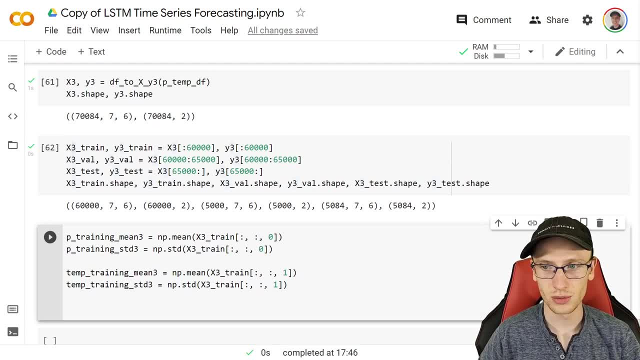 can write a new pre process function. So how it looks was pretty much like this: this before pre process three. Actually, no, I'll just write it out for you to make it clear. So define pre process of: we'll put a three there of x. this is actually just preprocessing the input. 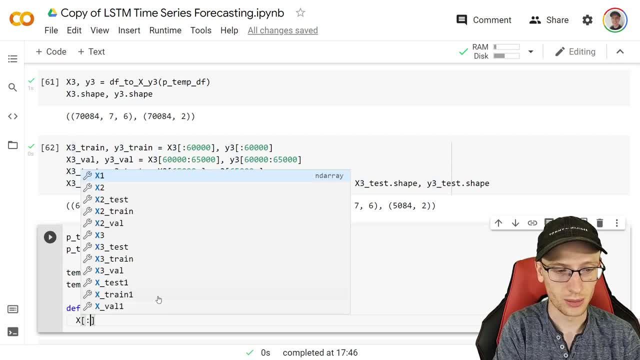 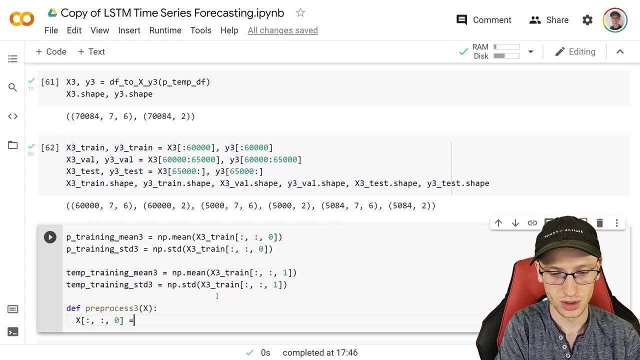 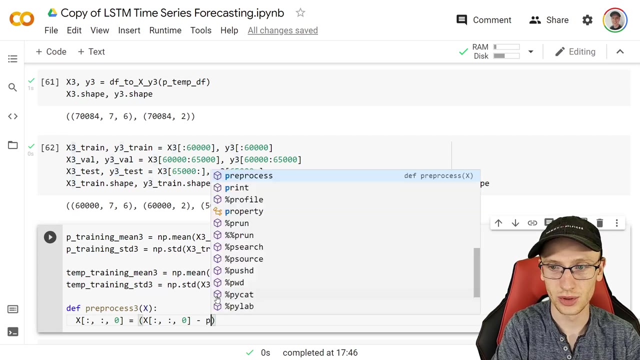 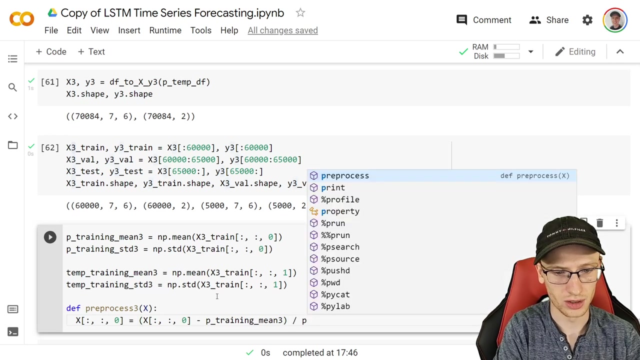 preprocess three, x. it's going to do exactly the same thing, except to do that with both columns. So we want to do set all of those equal to equal to itself, itself, like that. And then this is about the pressure. So we want to do p training. training mean three, and divide that by p, p training. 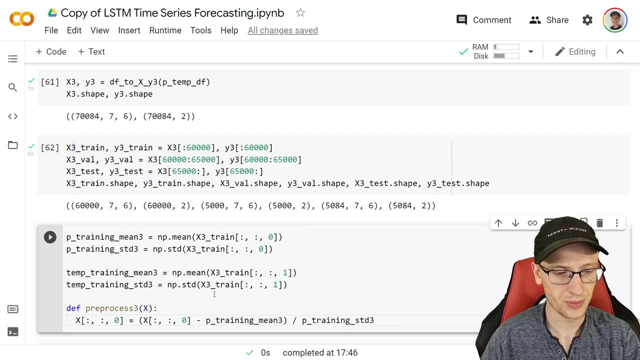 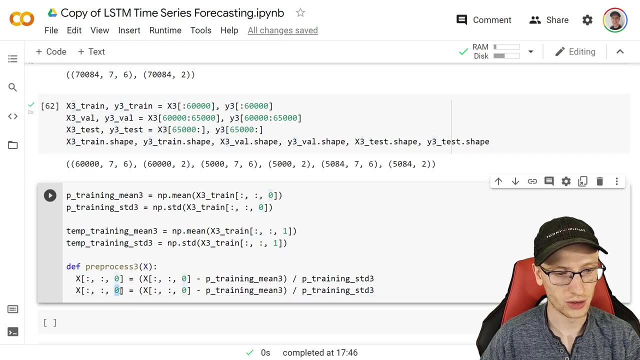 peach- sorry it's not showing up- p training STD three. And then we want to do exactly the same thing, except change the the temperature column. So that's going to be one now. So one and one, and this will be with temp. 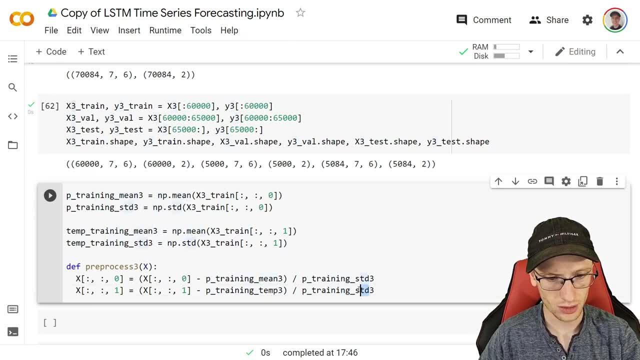 three. By the way, these sorry one second. I'm acting like you're. you're like talking to me, I'm talking to you, So I'm acting, nevermind. I don't know what I'm talking about. So basically, 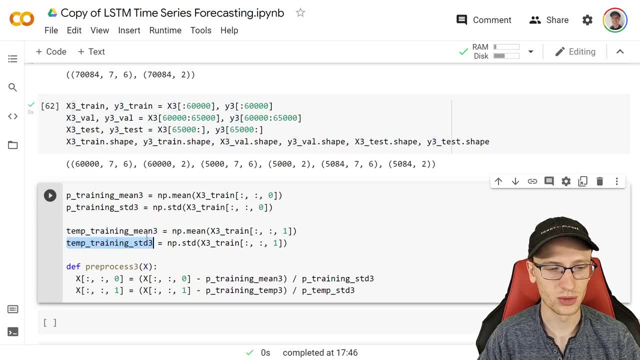 these values here. we didn't really have to gather them Again. it's pretty much just the mean and the standard deviation of all the temperatures, which we already did that earlier. But it's a little bit cleaner if we have this here as well. 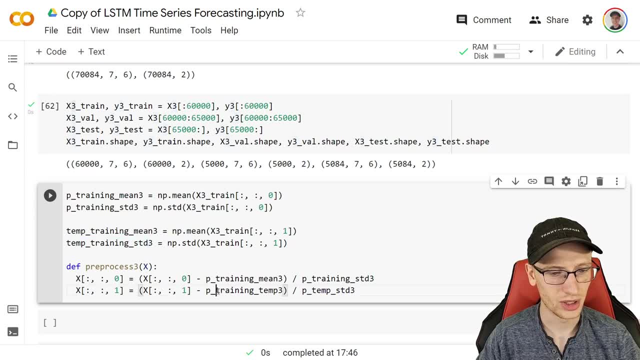 And why do I feel like I messed something up? Yeah, I did, Peach. Yeah, I figured that this was wrong. This is temp training, mean training, mean three. And this is temp training, ST training, STD three. Yeah, I was mixing them up there. Okay, so that's going to be our preprocessing functions. 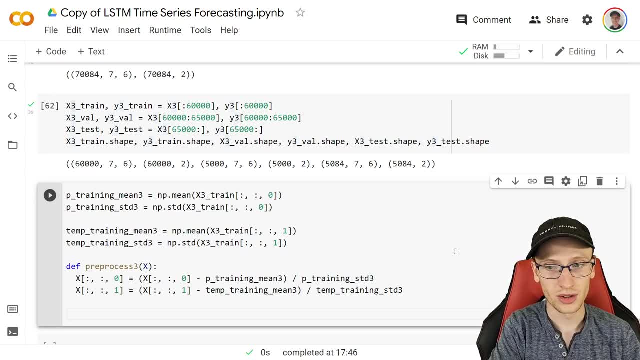 for the input as well as the input. So we're going to do the same thing, And actually I will just copy this one for you, because it's exactly the same thing, except we're just setting it differently based off how the 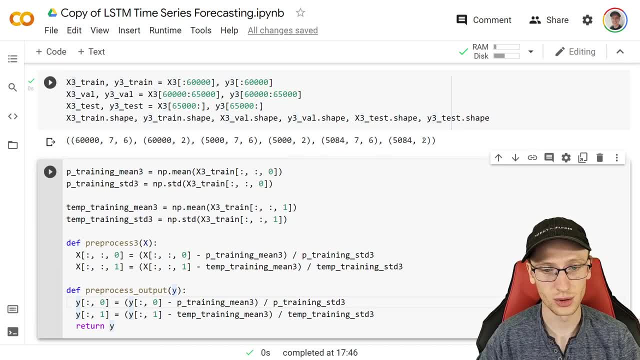 output looks. If we remember, the output looks like this: 5084 by two, for example. So we're just going to say all the rows and then the first column corresponds to the pressure. So we're going to minus those all by the pressure and divide by the mean of that and then divide by. 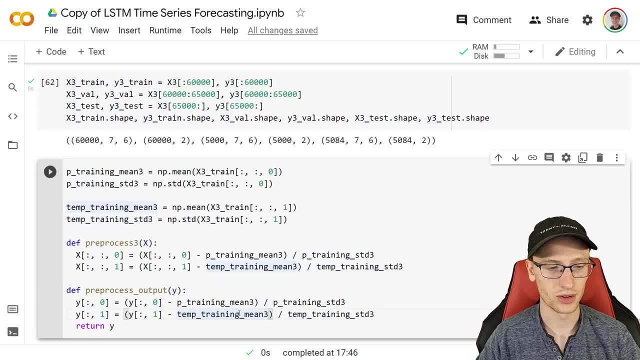 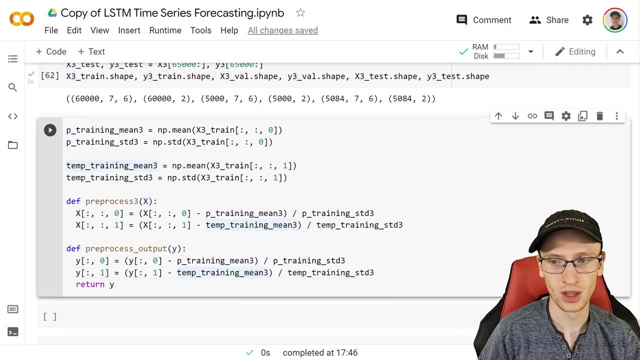 standard deviation, And the same thing for the temperature part. So that's a little bit weird how we're doing that, And it might not be totally necessary, but it's probably a good thing to do. Okay, a lot of talking, a lot of talking. 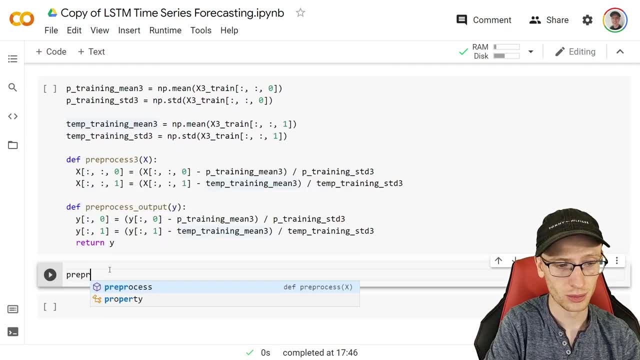 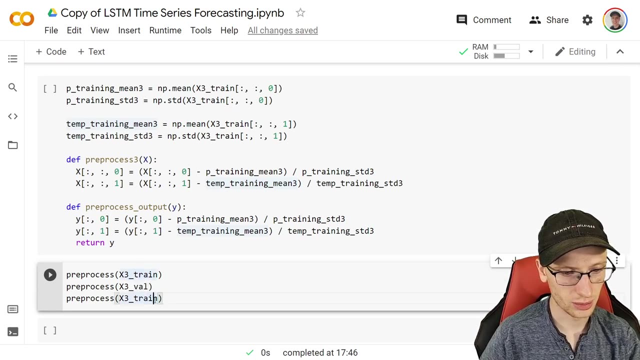 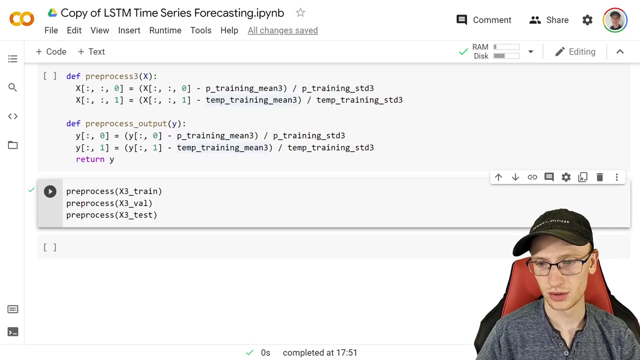 so it's getting a little bit sore. We want to preprocess. preprocess the x3 information for all those x3 train, x3 train, val and test. this is going to be val, this is going to be test. Those are done. Okay, preprocess all those. I'm going to kill the output. We also want to 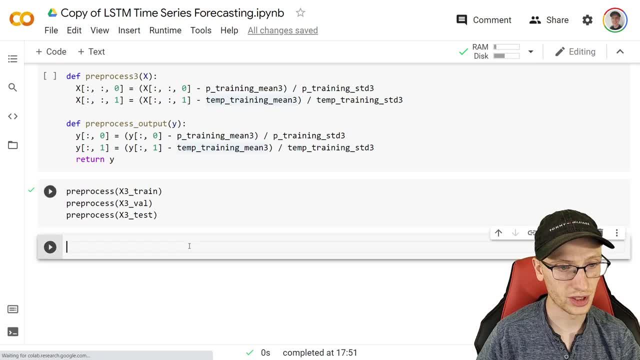 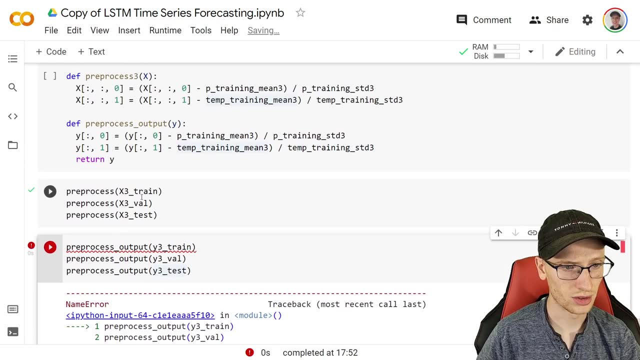 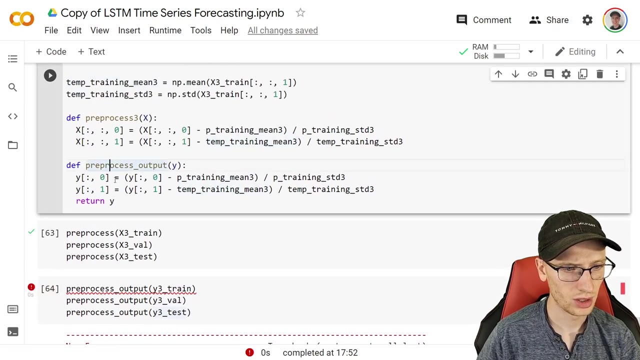 preprocess the output. And just to do that quickly for you, it's going to be the same there. It's just preprocessing the train, the validation and the test. Happy with that? No, we're not. I must call it something different. preprocess output is not defined. preprocess output is: how is that? 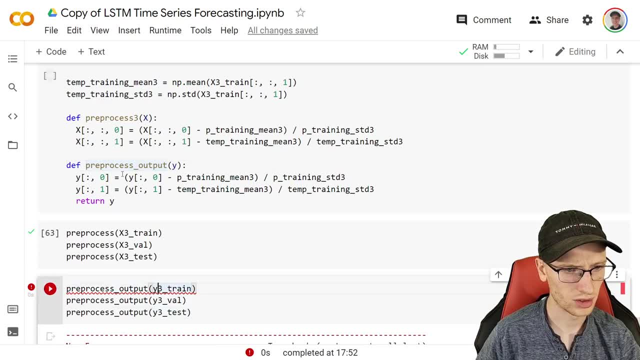 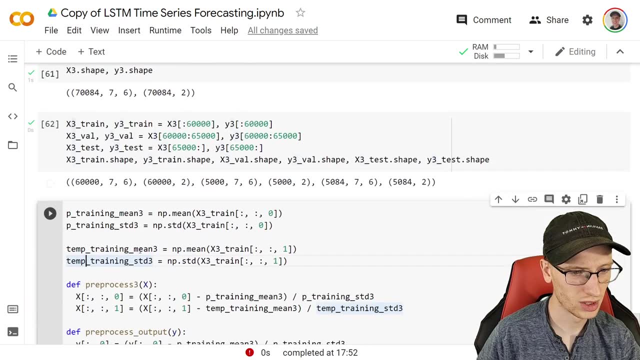 not defined preprocess output. Did I not call that? I thought I called this. I'm just going to do this again because I don't quite know what happened there, Because the name name definitely looks the exact same: preprocess output on y. So 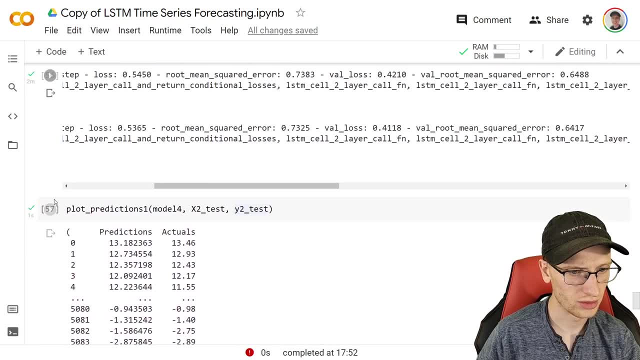 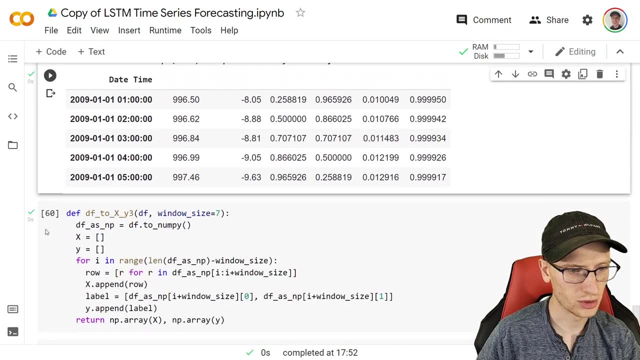 I'm just going to run this stuff again, because it gets a little bit weird If you do have to run it again. Where did it come from? Where'd it come from? Where'd it go? Yeah, okay, so those variables look right And I recall that function. get that again. get that again And make sure. 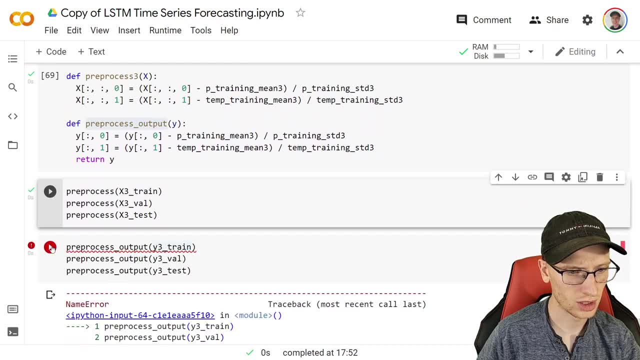 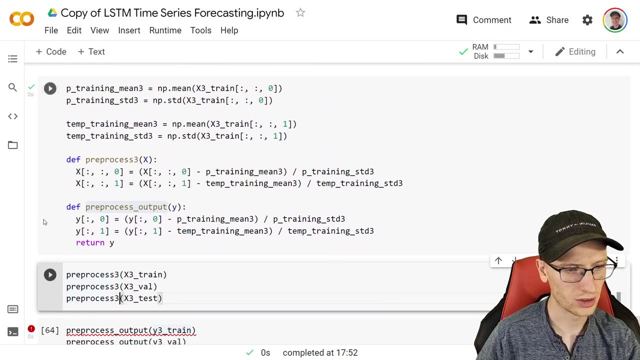 that's ran. I'll preprocess And I will. oh, it's because preprocess. Oh, I wasn't calling three there, That should be a three. Yeah, sorry about this part. I like to leave it in there, just to show you what happens. 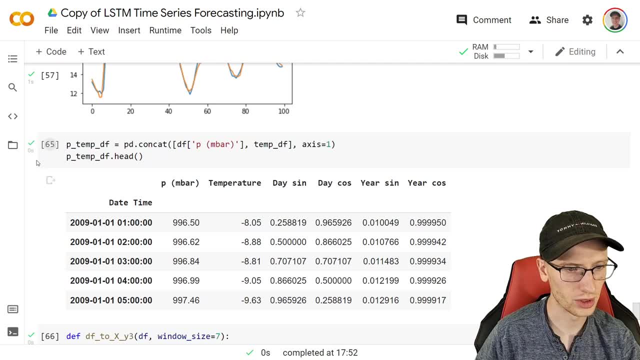 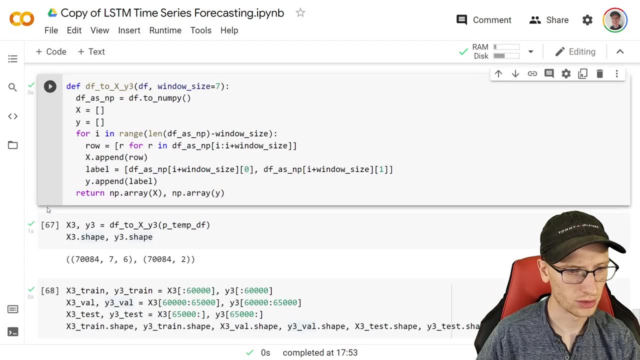 If you do kind of mess something up a little bit. I don't like to pretend everything's totally pretty, So I will get that again. P temp df is going to be that information on the function don't really need to do that. The x three and y three, x three train and so on, This stuff. 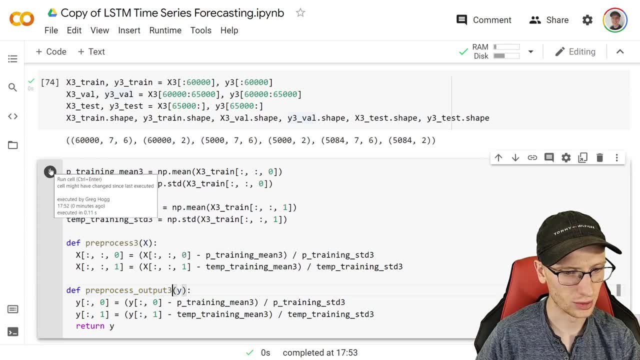 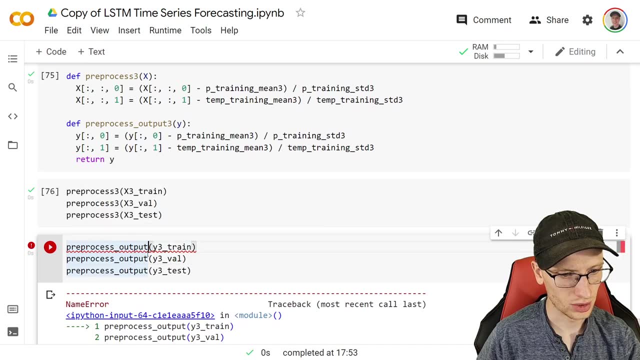 I really should call that, call that three, because that's a little bit weird without that. Okay, preprocess three and preprocess output Three should definitely be defined here. I'll be confused if that one doesn't work. Yes, that's totally fine. Okay, so sorry about that. And now. 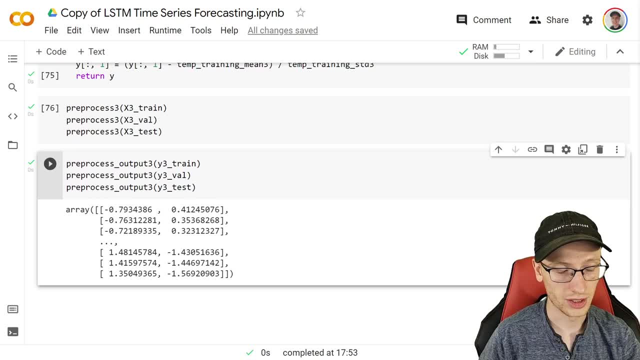 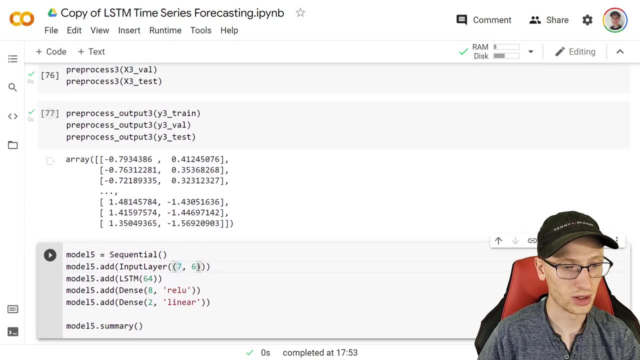 let's make a new model Now. it's going to be basically the exact same thing as above, So I'm very happy copy and pasting because it's not too much effort. The input layer is going to be again the number of the. 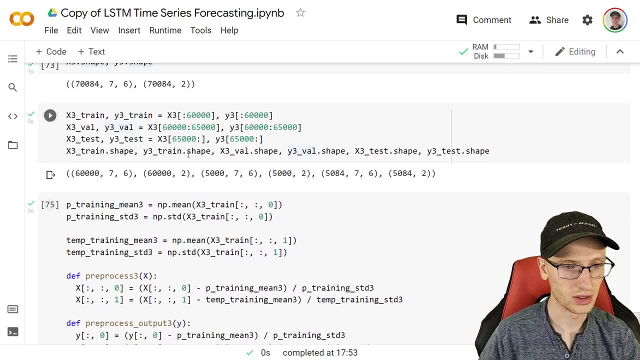 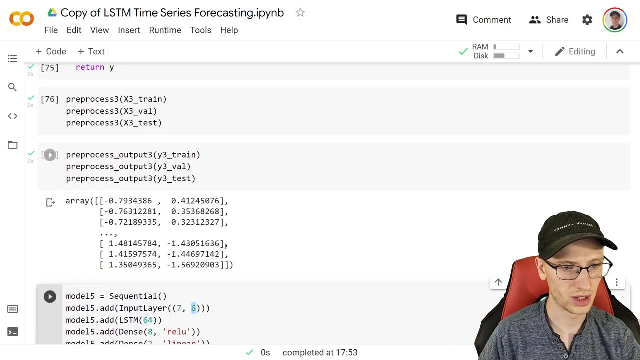 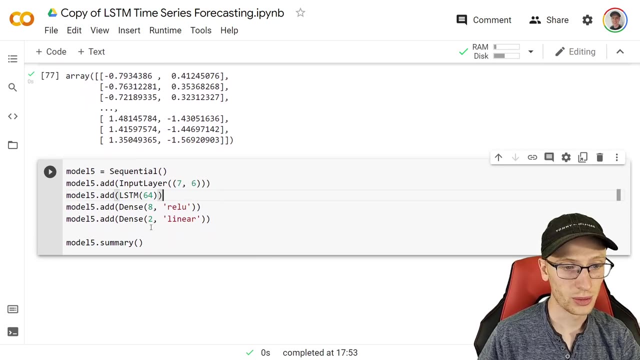 the number of the window. So then the window- I changed that to seven to match that seven that we were using- And the value here that is going to be the number of variables, which is six, as is correct, as we can see from the six here. Okay, so we have all of that And, yeah, that should make. 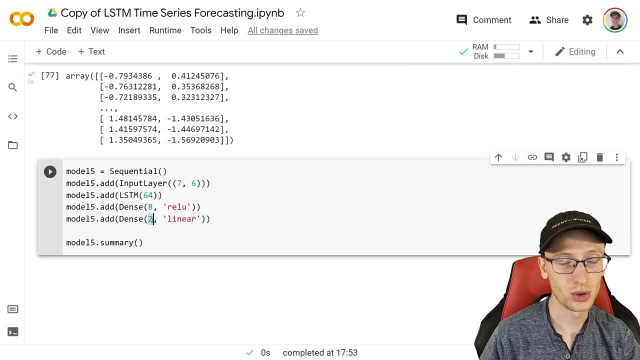 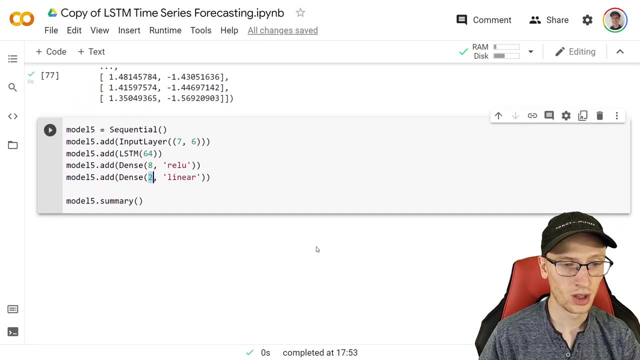 a model, because we changed this off screen and change this to two. So that's saying, okay, the first spot is going to be, say, for pressure and the second spot is going to be for the temperature. So much talking and getting really tired, But there, those are. that's what we're going to be. 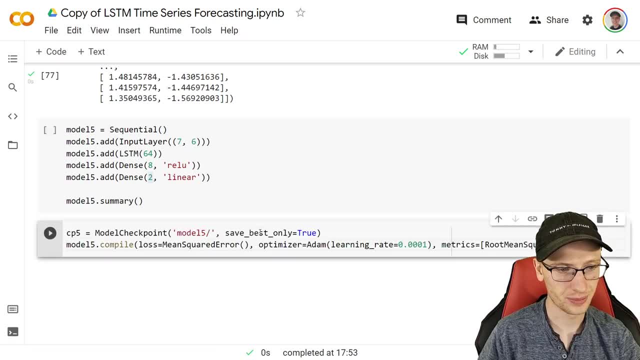 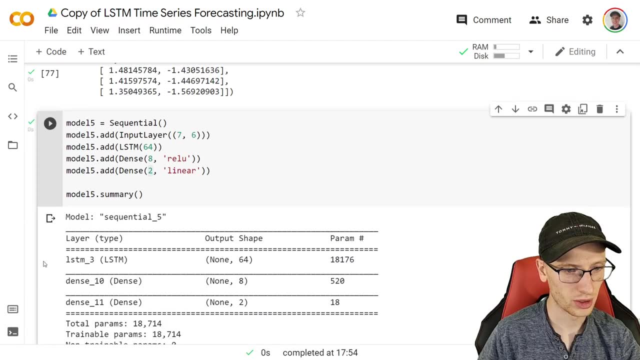 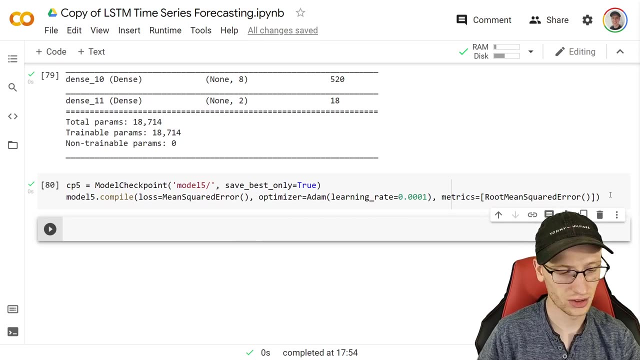 doing. We're going to copy and paste the checkpoint here. CP five is totally fine to match up with model five. Sorry, I'd killed that Model five. there's our model CP five. I don't know why these things are never coming in. And then model dot fits And luckily I can take a little bit of. 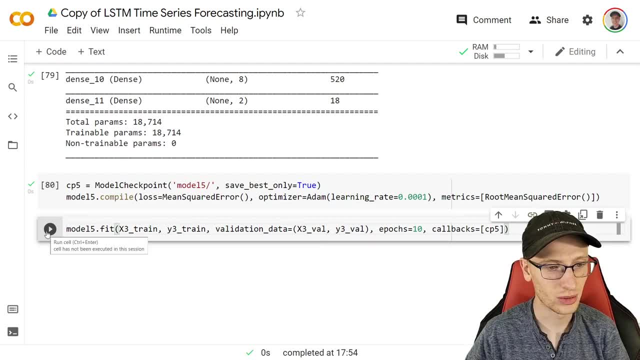 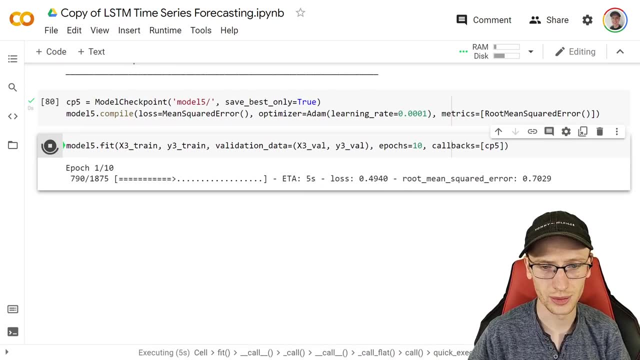 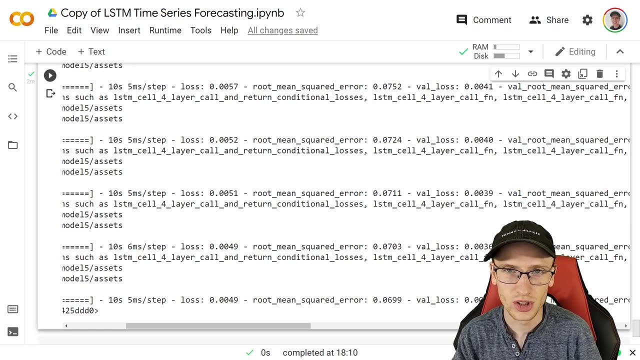 a break because I've been talking so much, getting tired And that's going to run with the x three and then model four And then model five. there's our model five And we can see that we have a very tiny validation loss. Now recall that we did do this pre processing on the output, which makes 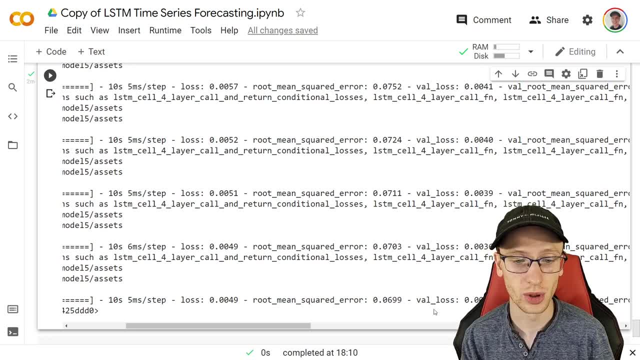 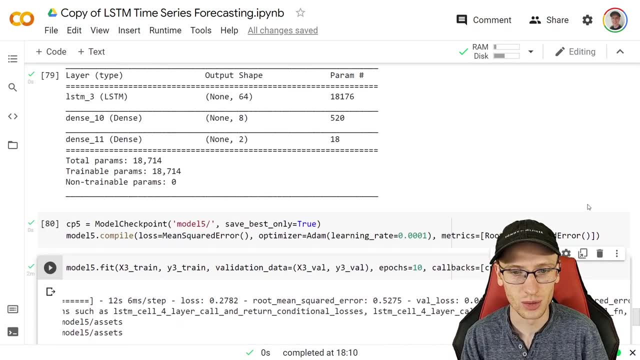 them those values a lot smaller and therefore a make a lot smaller, loss as well, which doesn't that doesn't mean anything good or bad. It just means that the values are smaller And the thing that we care about is that, whether it's going up or down, and the validation loss, you know. 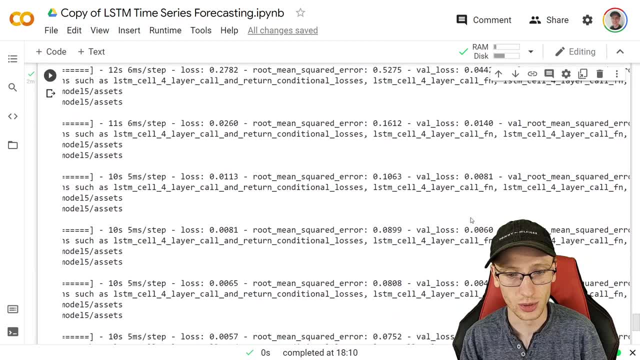 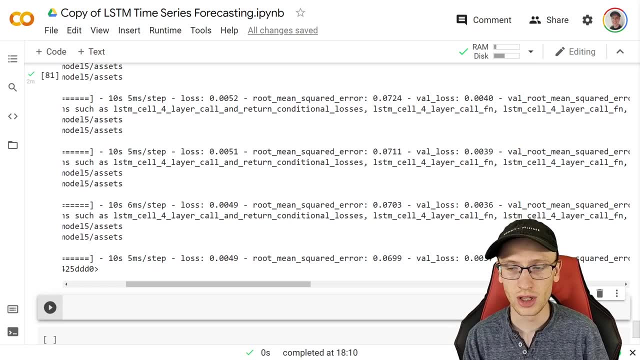 it starts at zero point four zero one. zero four zero one, zero one, zero zero eight one. it's clearly going down and down and down, like the other ones were, And so we look pretty. I think we're pretty happy with that, Okay. 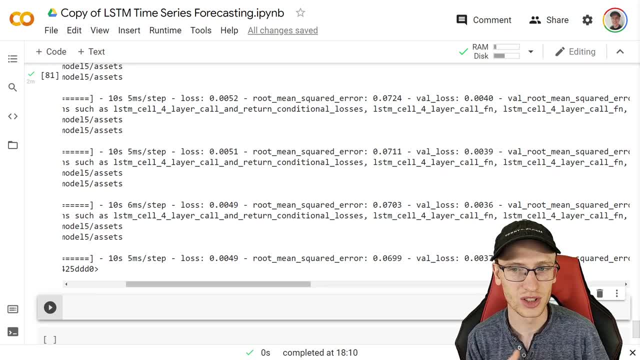 now I want to make a function that's going to plot pretty much all of this stuff at once, And I do not want to write it out with you because I think you can just look at it And I know we'll explain what it's doing. So here you go. I'm just going to copy and paste this function in here, which is: I'll. 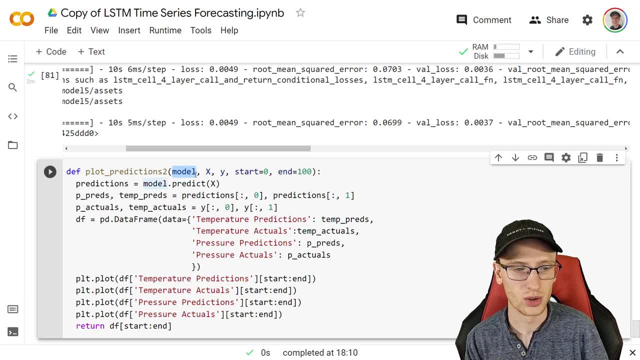 explain what it does. So very similar to our other function earlier for plotting the results it brings up. here where this condition kind of takes place. Yeah, i'm going to say I'm quick, And what that does is it muit pants the whole function, And this is where the roughness is going to be. 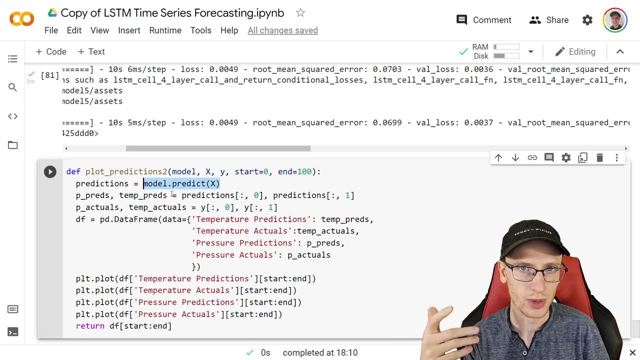 speeded up by using some kind of gradient感じ v渨, which is. I'm curious to see where this führen goes. So we're going to try to automate these two functions in here. So that's probably an imperfection here. So the first function here is okay. the first function here we got the 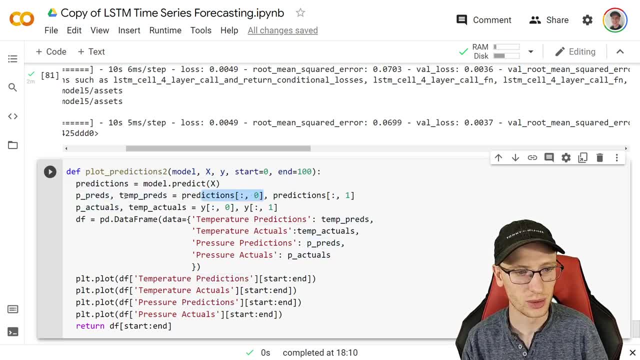 handed selection function here, that's one estouition parameter that's going to be hand selected is hand selected. And then the second function here, which I'll explain: this, the other And the actuals. since we passed in y, the pressure for the actuals is the first column. 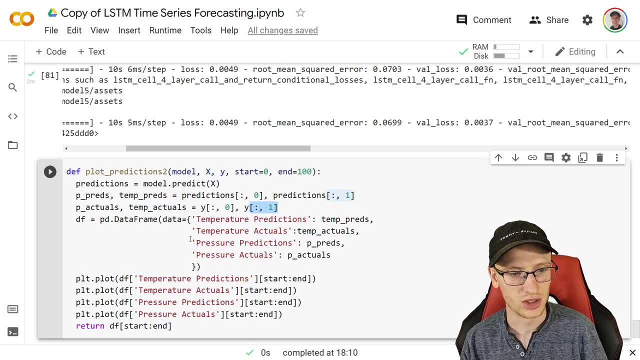 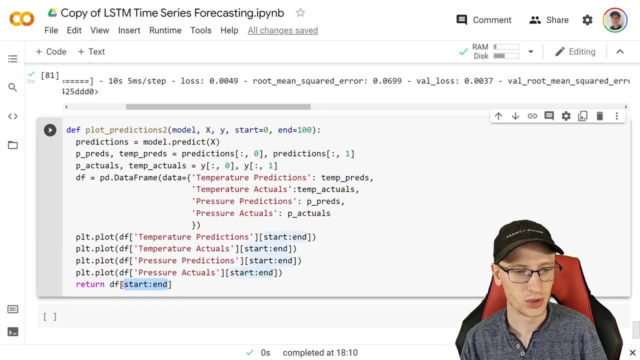 Temperature actuals are the second column, And then we're just going to make all of this into the data frame And we're going to plot all of this all at the same time, And then I'm also going to return the data frame for just start to end. 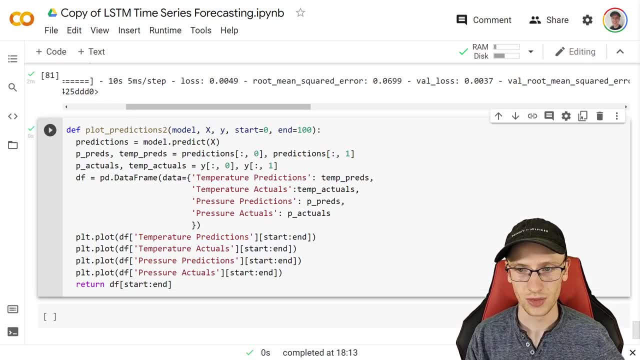 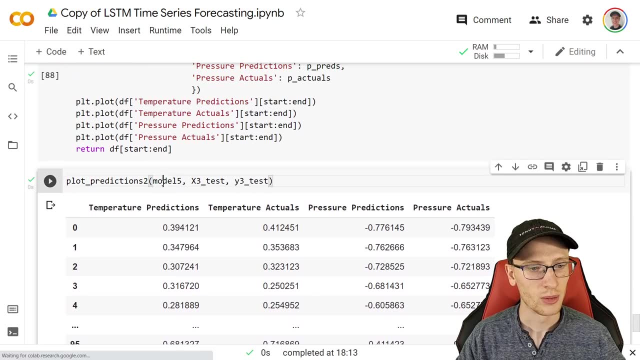 And I'll show you why we choose to do that. So if I do this- plot predictions- And I called that with- sorry, I did that too quickly- Model 5 and X3 test and Y3 test. So the input and the output there. 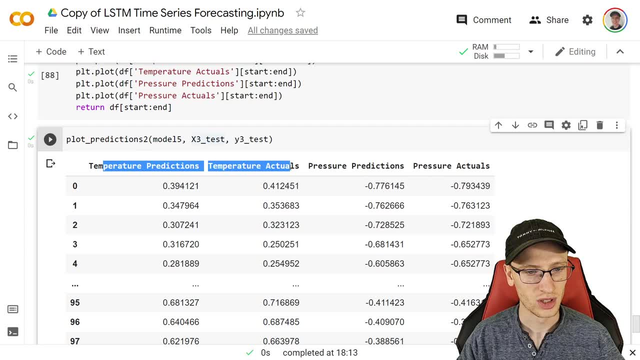 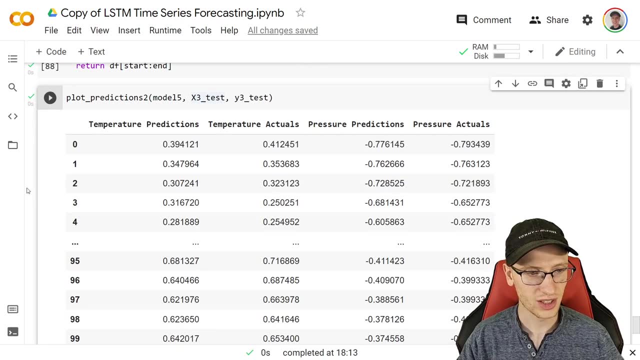 We can see, these numbers are very, very close. So for temperature the predictions are very, very similar, which is great. For pressure, they're actually very close as well. So that's fantastic. And here's just the first 100 results here. 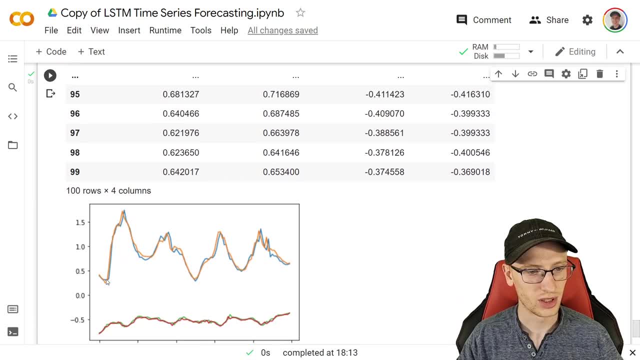 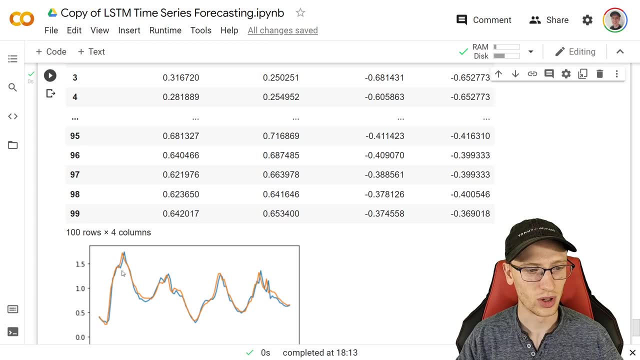 And this also plots it for the first 100.. We can see here the mapping is. again, I don't really know which one is the orange or blue, or which one is the red and the green, But the point is that clearly one of the two is forecasting this stuff. 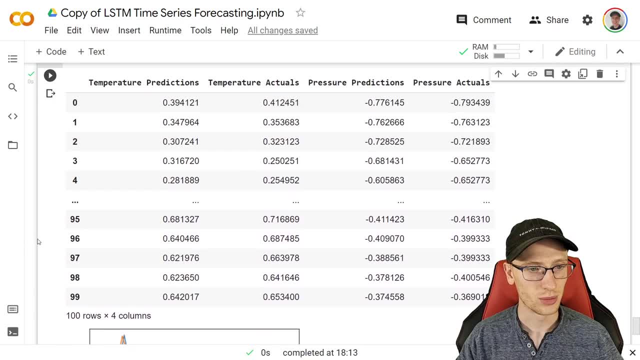 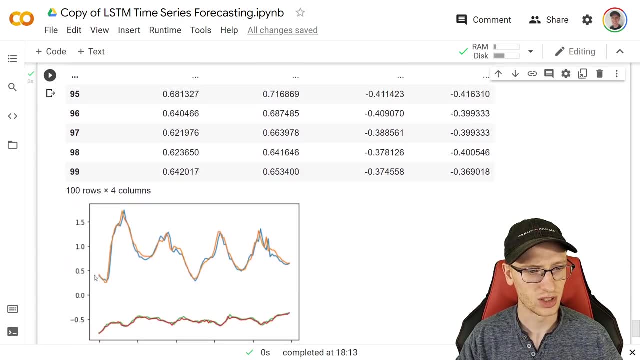 and the other one is forecasting this stuff And they're very close to each other. So to show the difference between temperature and pressure, temperature seems to go from 0.4 at the beginning and then 0.64.. So 0.4 and then 0.64.. 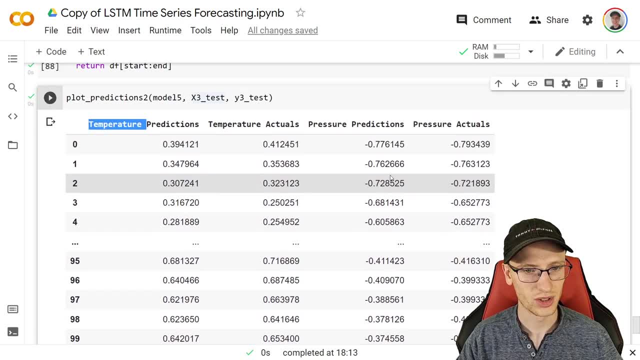 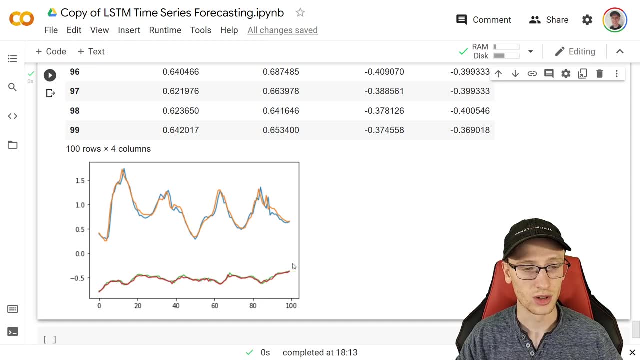 So this is the temperature stuff And our predictions are very close. And pressure they're from negative 0.76 to negative 0.37.. Negative 0.7 and negative 0.37.. They are, their predictions are very close as well. 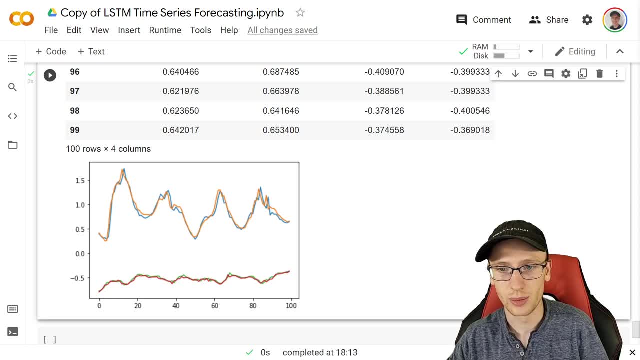 If you want to, if you want to edit this to make again change, get a better function for graphing it, then absolutely, by all means, go ahead and do that. Okay, so that is, that is our results. 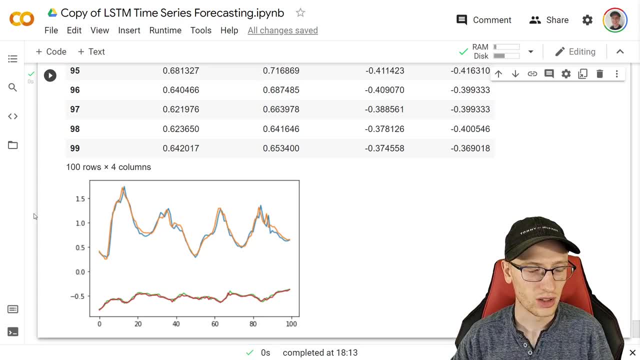 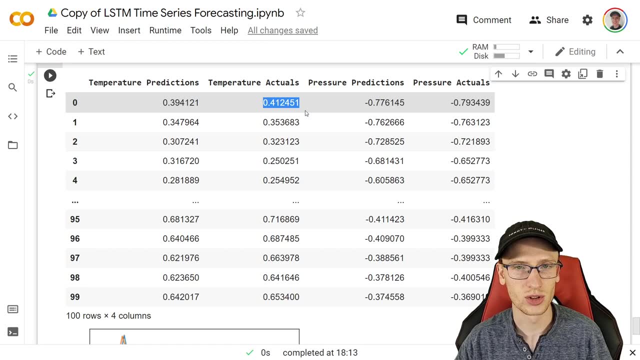 And they are very promising, But these are. these are not numbers that we actually care about, because we need to be able to undo this mapping. We can, of course, undo the mapping for the actuals, because we have the actuals, But for the predictions. you know, this is something where a model said: 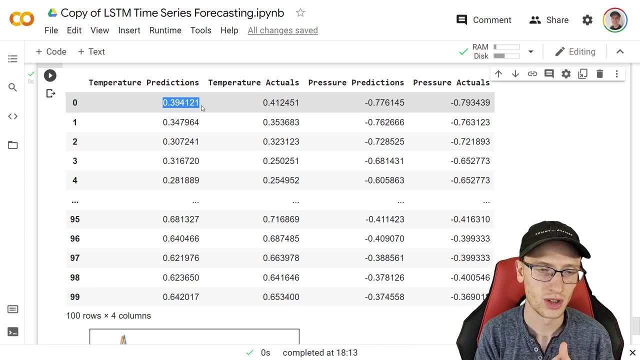 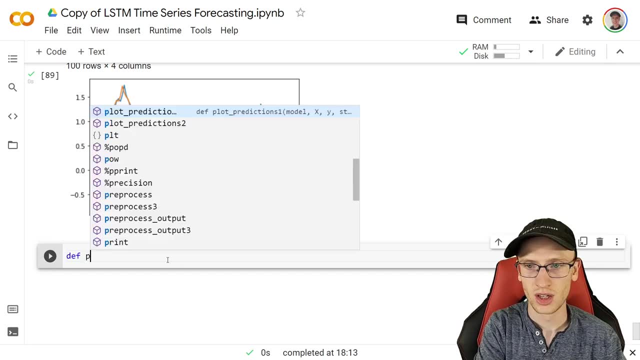 this is my guess, And we have to be able to complete, we have to be able to completely undo this with some, with some function mapping, And so we can do this by what's really called the inverse of, or the opposite of, what our pre-processing is. 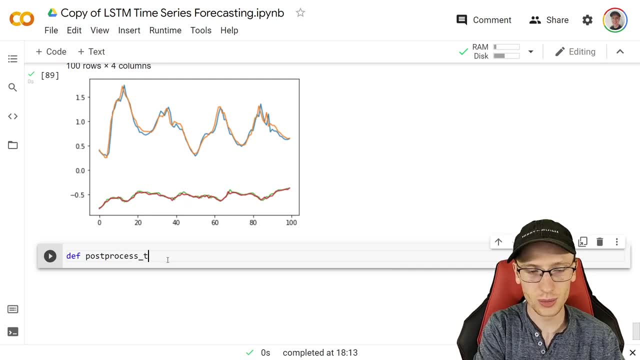 It's kind of interesting What we're going to call post-processing, post-process- this is just going to be for the temperature, And I'm just calling this an array because it's it takes in. really, you'll see how it works. 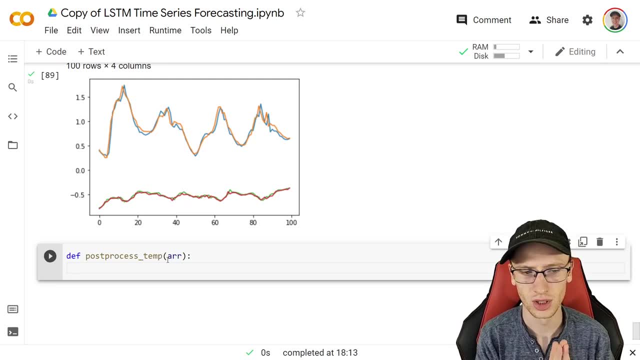 It doesn't really matter what the shape of this thing is, because it's just going to apply a function to that thing, regardless of what it is. But so what I mean to say is it's a scalar operation. It's going to do it to every single element in the array. 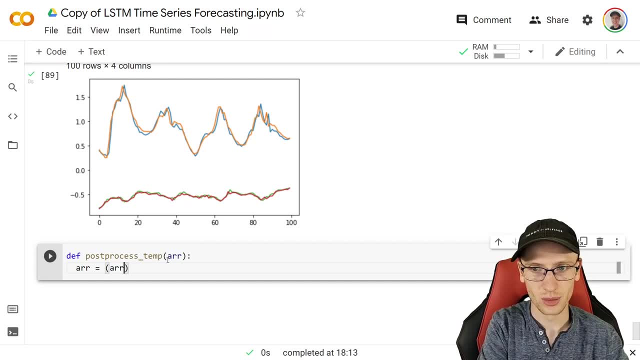 So I can just say array is equal to array times, and I'll explain this after temp training. temp training mean three And that, so we multiply that and then we add temp. Sorry, that's not that first one. That should be standard deviation. 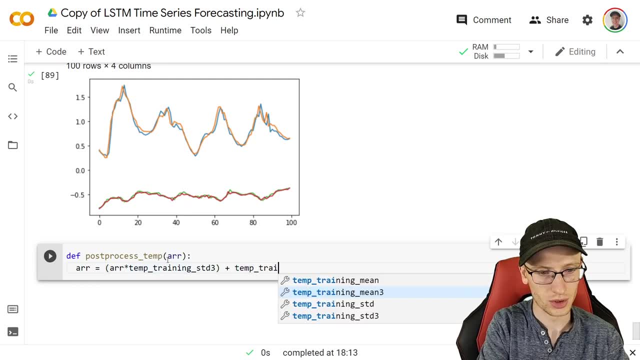 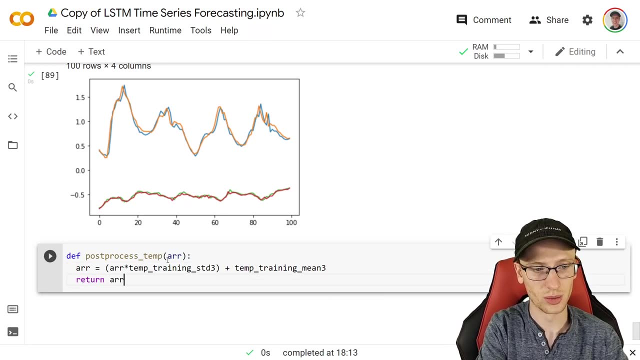 STD three plus temp temp training mean three. Okay, And then the reason for that and we'll return array. So note that this doesn't actually change this thing. This returns back a different one. So the reason before we had a divide: 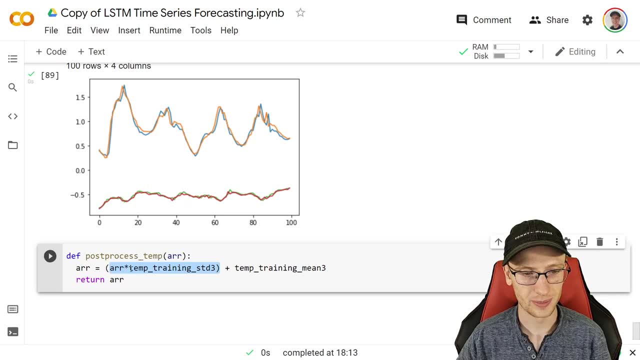 and so we changed that we do that first to do a multiplication And then after that we do an add. This happens to be the exact inverse of that standardization function. It gets back our prediction, And so I can write the exact same thing. 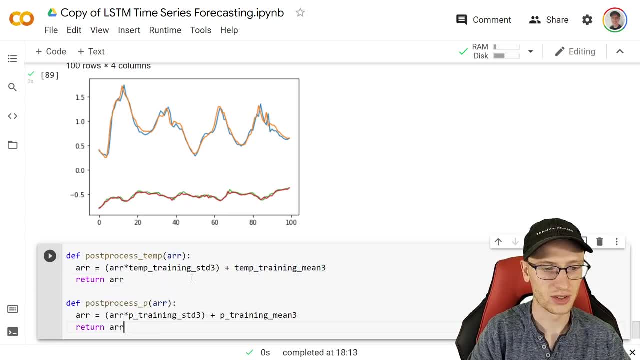 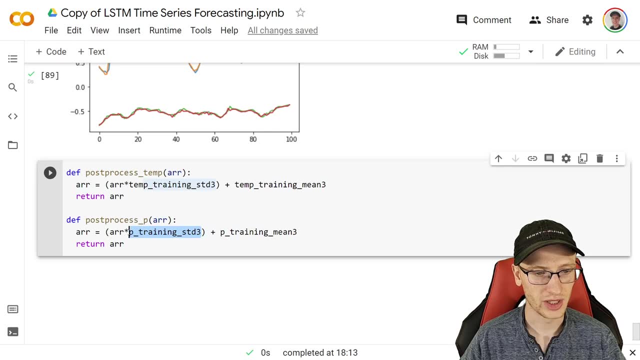 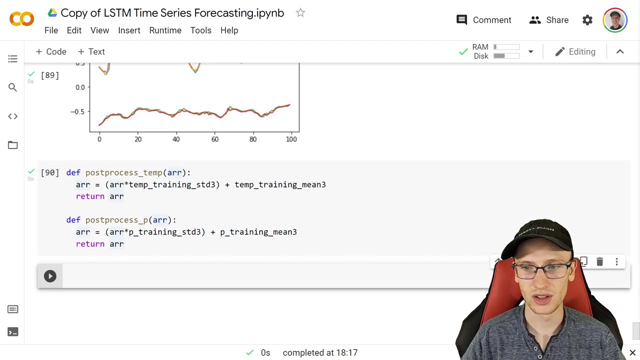 but for pressure, and that's just going to be like this: Post-processed P of R array is multiplied the array by that P training, standard deviation and that training mean as well. So we have those post-processed And then really this exact function. 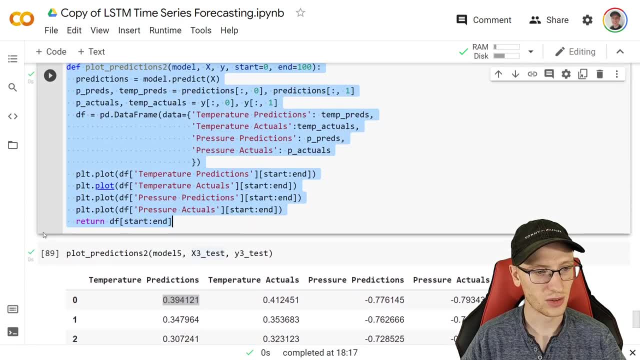 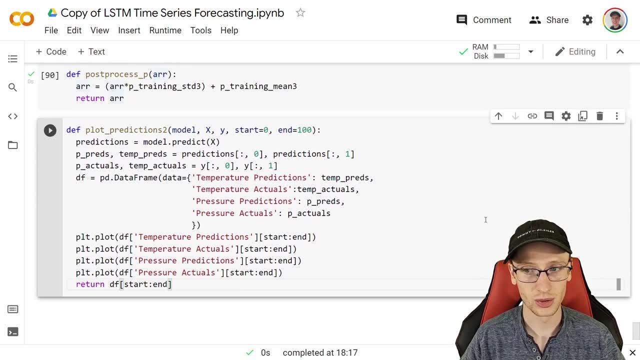 I'll just show you how it's made so we can follow this, This exact function we have before for plotting our results. but we can do the return the results, except with it post-processed. So we can put: um, we need to do this one. 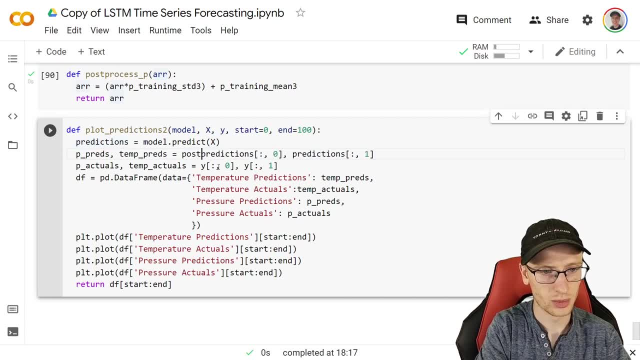 Um, this is for the pressure, So we can do this post-process. post-process. P: the, the pressure value there. We undo that. I'm going to copy that. I'll be writing that a lot. post-process. Uh, this is going to be temp like that. 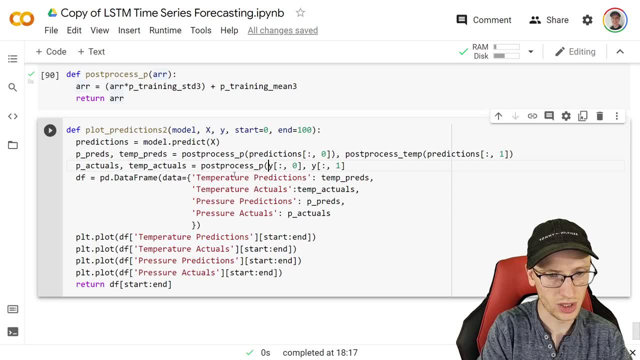 Okay, So we call that function there and post-process P of the first one there and then post-process P, So we're going to call it post-processed D. F is equal to P of the temperature as well. Sorry, that's not right. 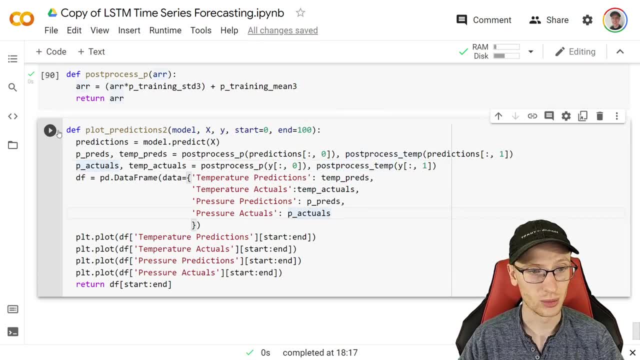 Um, temp, Okay. So that's like doing exactly the same thing, And I'm sure you don't have to write that much code. It's a better way to do this. but uh, that's just going to return it post-processed. 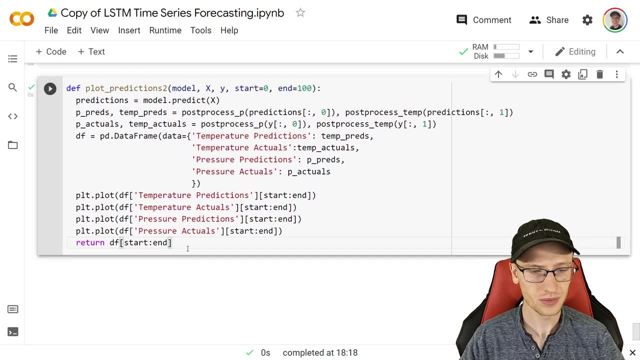 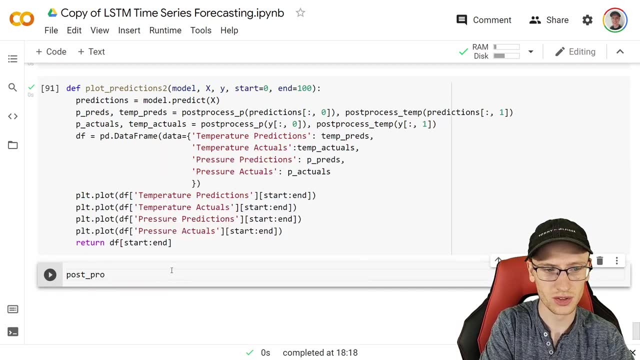 So that if we were to call it, um, and actually let me just uh, this returns the data frame And yeah, actually we might play around with this shortly, but let me, we'll call it like this: Post-processed. 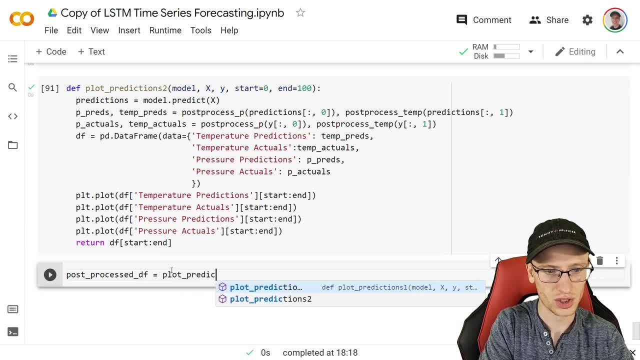 processed DF is equal to: uh, uh plot predictions. Oh, I remember why. Yeah, We're going to be switching this up- uh, plot predictions too. Um, and this is going to take in model five: X three, X three test and Y three test. 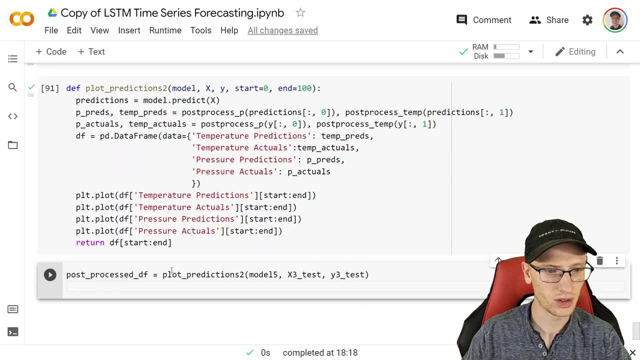 Okay, And then post um actually sorry. Yeah, it's fine If this returns the DF. so that's why I'm kind of just grabbing the DF Um. and there's a bigger reason for why this. I'm doing this shortly. 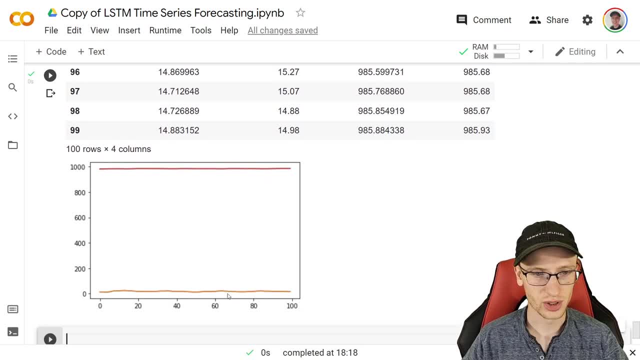 So this thing and it plots this- you can't even tell that there's four curves here. It looks like there's just two. uh, actually, maybe you can see it a tiny little bit that there's some blue down there. Um. 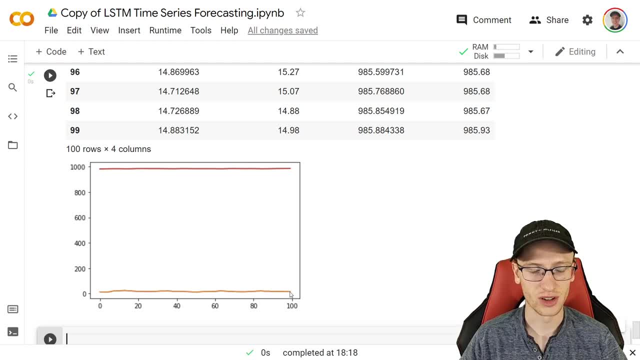 but yeah, so they're so close, And when we scale it like this to what they actually are, they end up to be so, so close to each other, And so because of this, we really can't graph them in the same plot. 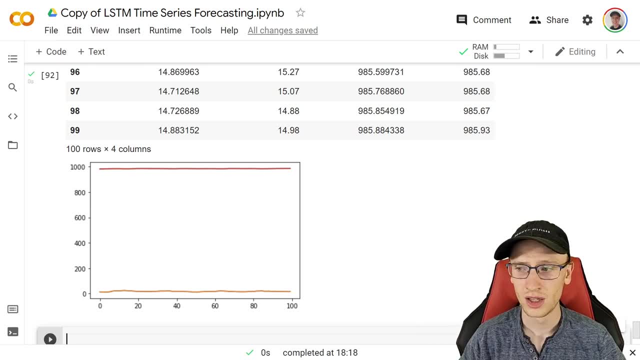 At least I don't know a nice pretty way to do that off by hand. Um, so we're going to just split them off, really, And I'm going to do this quickly for you because I don't think it's too relevant. 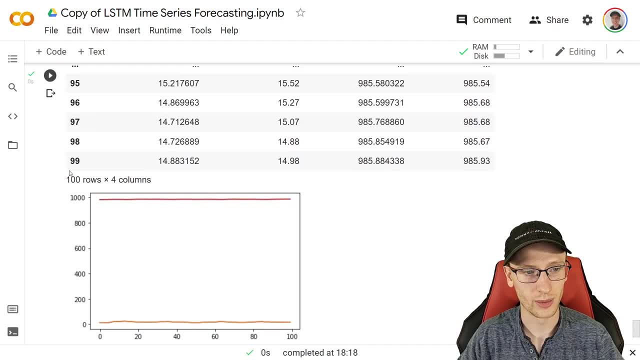 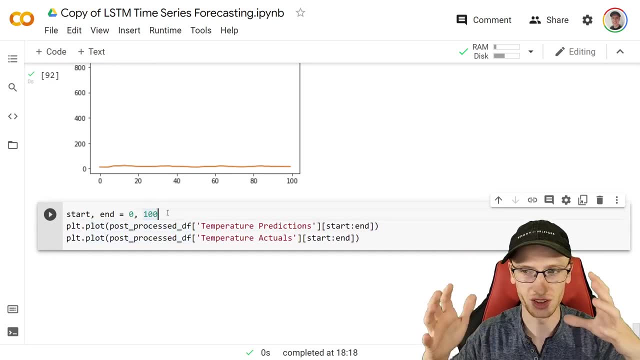 Basically, if we did, this is how we would do this. Since we grabbed post, processed DF, here I can do, uh say, start end equal to zero 100.. We need to take this out of the function because we're not doing it in the function anymore. 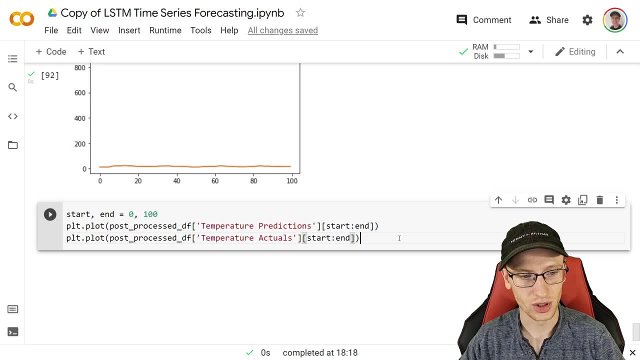 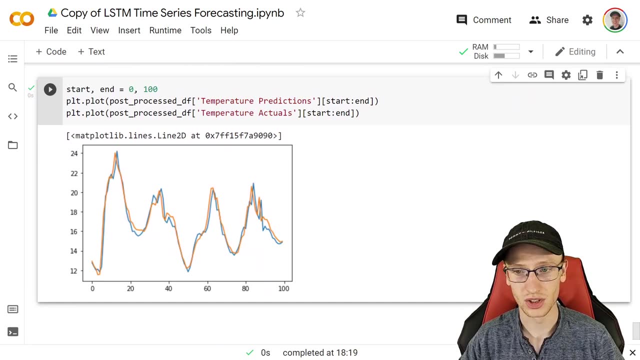 Uh, just with the DF temperature predictions and actuals from start to end, we could plot those And there is that. So that's just for pressure And we sorry, that's just for temperature And we can do this just for the pressure as well. 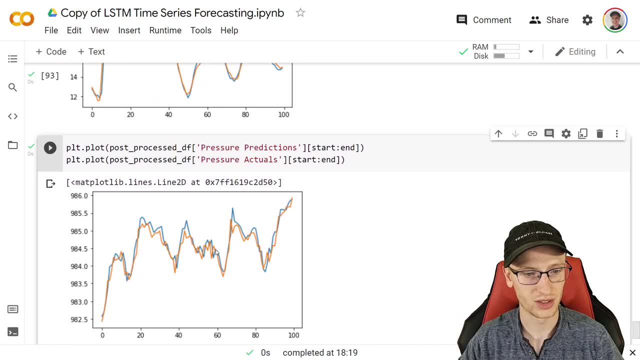 With, uh, plotting the pressure And it's nice how it is- It knows this really crazy jagged, jaggedy pattern, which is incredible. So that is mostly the end here, And it's really the end, if you want it to be. 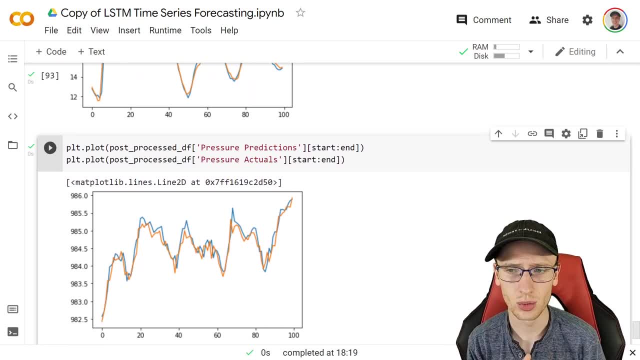 but I encourage you to stay for another, just a few minutes, where I'm going to show you some interesting things about time series and LSTMs. So, with the LSTM model, if we, if we take the exact same model as before, 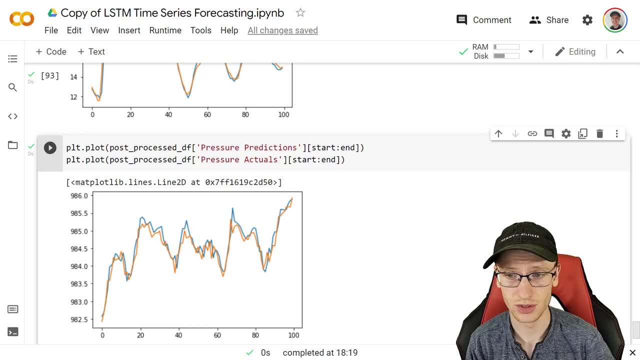 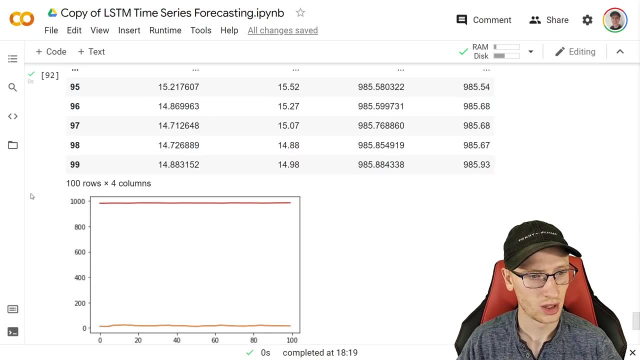 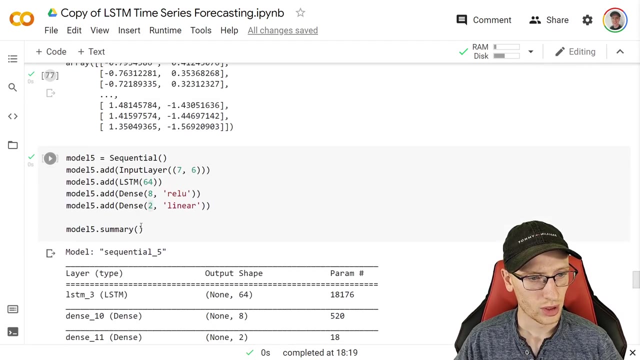 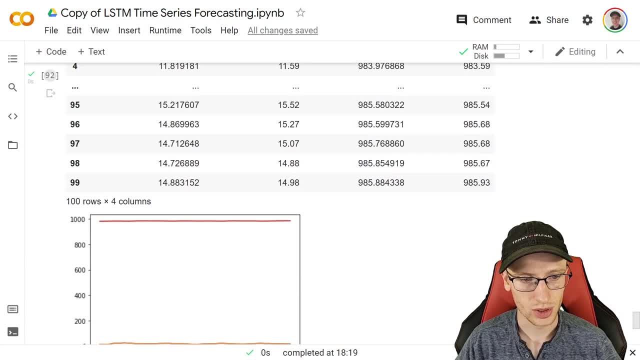 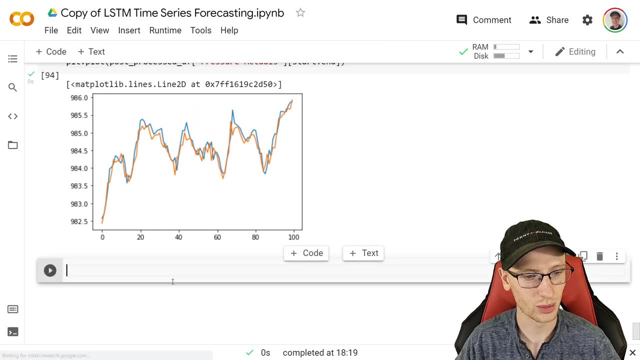 Uh, there's something interesting we can do to increase the complexity of the model if we wanted to, and you'll see if people do this a lot. why can I not? I never have these code blocks, I don't know why. Um. 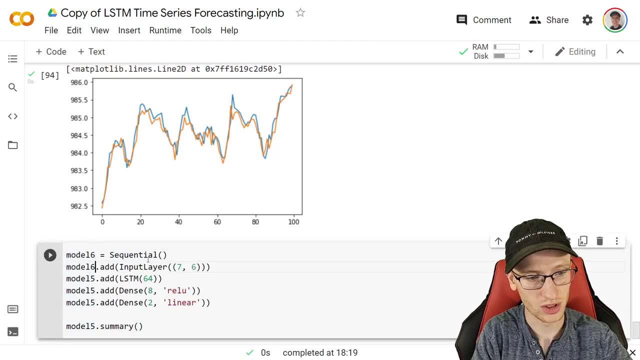 so here we have model five, but also quickly switch it to model six. I'm not actually going to fully train it, I'm just going to train it up until the point that shows you it works. Um, here we have LSTM 64.. 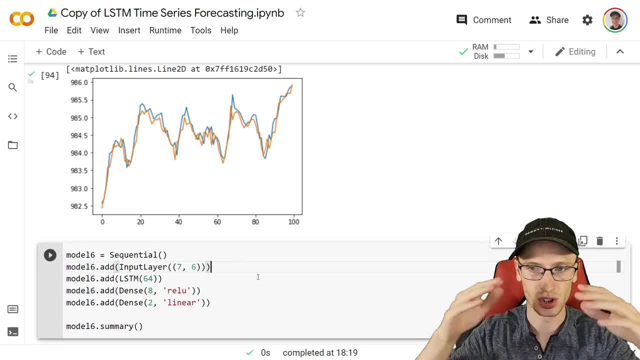 If you want it to actually uh, do this weird kind of chain. It makes this kind of like a square model. almost Basically. you pass things upward and then upward and then upward, rather than just kind of recurrent through this thing, And I know it's kind of hard to. 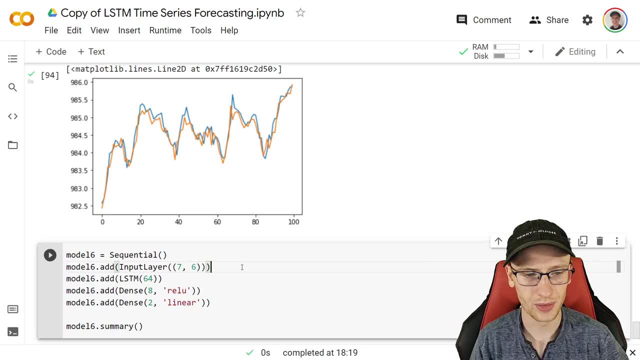 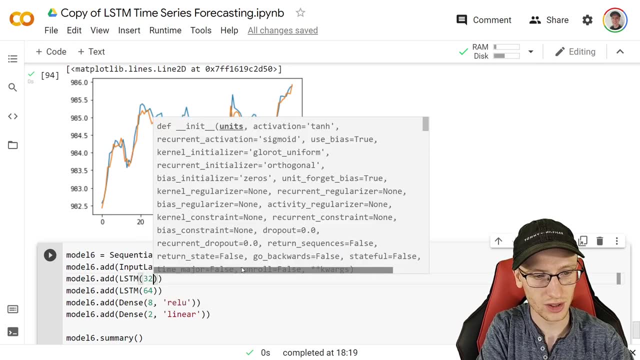 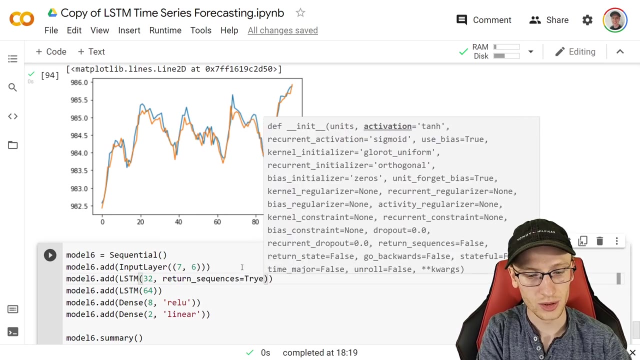 picture if you're not super knowledgeable about this stuff, But basically just to do it in code. we can do model6.add another LSTM And we can do this, say 32 of them. It actually didn't really matter the value too much. Return sequences equals true And this makes sense. 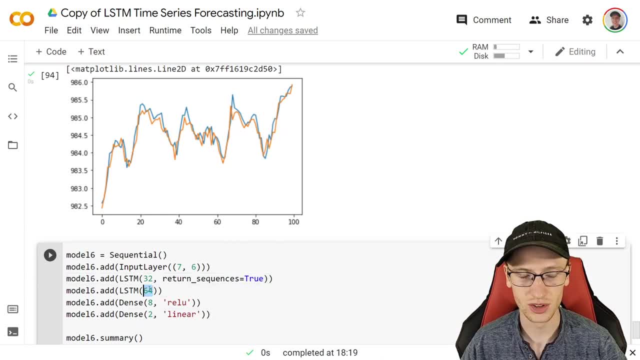 roughly, because you know that this LSTM it takes a sequence, It takes a time series And so if we feed it in, if it says, hey, return sequences and then feed it into this LSTM, that's basically passing this already processed and learnable LSTM here, passing that into this. 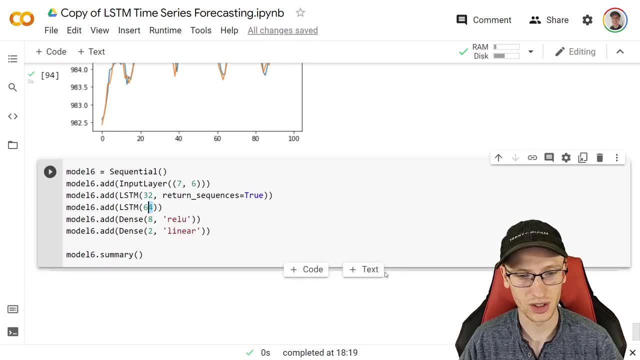 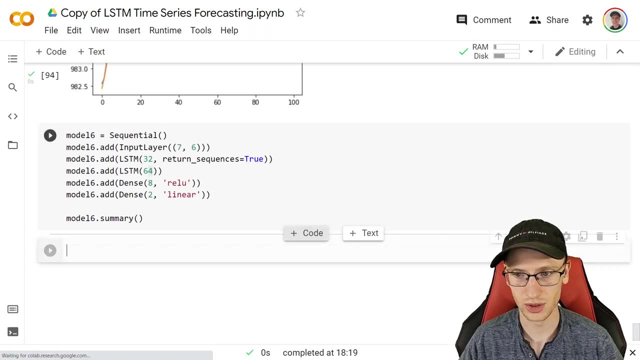 next one here, which is very interesting. That model would work. I'm not going to bother, Actually. sure, I will quickly just grab those. Actually, I'll grab it from my other notebook so that I don't have to bug you with this. 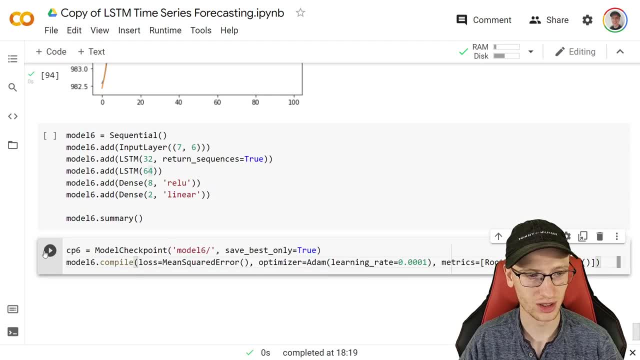 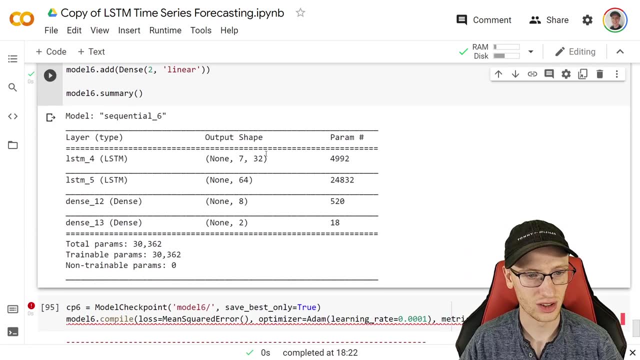 So here just model6.checkpoint would be exactly the same thing, And that's totally fine. And no, it's not. model6 is not defined. I didn't click that Now, it's fine. Yes, there's the model. So 7 by 32 now. 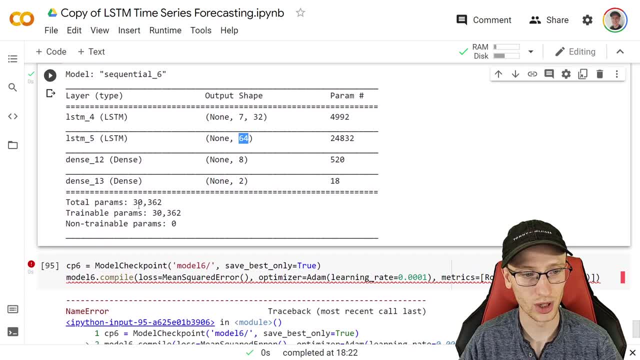 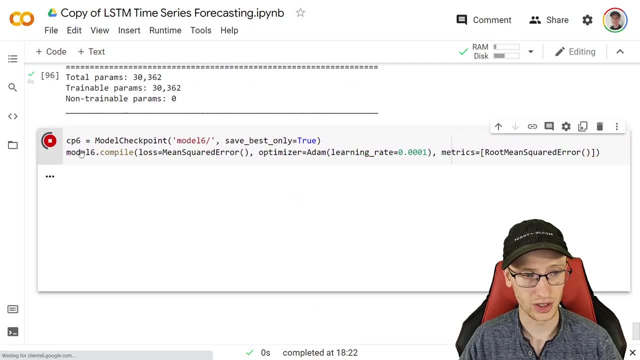 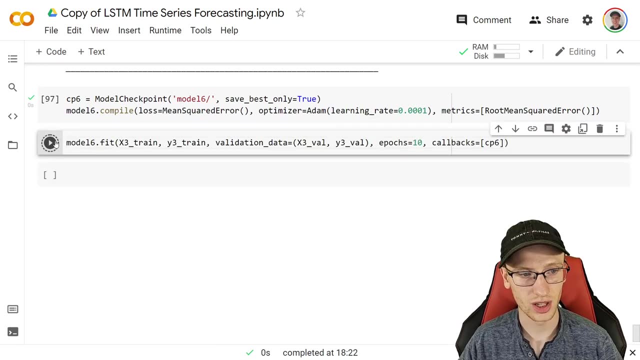 and 64.. Okay, very interesting. More parameters, for sure, A lot more parameters. It's a heavy model. 30,000 is definitely approaching a big model. model6 is defined now. There you go, There it is. We're going to fit that just to the point, to show you that it's going to work. 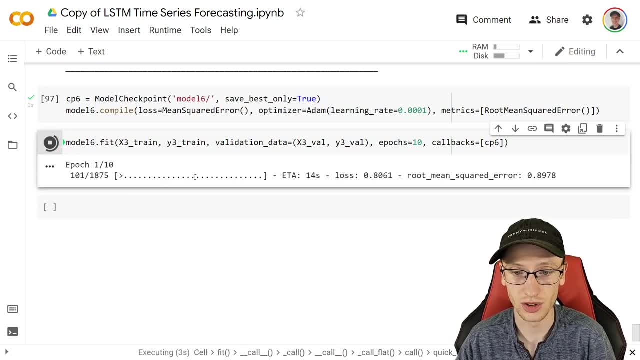 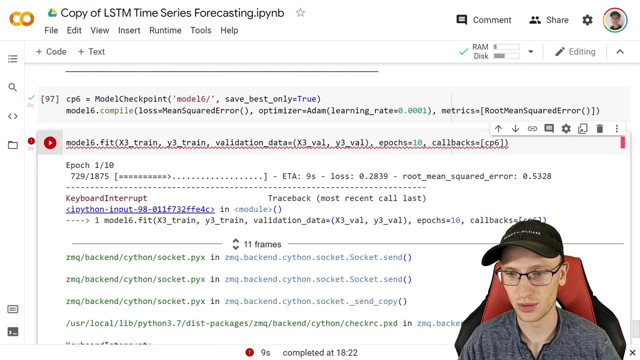 I don't really care about the accuracy, but I'm telling you it's probably going to be pretty darn high. It might overfit a little bit, That's quite possible- but it's going to work And I'm not going to let you see that. Absolutely go for it. If you want to check out my notebook, it is in the 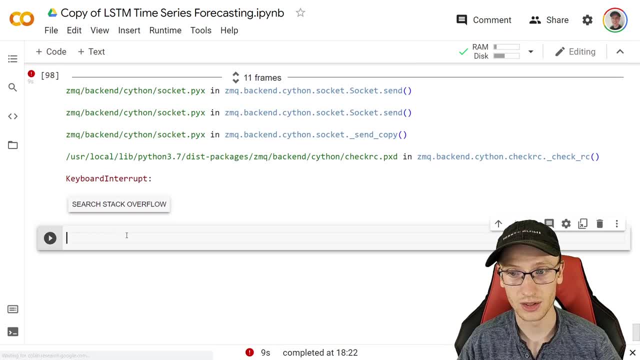 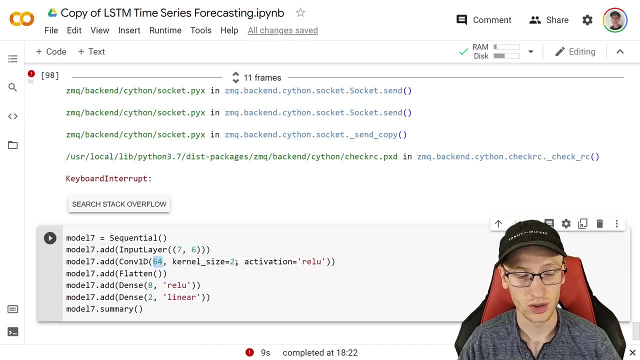 description, like always- And model7 is something else which I'm just going to paste here for you- is: takes in 7 by 6 and then conv1d64, kernel size of 2.. Let me show you something. Okay, if we go. 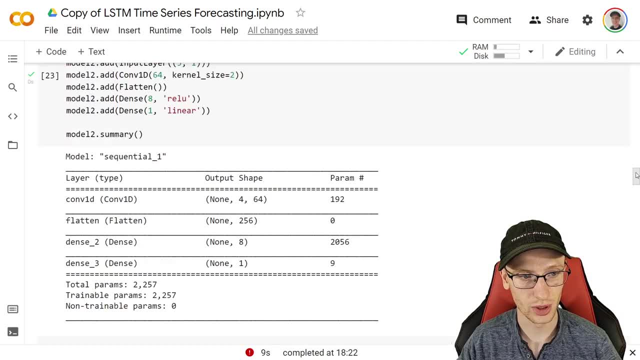 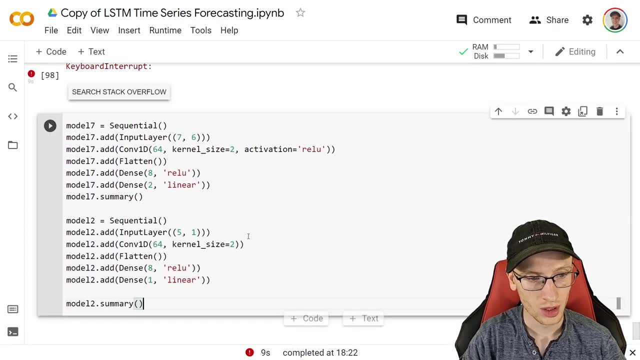 back up to- Sorry, all the way up into our other convolutional model. Convolutional model is here. Let me paste them side by side to show you the difference. Remember that why we were doing this is because the window was 5 and we were just using one variable. Well, here we just specify the input. 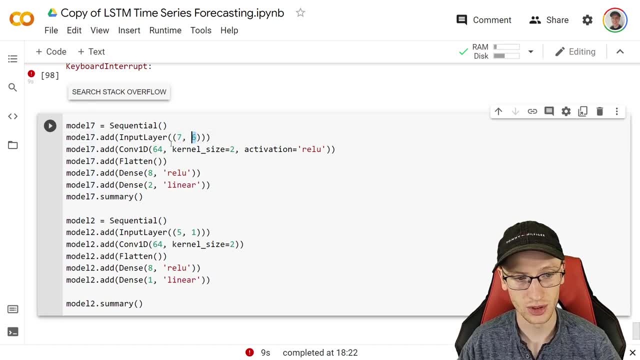 You always got to do that anyway. The window is going to be 7 now, with 6 variables and then conv64.. I guess I should also do an activation equals ReLU there. I don't know why I didn't have that earlier. 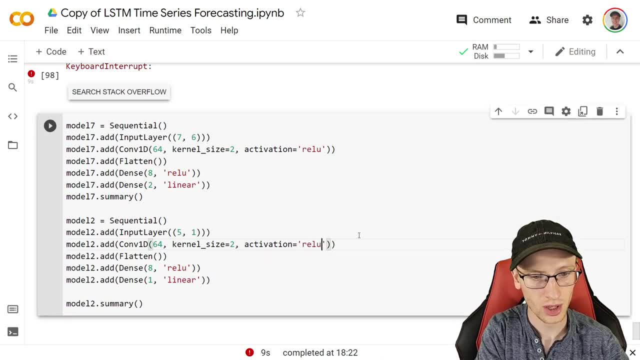 Okay, Activation equals ReLU is pretty common And yeah, so it is exactly the same thing, like exactly the same. You just specify that the input is going to look a little bit different, but it doesn't change the convolution part. This works totally fine And what it does is kind of traces. 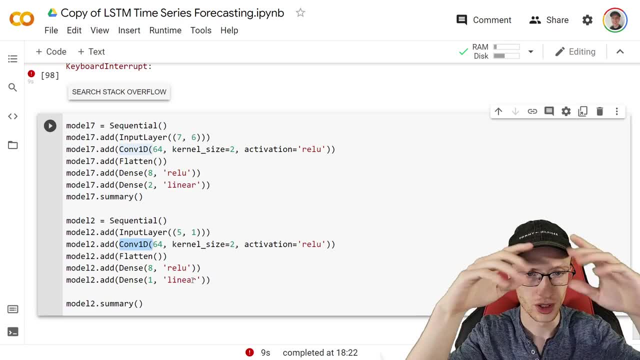 this like because we have. you can picture, basically it works on this matrix of input And so we're going to be sliding, or each row is going to be a particular line, Variable pretty much. It's a little bit tough to picture that way, So actually I wouldn't worry. 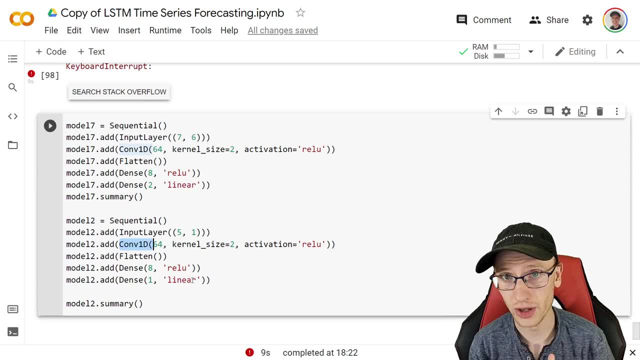 about it too much. Basically, you're sliding this window across multiple variables now, And this works as well, And that could be a lot lighter model And, as we'll see, I'll just let it do that Also. we also changed the output, but that didn't have to, So here it's still only.